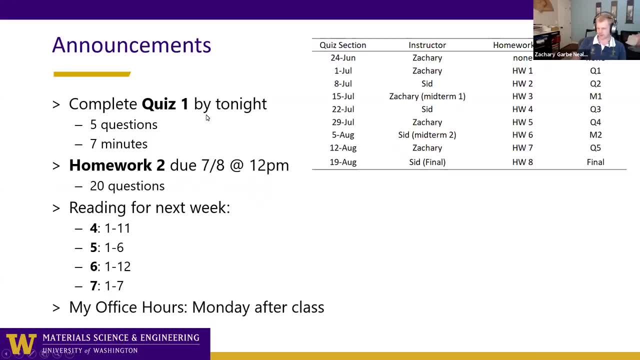 And this is what the quizzes will be like for the remaining quizzes as well, And it's only available today. So you have until midnight tonight to start and complete this quiz in seven minutes. Homework two: I'll post that today. It'll be due next Wednesday at noon. It has 20 questions. I think I might- actually I still have to edit one of the questions, but that'll be available this afternoon, this evening. 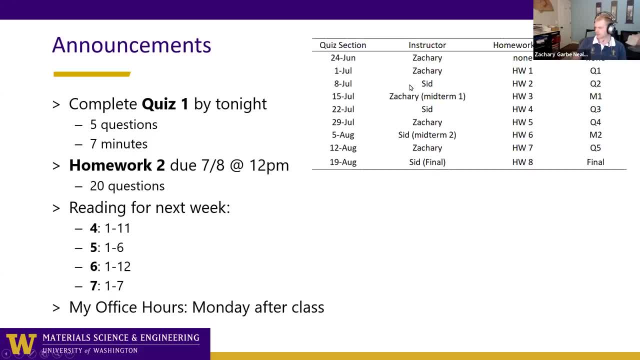 Next week we have a new TA in charge of quiz section- That will be Sid, And homework two is due next week And again there will be another quiz on the same day in a similar format, And then the week after that is your first midterm. So I will not be doing a quiz section, but during quiz section- I believe this is the case- you'll be taking your midterm. 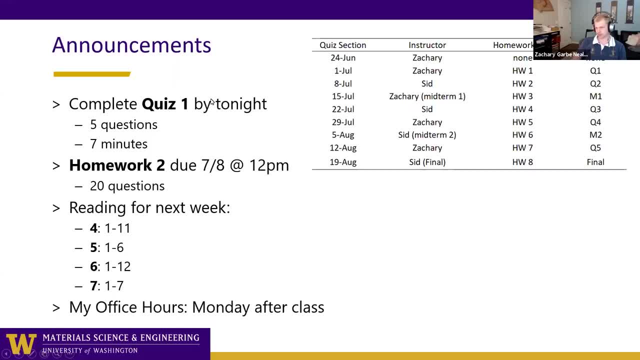 And we still don't know the format. It's either going to be on Canvas or through. I mean, it's definitely gonna be on Canvas, but it might be similar to the quiz, where you have like an hour to complete it and whatnot. 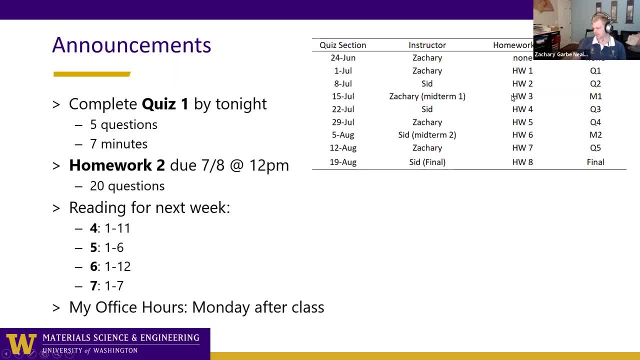 You also have homework due that that that day as well. Okay, And then make sure you're on top of the reading. Like I said, the summer quarter things are going by a bit quickly, So you know, read ahead for next week. This is this is the reading assignments for next week. 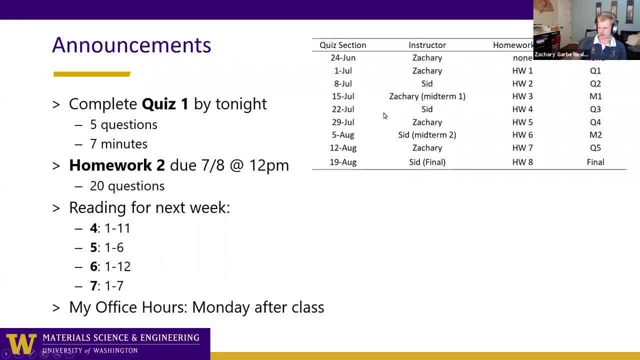 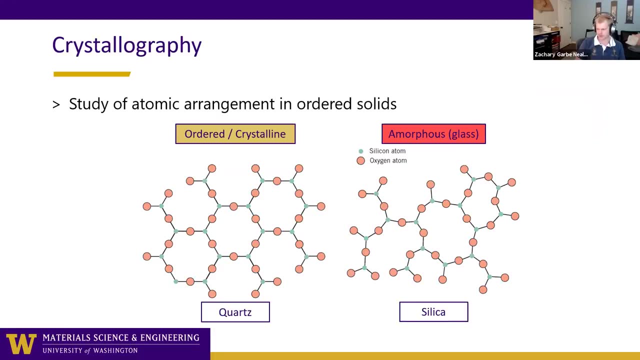 Also, I've established my office hours on Monday after class. on Monday, Every now and then I might offer some additional office hours and I'll send an announcement out, Okay? So Dr Brush today talked about crystals and I wanted to talk more about that, Crystallography, of course, the study of the atomic arrangement and solids. So you have a. 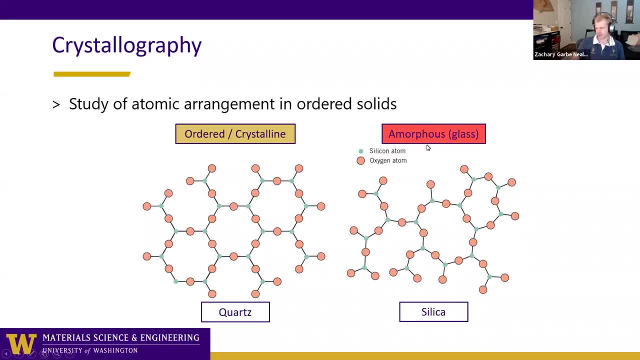 crystalline solid, where it has long range order, and then opposed to an amorphous solids known as a glass material, where it still has short range order. right, so you have silicon. Silicon is still tetrahedrally coordinated to oxygen, but there's no long range order in an amorphous solid. 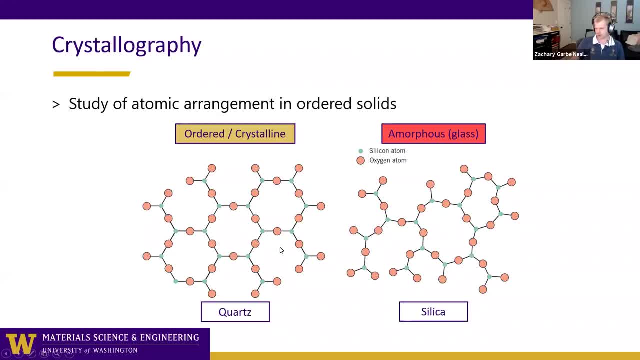 Alright, so this is an example of quartz versus silica And quartz and silica. they have the same chemistry, the same components- silicon and oxygen- but one is crystalline, one is amorphous And, of course, as you know, silica makes up most. glass is a major component of like window glass and other glasses. 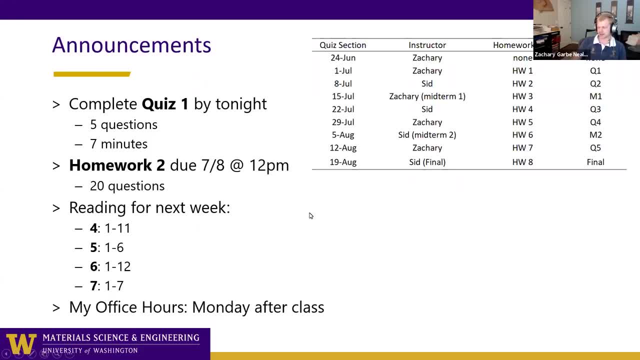 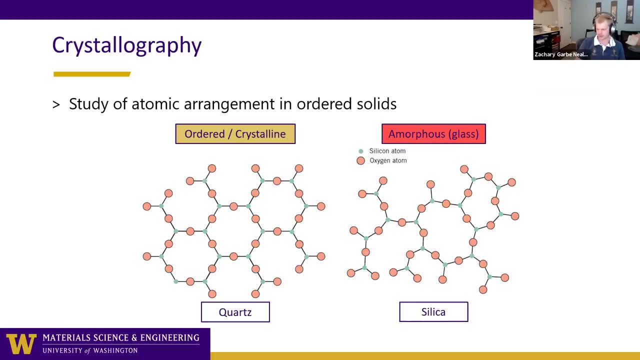 Also, I've established my office hours on Monday after class on Monday. Every now and then I might offer some additional office hours and I'll send an announcement out, Okay? So Dr Brush today talked about crystals And I wanted to talk more about that: Crystallography, of course, the study of the atomic arrangement and solids. So you have a crystalline solid where it has long range order. 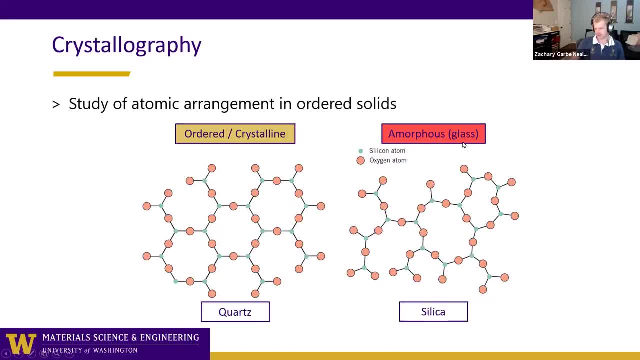 And then opposed to an amorphous solids, known as a glass material, where it still has short range order. right, So you have silicon. Silicon is still tetrahedrally coordinated to oxygen, but there's no long range order in an amorphous solid. 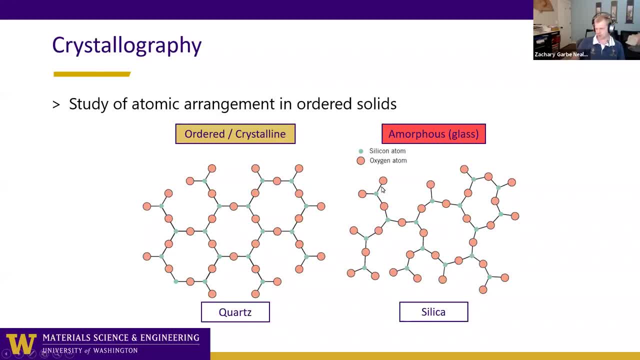 All right. So this is an example of quartz versus silica And quartz and silica. they have the same chemistry, the same components- silicon and oxygen- but one is crystalline, one is amorphous And, of course, as you know, silica makes up most. glass is a major component of like window glass and other glasses. 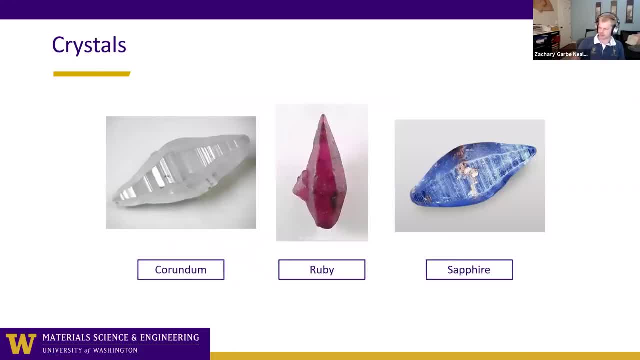 Like drinking glasses. So here's another example of crystals. These three crystals look very similar, right? They have the same sort of shape to them and Although they're different colors. So this is corundum, ruby and sapphire. And does anyone know the atomic- excuse me, the chemical formula for these three crystals? 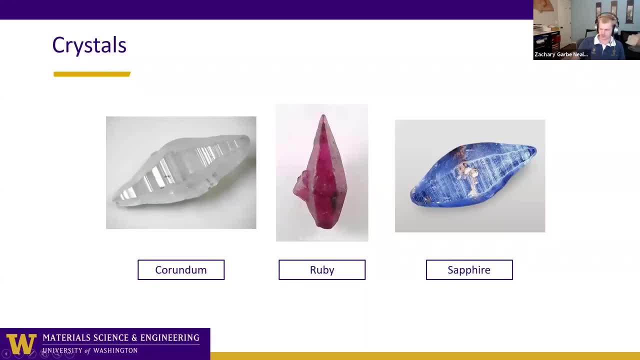 Or one of these three crystals. Okay, The chemical formula for corundum, ruby and sapphire is Aluminum oxide, Aluminum oxide, For all three of these are made out of the same base material, which is aluminum oxide, a crystalline aluminum oxide. Now for ruby and sapphire is interesting To make the color. it gets doped doping. It means we're adding some kind of impurity to the crystal. In this case, for ruby, we're adding about 1-3% by weight. 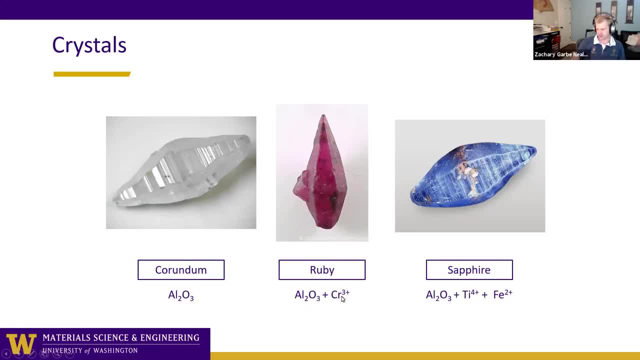 I think it's weight, not atomic percent. Chromium 3+: The crystalline material in blue here is actually lithium tri piano, Immerflux, And we're substituting it with aluminum inside the crystal structure. So the crystal structure is still the same, just some of the atoms have been replaced with chromium, And that makes the crystal read. 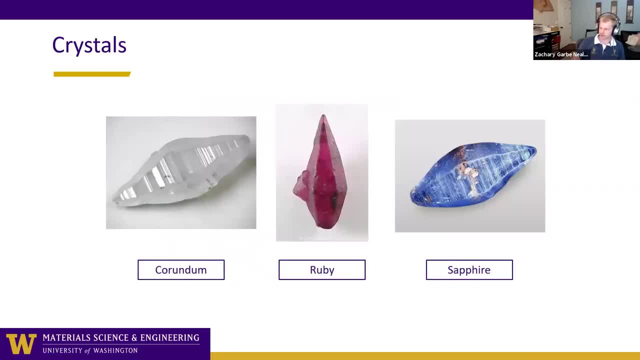 Like drinking glasses. So here's another example of crystals. These three crystals look very similar, right? they have the same sort of shape to them And although they're different colors. So this is corundum, ruby and sapphire. And does anyone know the atomic- excuse me, the chemical formula for these three crystals? 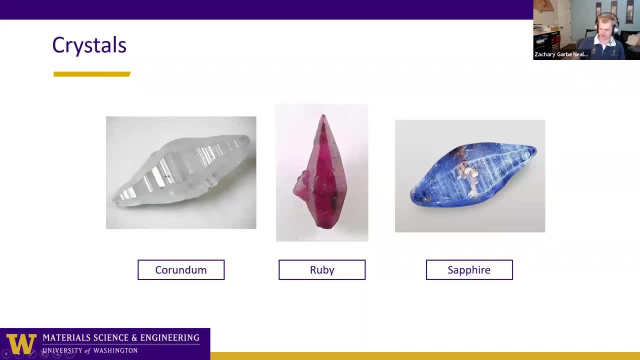 Or one of these three crystals. Okay, The chemical formula for corundum, ruby and sapphire is aluminum oxide- Aluminum oxide, For all three of these are made out of the same base material, which is aluminum oxide, a crystalline aluminum oxide. Now for ruby and sapphire, it's interesting to make the color. it gets doped doping, which means we're adding some kind of impurity to the crystal. 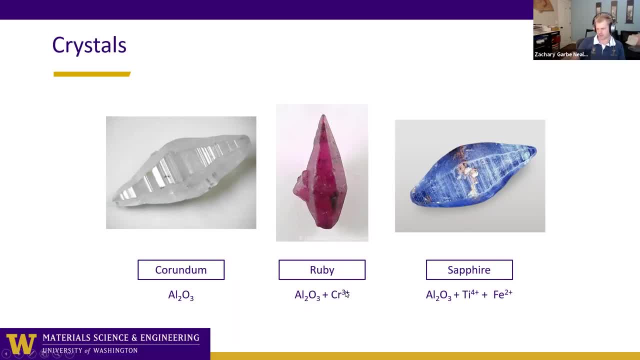 In this case for ruby. we're adding about one to 3% by weight- I think it's weight, not atomic percent- Chromium 3+, and we're substituting it with aluminum inside the crystal structure. So the crystal structures is still the same, just some of the atoms have been replaced with chromium and that makes the crystal red. 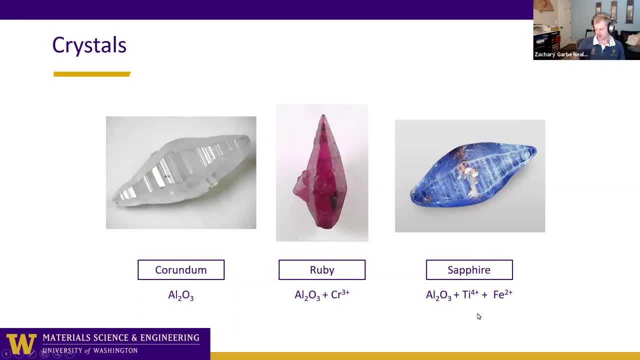 And sapphire. you do the same thing with titanium and iron: you have to have both in order to make it blue color. So that's a little bit of interesting. But the point is that they have the same crystal structure and that's what gives it this macroscopic shape. 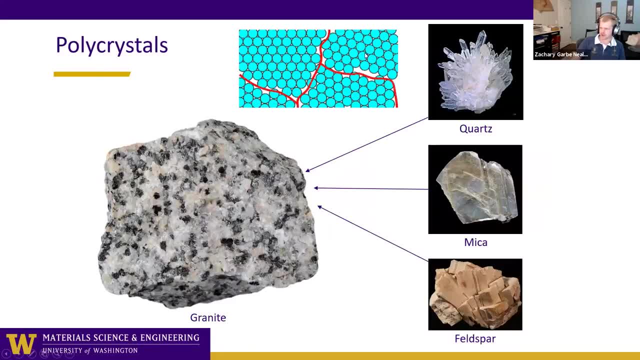 And, as Dr Brush mentioned, there's polycrystals, polycrystalline and polycrystalline. Polycrystalline materials have many smaller crystals and the boundaries of these crystals are called grain boundaries. So each one of these- 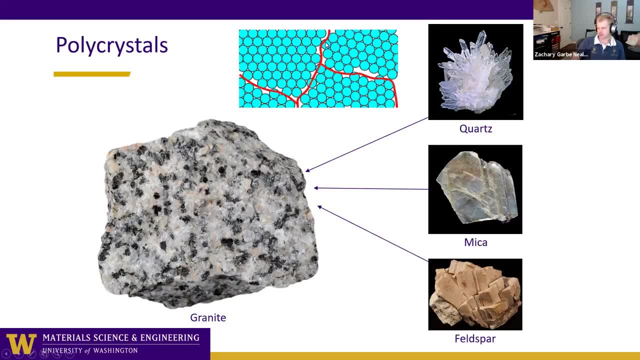 crystallites has its atomic arrangement, its crystal structure, but they might be in different orientations next to each other. Here's an example of a polycrystalline material. Not only is it polycrystalline, but it's a. 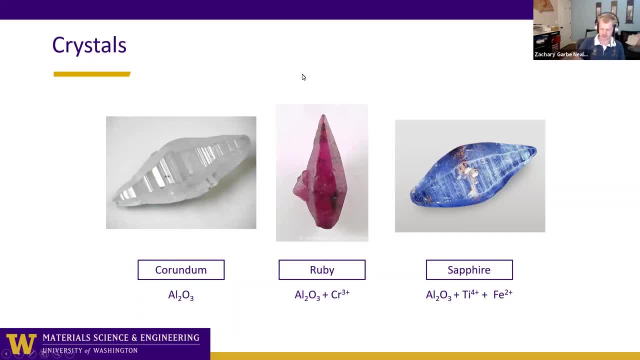 And sapphire, or the same thing with titanium and iron: you have to have both in order to make it blue. So that's a little bit of interesting, And but the point is that they have the same crystal structure and that's what gives it this macroscopic shape. 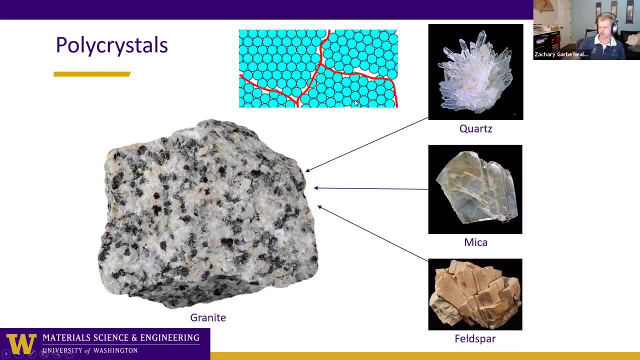 And as Dr And as Dr Dr material have many smaller crystals and the boundaries of these crystals are called grain boundaries. all right, so each one of these uh crystallites has its atomic arrangement, this crystal structure, but they might be in different orientations next to each other. here's an example. 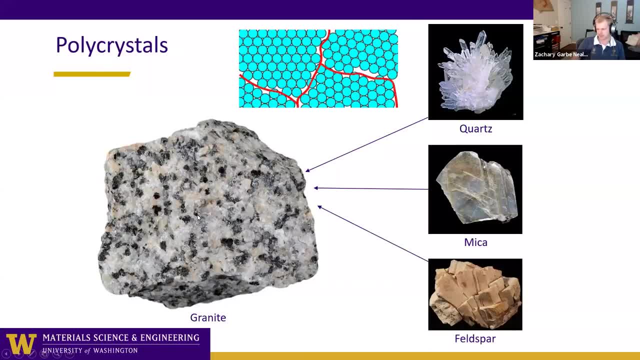 of a polycrystalline material. not only is it polycrystalline, but it's a polycomposite material. it's a- you could consider it a composite right? it has multiple minerals, multiple different, uh chemical formula, uh, excuse me, chemical compounds that make up this granite. so quartz. 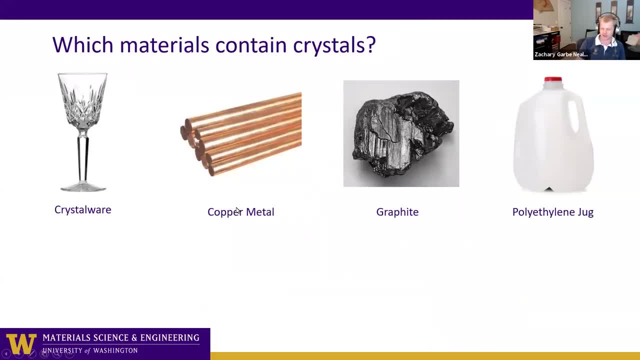 mica feldspar. uh, here's a a little quiz. i i like to give this to um. i do a lot of outreach for k through 12, so i don't give you guys the same kind of quiz. uh, you know which one of these materials? 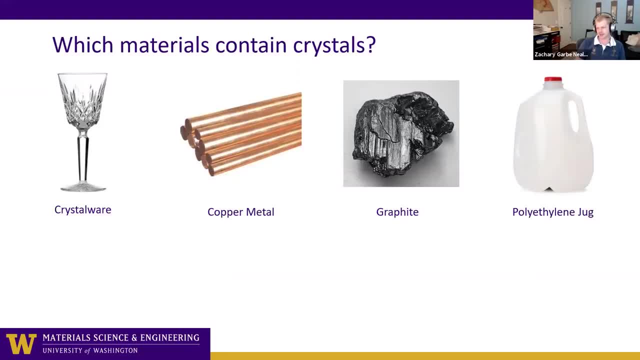 contains crystals. and uh, there's, there's one of these materials that does not contain crystals. so in the in the chat, where you can shout it out, which one of these do you think does not contain crystals? we have crystalware: copper, metal, graphite, polyethylene. all right, it looks like most of you guys are saying, uh, the polyethylene jug. 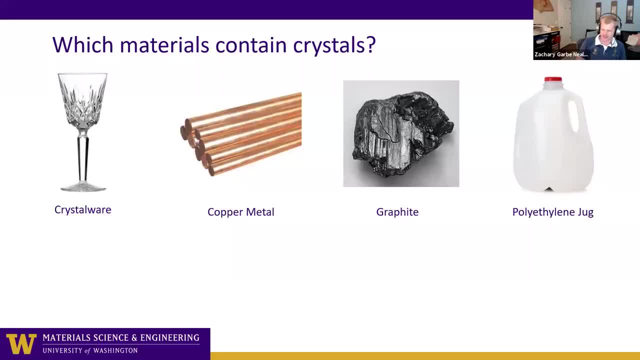 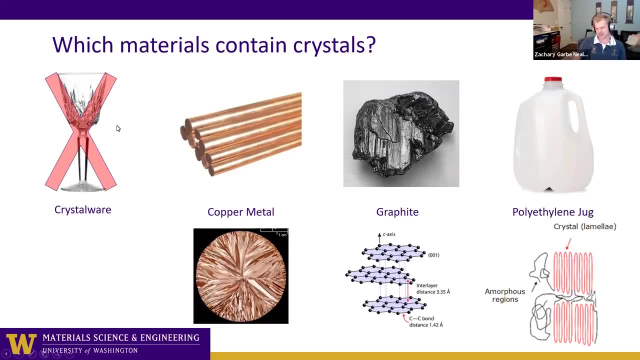 does not contain crystals and that is incorrect. yeah, it's a kind of- yeah, it's a trick question: the crystalware material on this uh list that does not contain crystals, crystalware, is actually glass. all right, it's just called crystalware because you know it has facets, it's cut and it looks like crystals. 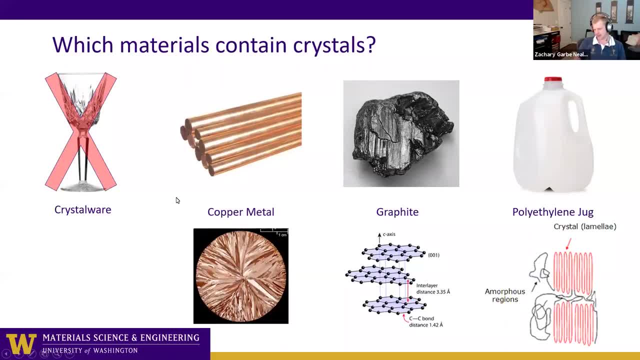 where you know- uh, this is something i learned. i didn't know until like high school i took a material science camp here at the uw- that metals contain crystals and that kind of blew my mind that metals, and everything almost, is made up of crystals. graphite, of course, has a crystal structure. 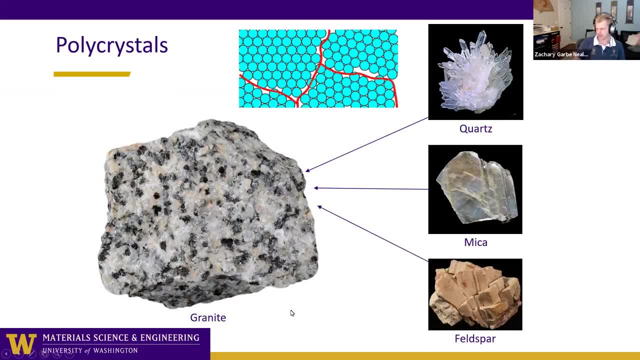 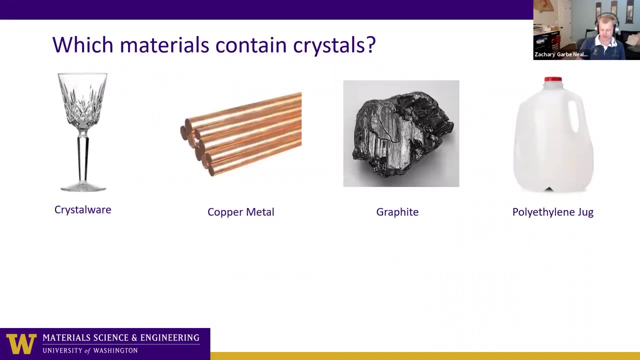 polycomposite material. You could consider it a composite. It has multiple minerals, multiple different chemical formulae, excuse me, chemical compounds that make up this granite. So quartz, mica, feldspar. Here's a little quiz I like to give this to. I do a lot of outreach for K through 12, so I'm giving you guys the same kind of quiz. You know which one of these materials contains crystals and 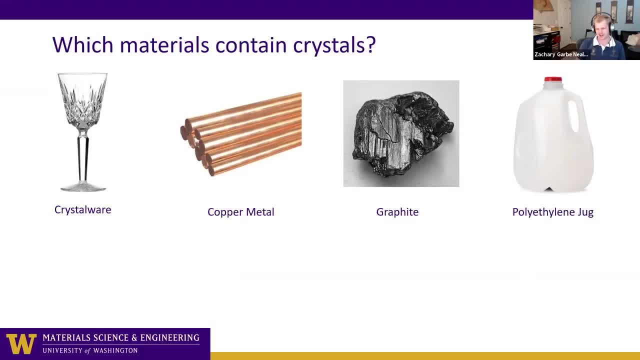 there's one of these materials that does not contain crystals. So in the chat where you can shout it out, which one of these materials contains crystals? here's the question: Which one of these do you think does not contain crystals? We have crystal ware: copper, metal, graphite, polyethylene. 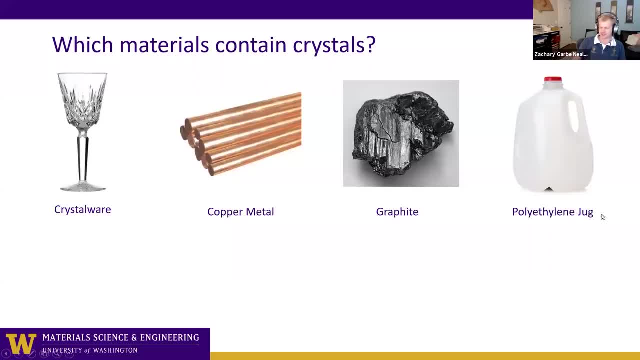 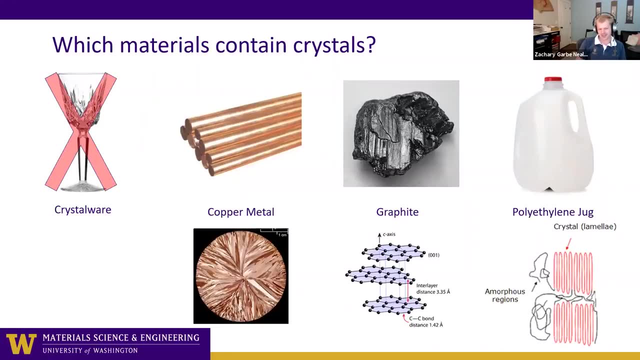 All right, Looks like most of you guys are saying the polyethylene jug does not contain crystals and that is incorrect. Yeah, it's a kind of a trick question. The crystal ware is the only material on this list that does not contain crystals. Crystalware is actually glass. all right, It's just called. 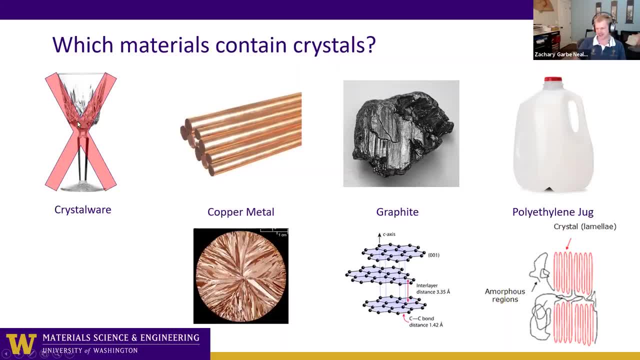 crystalware because you know it has facets, it's cut and it looks like crystals where you know. this is something I learned. I didn't know until like high school I took a material science camp here at the UW- that metals contain crystals and that kind of blew my mind that metals and 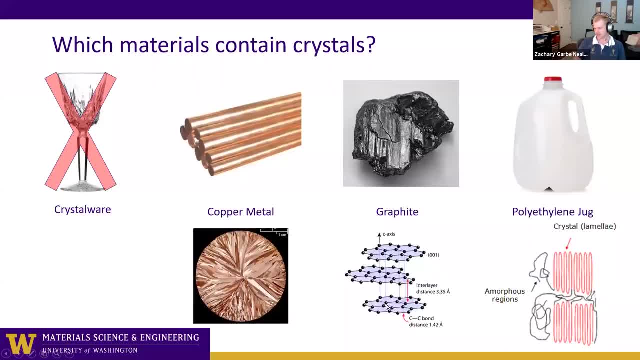 everything almost is made up of crystals. Graphite, of course, has a crystal structure. We talked about that on the first week. The polymer- and this is what most people say- is that it doesn't have containing crystals. Polymers do will be kind of semi-crystalline, where their polymer chains will. 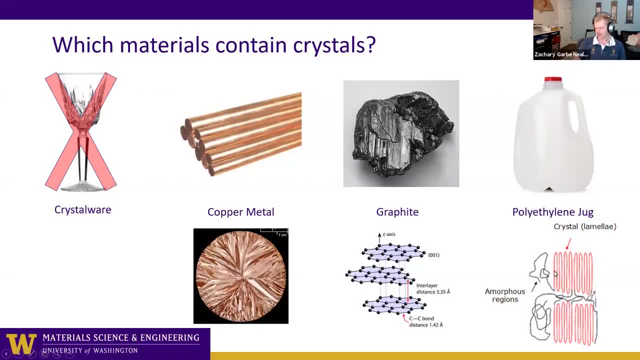 arrange in a periodic fashion with long-range order and so that the polymers do contain crystals, a crystal structure. Crystalware is a specific type of glass. Does anyone know what crystalware is? No, the K through 12 students also all said the polymer. Some of them say the copper metal too. so 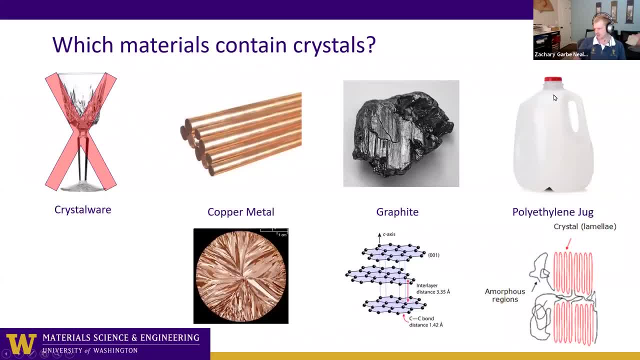 the polymer- and this is what most people say- is that it doesn't have containing crystals. polymers do will, uh, be kind of semi-crystalline, where their polymer chains will arrange in a periodic fashion with long-range order, and so that it, the polymers, do contain crystals. 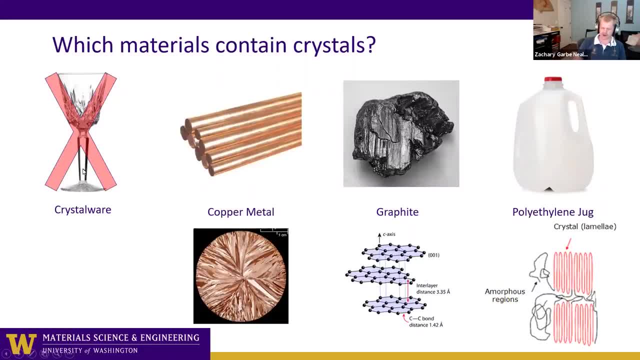 a crystal structure. crystalware is a specific type of glass. does anyone know? no, the k-12 student also all said the polymer. some of them say the copper metal too. so it's all right, the crystalware. does anyone know what uh type of glass crystalware is? 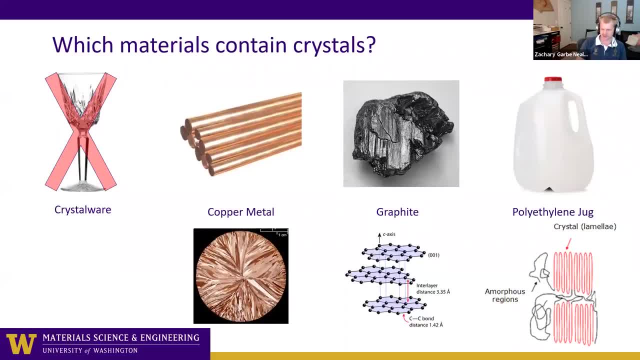 or what the chem? what the major? uh, what? what's the chemical formula that makes crystalware unique and doesn't look like anyone knows? so, crystalware, boron silicate, uh, nope, not quite, uh, nah, but it's not a borosilicate glass like pyrex is a borosilicate glass, crystalware is a lead glass. 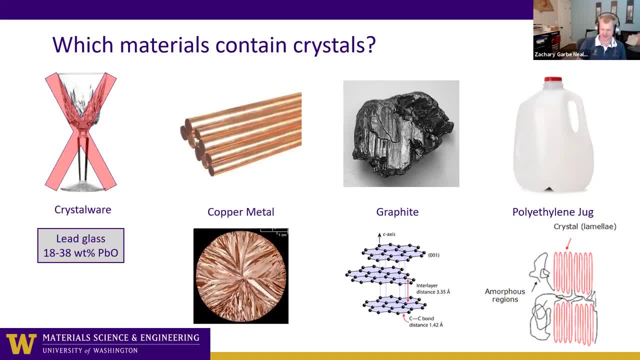 so you know, if you have any fine crystal in your house, it contains a bit of lead oxide. and the reason why? does anyone know why? well, i guess you might not know because you didn't know. the first question, the reason why crystalware uses lead oxide- is that the lead oxide component in glass. adding lead oxide to this glass increases. 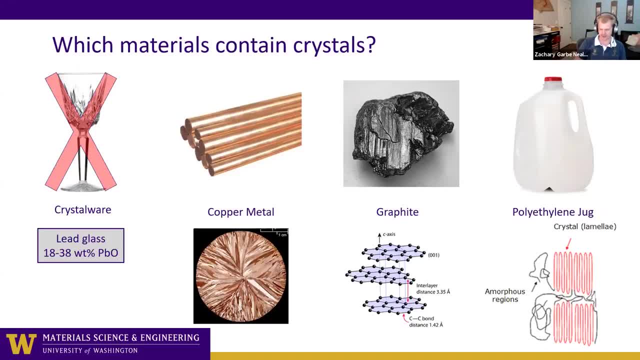 the index of refraction, all right. the refractive index, so it makes it. so the light that bounces in bounces out at a higher angle and so it makes it optically attractive. right like diamond has a very high index of refraction. cubic zirconia has a very high index of refraction. that's why we use it as a 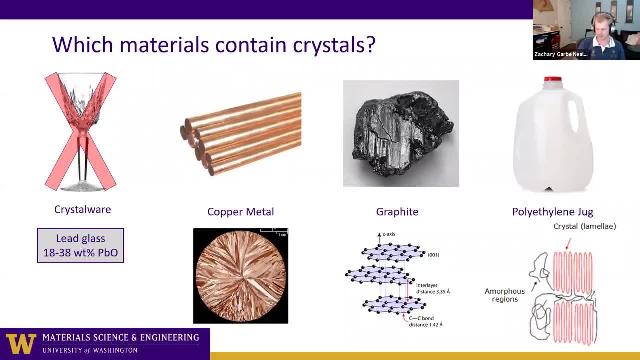 substitute for diamond and jewelry crystal. lead glass also has a fairly high index of refraction. the other reason why lead glass is used for crystalware is that it makes it easy to machine. it makes it softer. it's easier to cut these facets into the glass to make it, as we call it, a crystal. 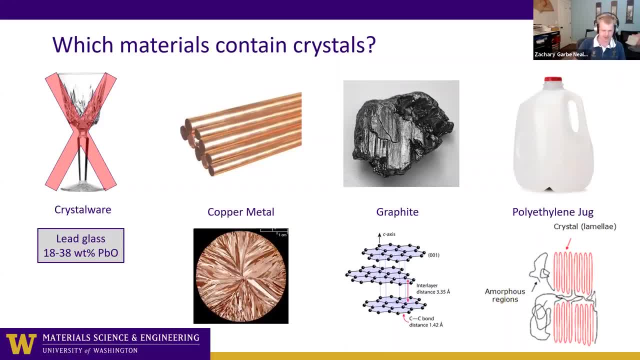 but in fact it's actually amorphous. does it make it melt into molds? yes, but, related to the manufacturability, it makes it easier to cut. so make these facets and there's actually been some studies that look at, you know, different types of beverages: acidic. 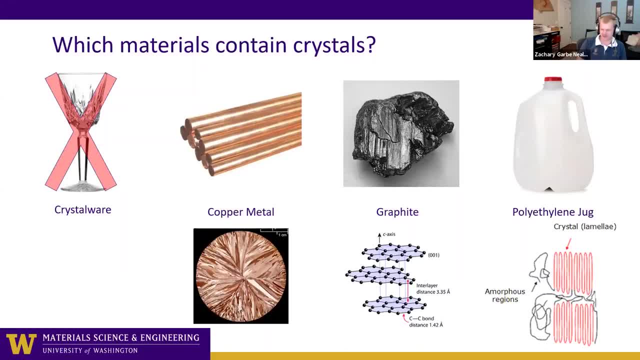 it's all right. The crystalware: does anyone know what type of glass crystalware is? Or what the chemical, what the major? what's the chemical formula that makes crystalware unique? And it doesn't look like anyone knows So. crystalware, boron, silicate, nope. 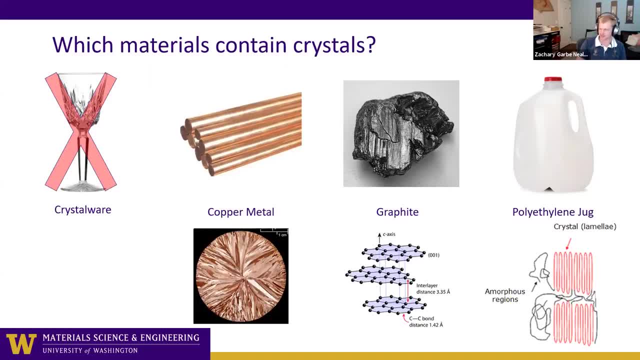 not quite. It's not a boron silicate glass like. Pyrex is a boron silicate glass. Crystalware is a lead glass, So you know if you have any fine crystal in your house it contains a bit of lead. 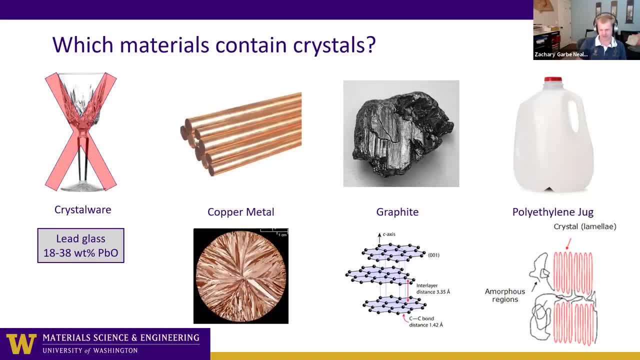 oxide and the reason why. does anyone know why? Well, I guess you might not know because you didn't know the first question. The reason why crystalware uses lead oxide is that the lead oxide component in glass adding lead oxide to this glass. 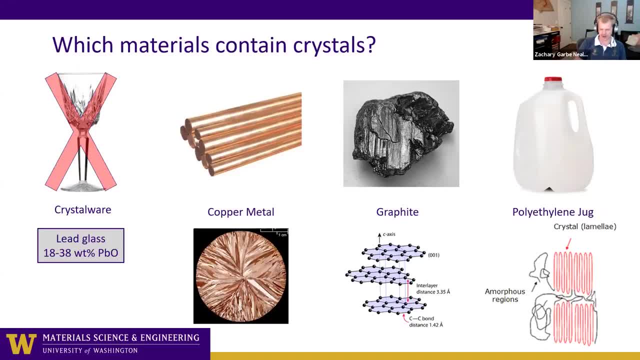 increases the index of refraction. all right. The refractive index So it makes it so the light that bounces in bounces out at a higher angle, and so it makes it optically attractive. right, Like diamond, has a very high index of refraction. Cubic zirconia has a very high index of refraction. 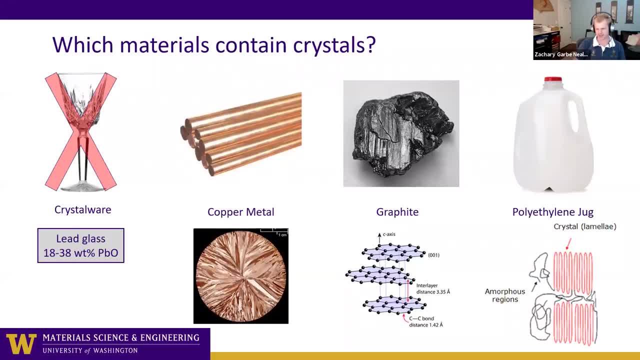 That's why we use it as a substitute for diamond in jewelry. Lead glass also has a fairly high index of refraction. The other reason why lead glass is used for crystalware is that it makes it easy to machine. It makes it it softer. it's easier to cut these facets into the glass to make it, as we call it, a crystal. 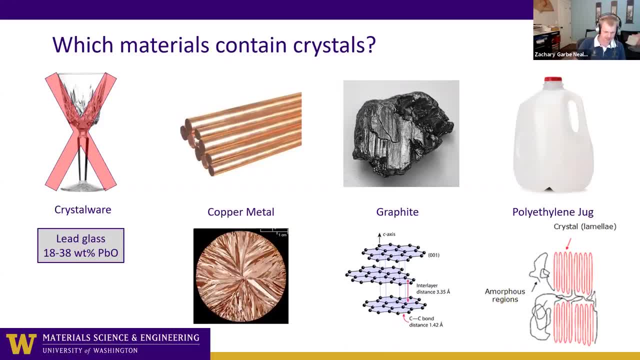 but in fact it's actually amorphous. does it make it melt into molds? yes, but, related to the manufacturability, it makes it easier to cut to make these facets, and there's actually been some studies that look at, you know, different types of beverages, acidic beverages like wine, and how much. 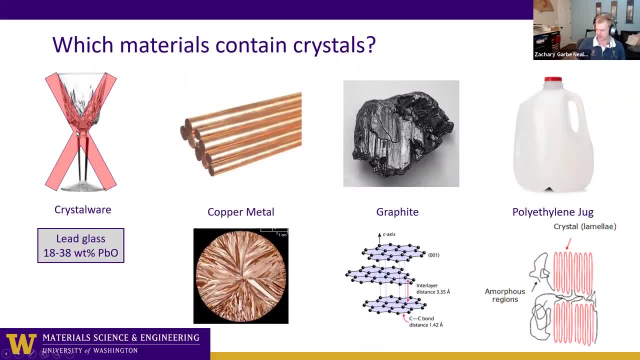 lead is actually leached out of the wine, so you got to be a little bit careful. actually, my family has a bunch of crystal glass that we use almost every day, so i should probably check in the how safe it actually is anyways, just uh, and here's another example of crystals in real life. 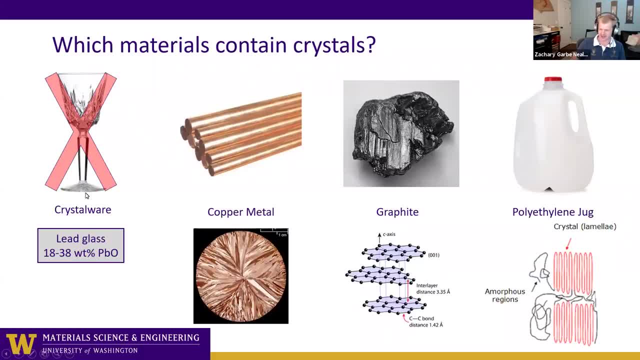 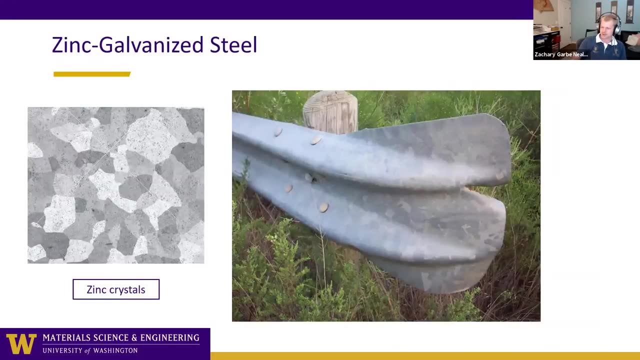 beverages like wine, and how much lead is actually leached out of the wine. so you got to be a little bit careful. actually, my family has a bunch of crystal glass that we use almost every day, so i should probably check into how safe it actually is anyways. just uh, and here's another example of 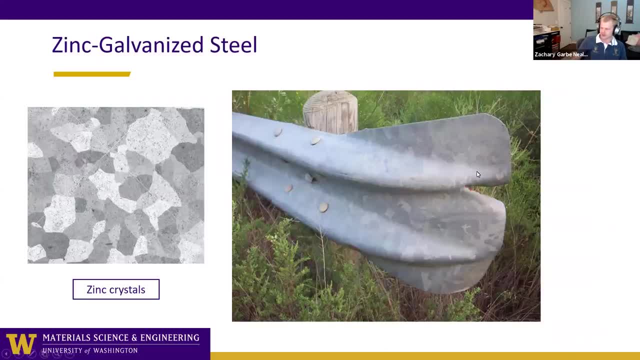 crystals in real life. so you might have seen these guard rails or like light posts, lamp posts, hand rails that are zinc galvanized. right, so they're. they're made out of steel, but they're dip coated in zinc, metal and uh to act as a corrosion protection for the. the steel or iron, and the zinc makes these very 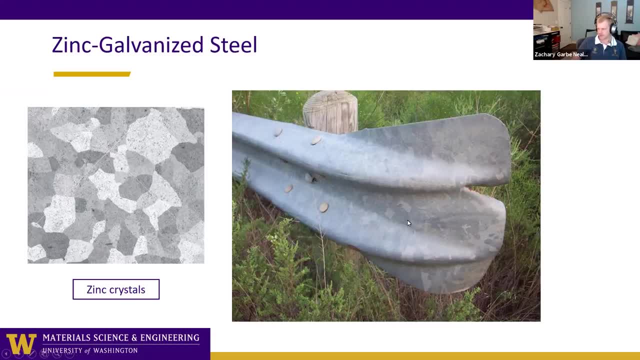 beautiful uh crystals and the the shape and size of these crystals. this is called a spangle. all right, you can have different types of spangle and, depending on the different additives you put into the zinc alloy, you can make them smaller or bigger. uh for different optical properties, but it's 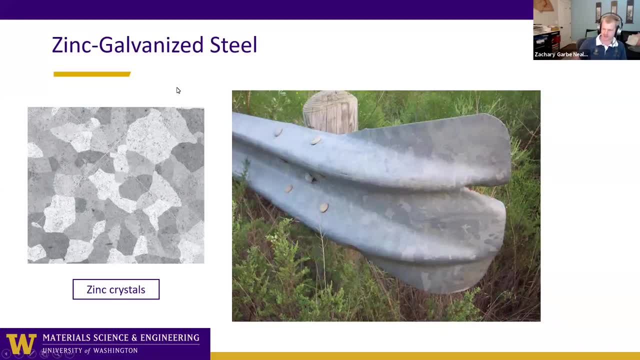 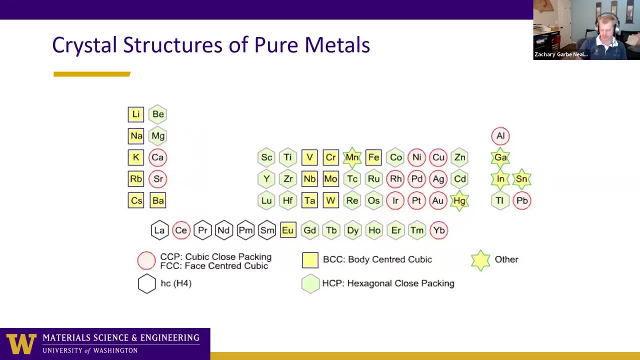 mainly for corrosion prevention. so next time you're at the street corner and you take a look at if the lamp post is uh zinc galvanized, you can see spot out these giant crystals. um so metals, the element, pure elements, uh have a variety of different crystal structures and we're 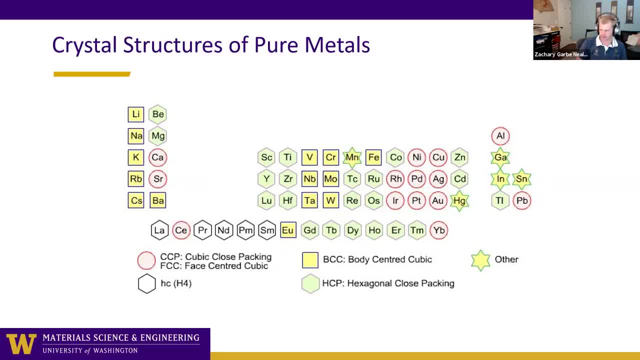 going to look at some of the more common crystal structures. that duck brush has already covered, but you can see how the crystal structures follow. you know these different chemical groups so obviously you know how the atoms arrange depends on the, the electron configuration, uh in in the chemistry of 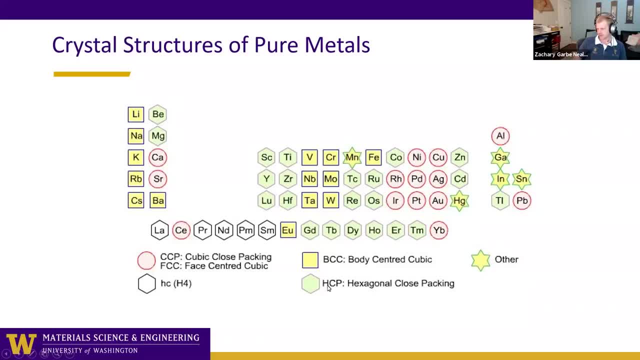 the atoms um some, so the common ones are the the face centered cubic, also known as cubic close packing. all right, so nickel, copper, silver, gold, aluminum, those are the very common uh face centered cubic metals um. and then bcc is another common iron at room temperature is bcc um. 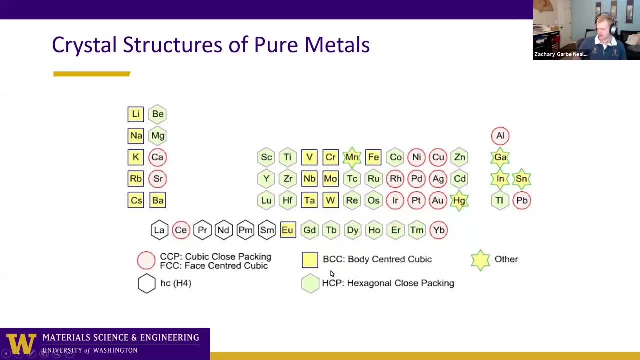 is technically a carbon rock and the alkali metals are also bcc. and then hexagonal closed pack is also the common uh element or crystal structure we talk about titanium specifically is uh when when i think of hcp, i always think of titanium metal. um, yes, some some of the crystal structures will change. 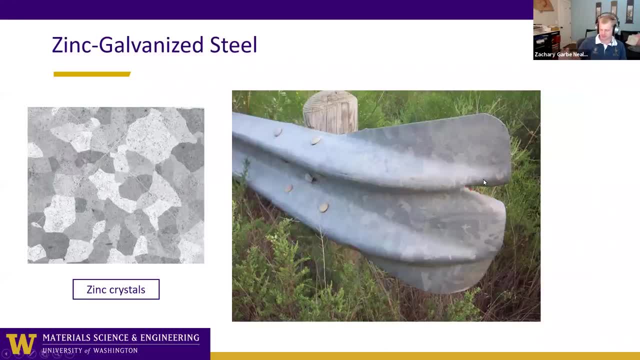 so you might have seen these guard rails or like light posts, lamp posts, uh, handrails that are zinc galvanized, right, so they're made out of steel but they're dip coated in zinc metal and uh to act as a a material that's made out of steel but they're dip coated in zinc metal and uh to act as a a. 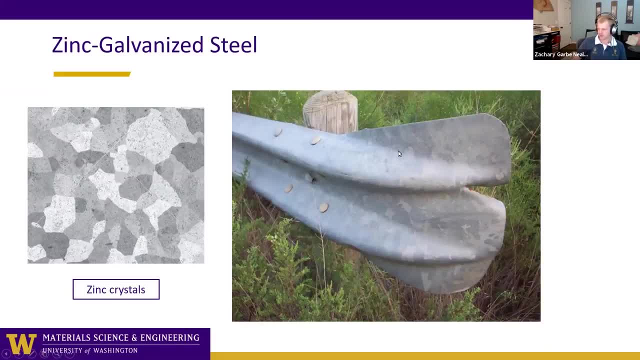 corrosion protection for the, the steel or iron and the zinc makes these very beautiful uh crystals and the the shape and size of these crystals. this is called a spangle. all right, you can have different types of spangle and depending on the different additives you put into the zinc alloy. 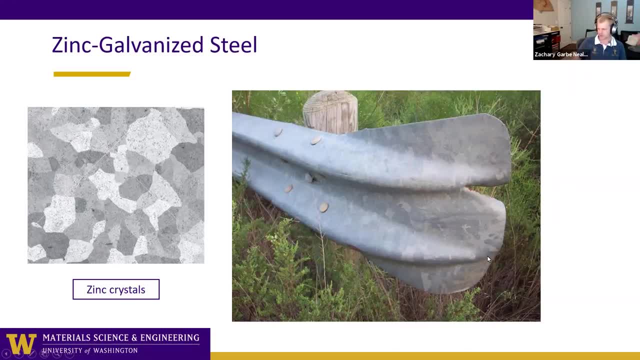 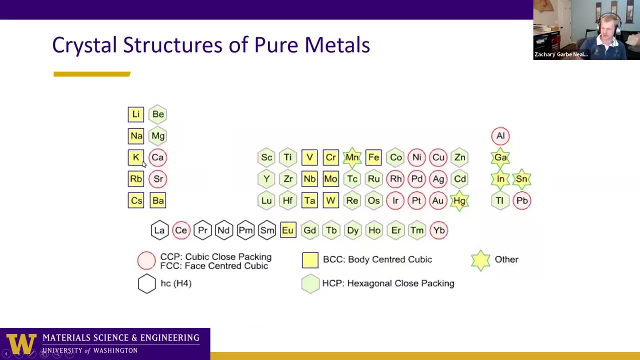 you can make them smaller or bigger for different optical properties, but it's mainly for corrosion prevention. so next time you're at the street corner and you take a look at if the lamp post is, uh, zinc, galvanized, you can see spot out these giant crystals. um so metals, the element pure, 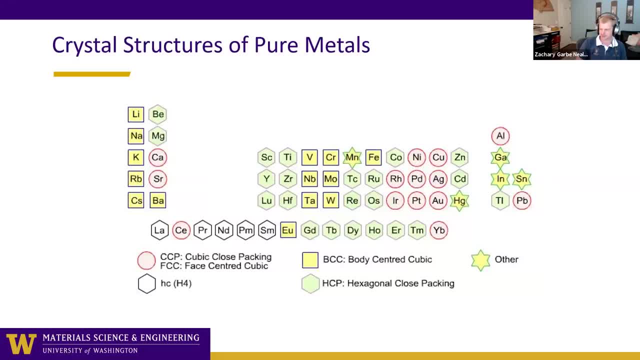 elements, uh, have a variety of different crystal structures and we're going to look at some of the more common crystal structures that doug brush has already covered, but you can see how the crystal structures follow. you know these different chemical groups, so obviously you know how the 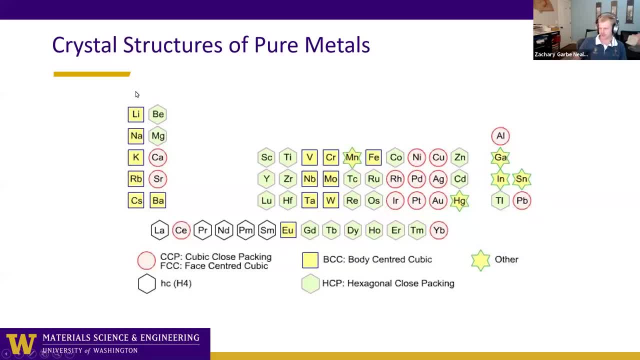 atoms are ranged depends on the, the electron configuration, uh in in the chemistry of the electron configuration, uh in in the chemistry of the electron configuration, uh in in the chemistry of the the atoms um some. so the common ones are the the face centered cubic, also known as cubic. 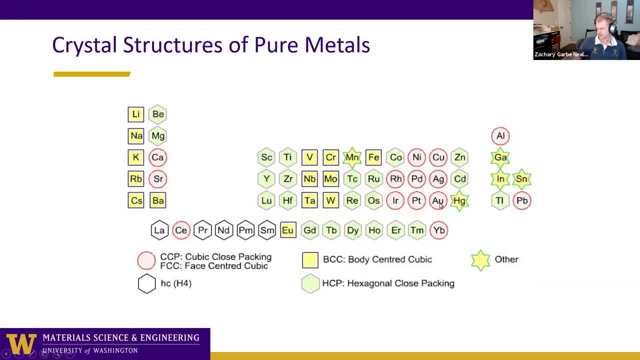 close packing, all right. so nickel, copper, silver, gold, aluminum, those are the very common face centered cubic metals, and then bcc is another common. iron at room temperature is bcc, and the alkali metals are also bcc. and then hexagonal closed pack is also the common 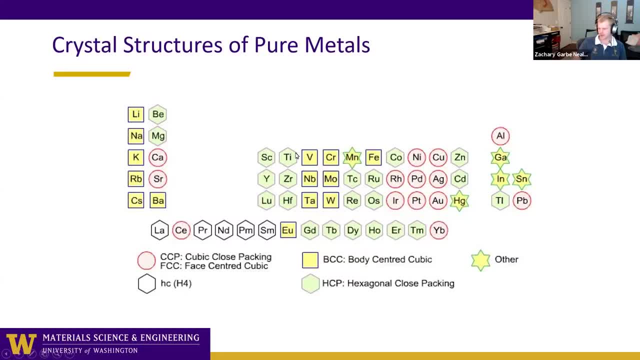 uh element or crystal structure we talk about titanium specifically is when, when i think of hcp, i always think of titanium metal. um, yes, some, some of the crystal structures will change at different temperatures. uh, iron is is the the obvious example of that. at a higher temperature- i forget which, what temp is. 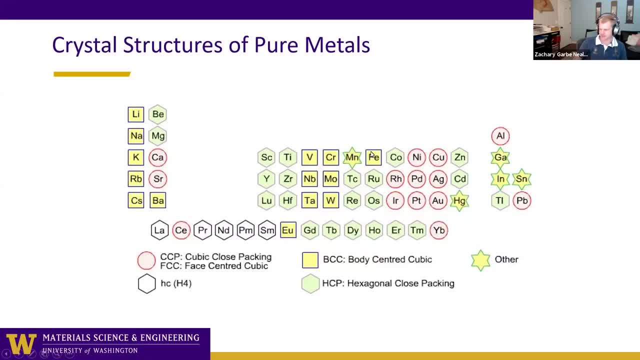 at different temperatures. uh, iron is is the the obvious example of that. at a higher temperature- i forget which what temp is like 700 and something degrees celcius, and and then the crystallized metal see a 724 or something like that. it changes from BCC into FCC, And then at an even higher 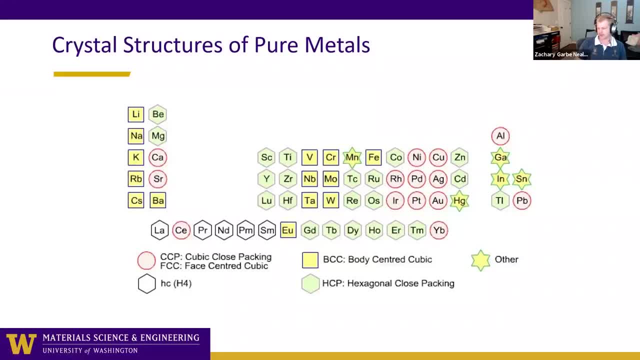 temperature it changes back to BCC. Another interesting thing about the crystal structure of iron is when we start talking about alloys. so we're substituting some of the iron atoms for some other atoms. specifically, stainless steel is made of a nickel iron alloy. There's a large 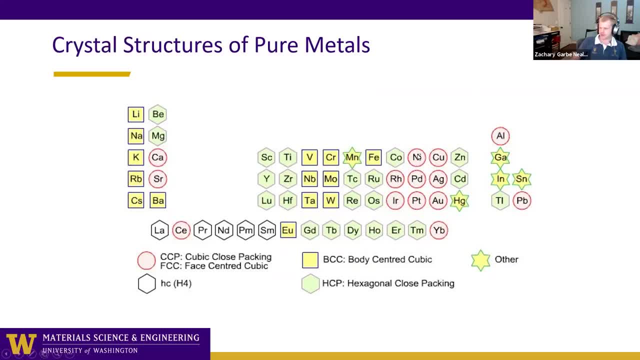 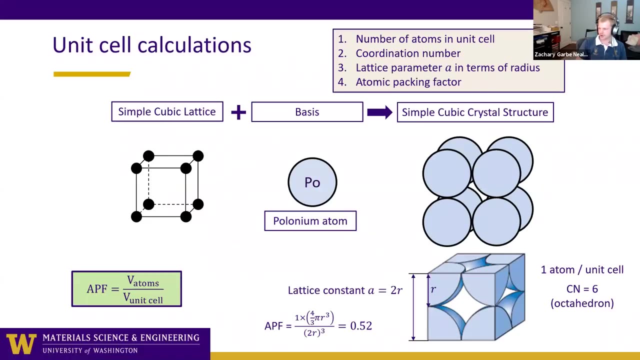 percentage of nickel. So if you put a large percentage of nickel substitute with the iron, what happens is your crystal structure changes. The crystal structure of stainless steel is FCC, not BCC. All right, let's move on. So we're coming to our first question, first problem. 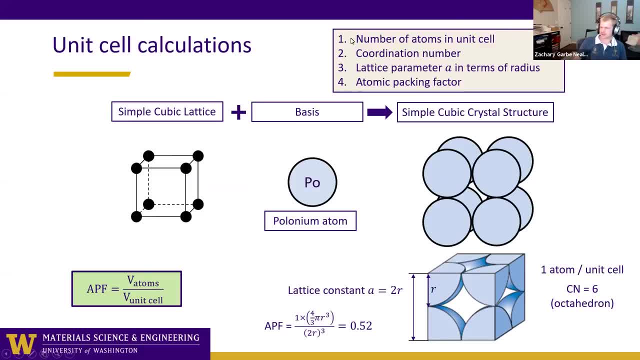 is unit cell calculations. I'm going to have you guys do these number of problems. I'm going to have you guys do these number of problems. I'm going to have you guys do these number of problems for each unit cell. The first is the number of atoms in the unit cell. 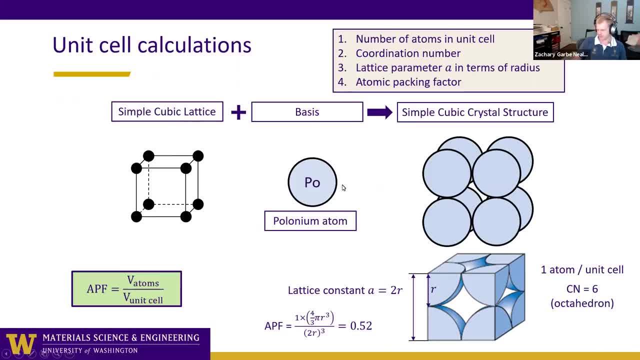 So in this example, it's just the simple cubic lattice And, as Dr Brush had said, polonium is the only single element that forms a simple cubic lattice. All right, the crystal structure is simple cubic And we'll talk about this a bit more. The crystal structure is made up of a lattice. 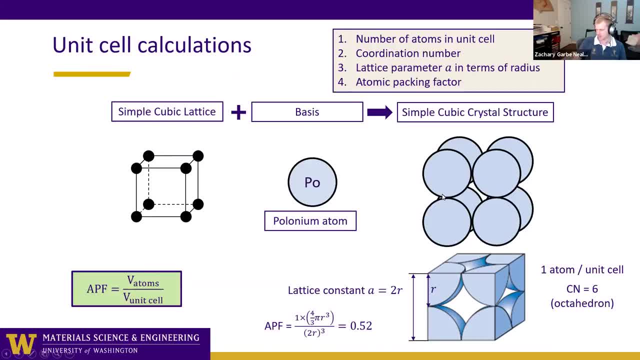 points and a basis. In this case it's just a single atom, All right, and so the number of atoms in the unit cell is the number of atoms in the unit cell. So for a simple cubic it's rather easy. Each corner, there's eight corners, and each corner has one eighth of an atom, So there's one. 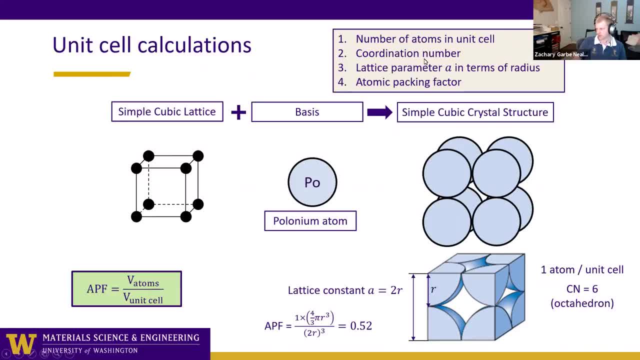 atom per unit cell. Okay, and then you want to find out the coordination number. So this is the number of nearest neighbors for any atom. They're all, they're all, they're non-unique, right, They're all the same. So if you take one atom here and find its nearest neighbors and you say 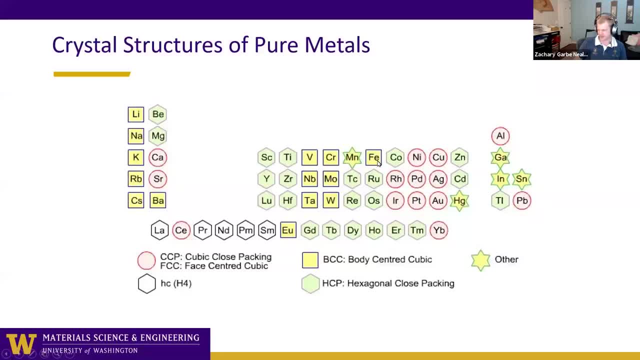 like 700 and something degrees celsius, 724, something like that. it changes from bcc into fcc and then at an even higher temperature, but sure it changes back to VCC. Another interesting thing about the crystal structure of iron is when we start talking about alloys. so we're substituting some of the iron atoms for 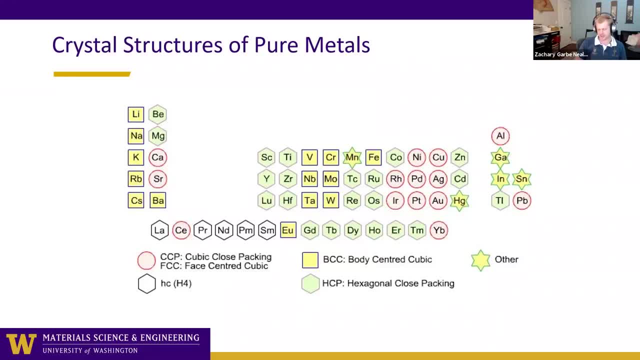 some other atoms. specifically, stainless steel is made of a nickel- iron alloy. There's a large percentage of nickel. So if you put a large percentage of nickel substitute with the iron, what happens is your crystal structure changes. The crystal structure of stainless steel is FCC. 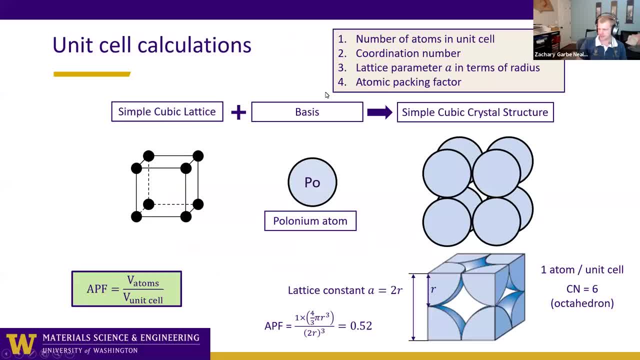 not VCC. All right, let's move on. So we're coming to our first question. first problem is unit cell calculations. I'm going to have you guys do these number of problems for each unit cell. The first is the number of atoms in the unit cell. So in this example it's just the 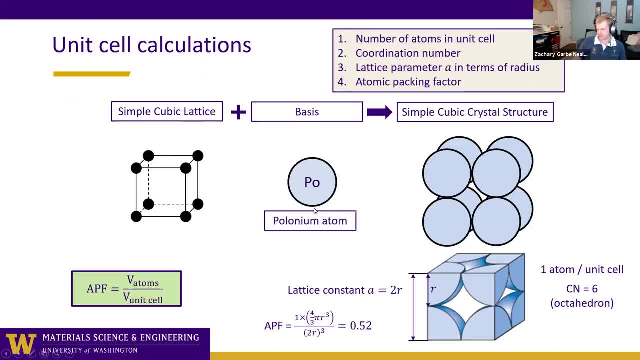 simple cubic lattice And, as Dr Brush had said, polonium is the only single element that forms a simple cubic lattice. All right, the crystal structure is simple cubic And we'll talk about this a bit more. The crystal structure is made up of a lattice points and a basis In. 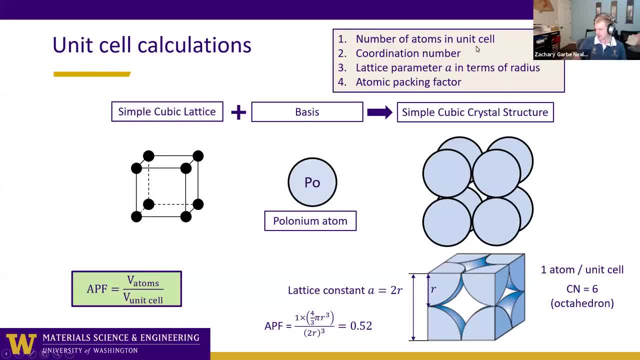 this case it's just a single atom. All right, and so the number of atoms in each unit cell you need to calculate, for simple cubic is rather easy. Each corner, there's eight corners, and each corner has one eighth of an atom, So there's one atom per unit cell. Okay, and then you want to find out the. 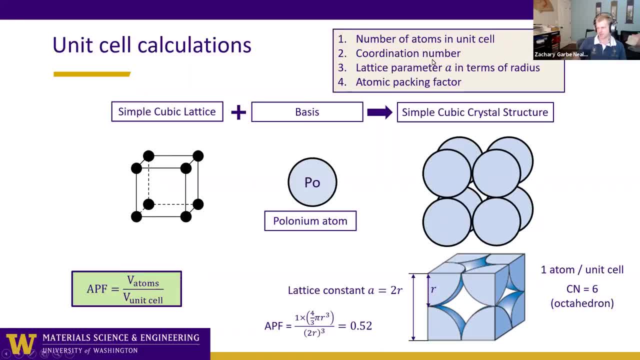 coordination number. So this is the number of nearest neighbors for any atom. They're all, they're all, they're non-unique, right, They're all the same. So if you take one atom here and find its nearest neighbors and you say you have to kind of imagine what does the unit cell above 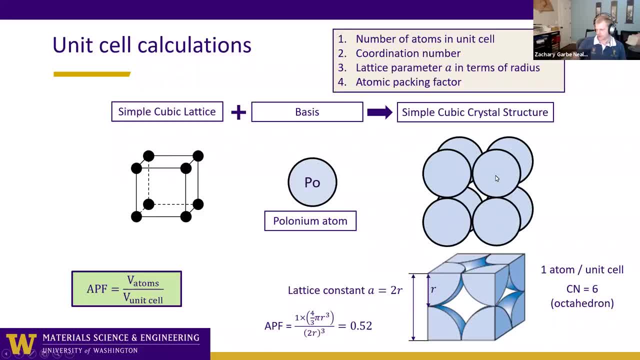 and to the right and in front of it look like. So, if we take this corner atom, there's these three here: one, two, three and there's also a unit cell above and to the right and in front of it. There's also going to be three: there's one above, one to the right and one in front, So the 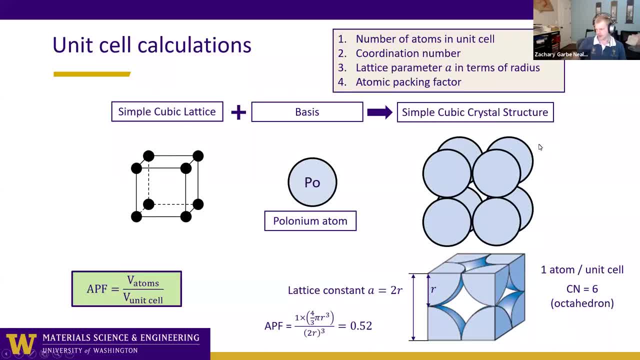 you have to kind of imagine what does the unit cell above and to the right and in front of it look like. So if we take this corner atom, there's these three here: one, two, three and there's also going to be three. there's one above, one to the right and one in front. So the coordination number 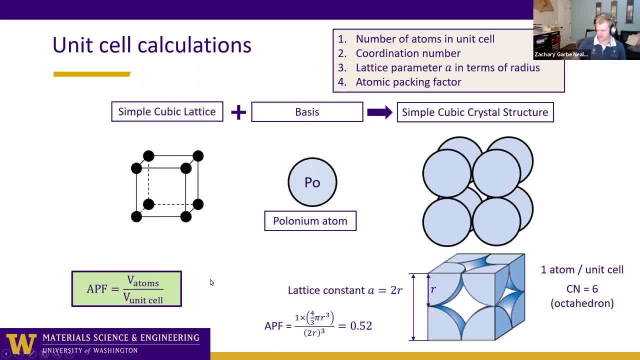 is six, which makes an octahedral coordination Okay. then lattice parameter A, so that's the dimension of the unit cell, okay, and in terms of radius. So a simple cubic is very easy. It's just the two radii. so A equals two R's. 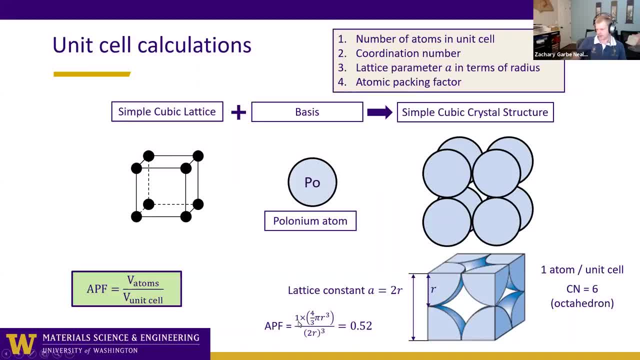 And then also the atomic packing factor. it's going to be the volume of atoms, so four-thirds pi R cubed times the number of atoms in the unit cell divided by the volume of the unit cell. So in this case A cubed which is two R cubed. Okay, so a simple cubic is not very dense, It's a 50%. 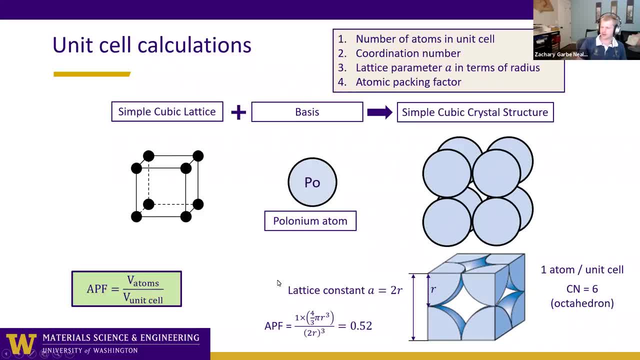 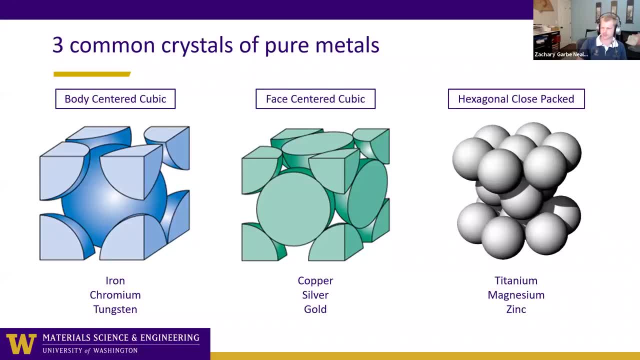 atomic packing factor. All right, I wanted to do this. we're going to do it for body-centered cubic and face-centered cubic, but not hexadecimal. It's a little bit more difficult. I wanted to do this, break you guys into breakout rooms. 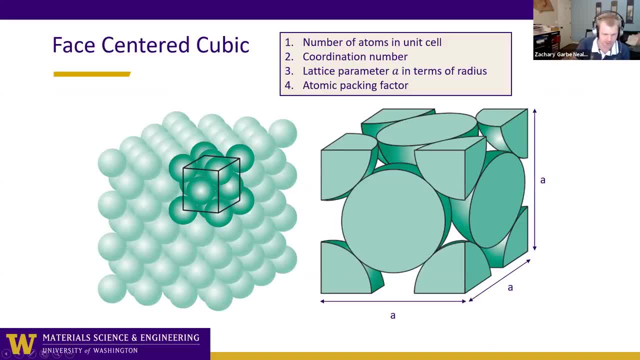 I haven't really prepared it, and then I'll give you about five or so minutes to do it. We're going to start with the face-centered cubic and then, after five or so minutes, I'll call out on a group for the answer. But so when I break you out into breakout rooms, you're, I think you're. 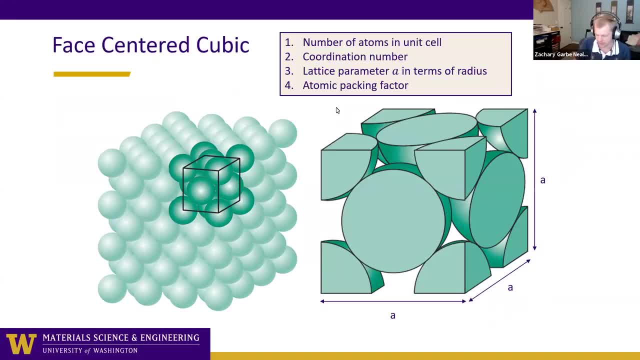 going to lose this page. So what I suggest you doing is, if you're on your computer, if you open up like PowerPoint or Word, you can quickly copy this slide. If you're on Windows, the shortcut for a screenshot is just Windows Shift S, and then it'll allow you to make a 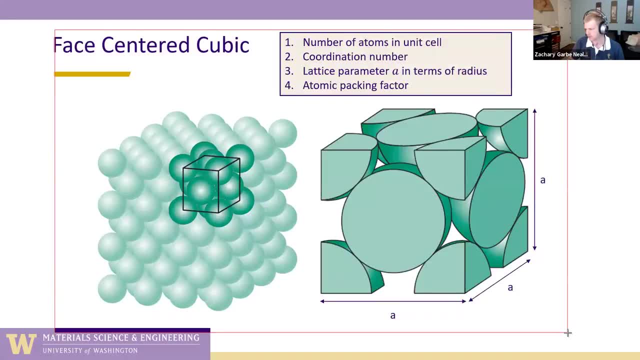 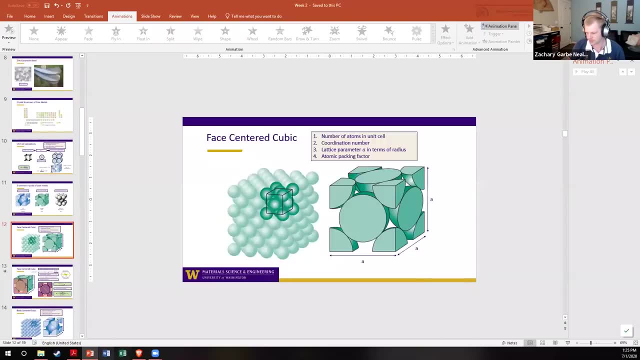 screenshot- I don't know if you can see what I see because of my screen- that gets frozen And then, when you select the area you want to screenshot, it copies it to the clipboard. So, for example, I like to do everything in PowerPoint. 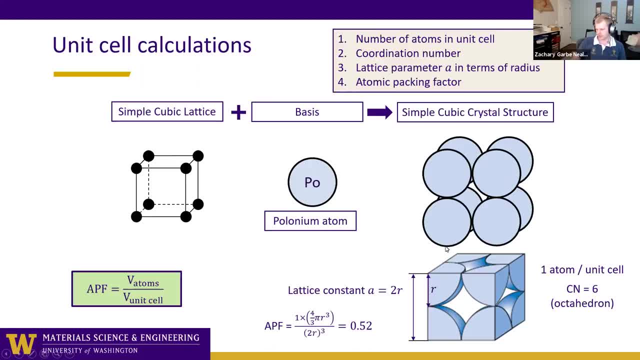 coordination number is six, which makes that octahedral coordination Okay. then lattice parameter A, so that's the dimension of the unit cell. okay, and in terms of radius. So a simple cubic is very easy, It's just the two radii, so A equals two R, and then also the atomic packing. 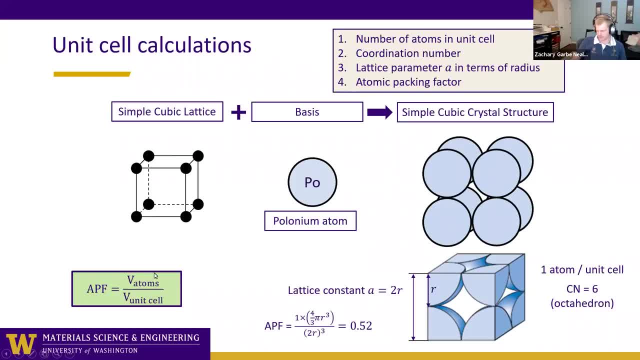 factor It's going to be the volume of atoms, so four-thirds pi R cubed times the number of atoms in the unit cell divided by the volume of the unit cell. So it'll be, in this case, A cubed which is two R cubed. okay, So a simple cubic is: 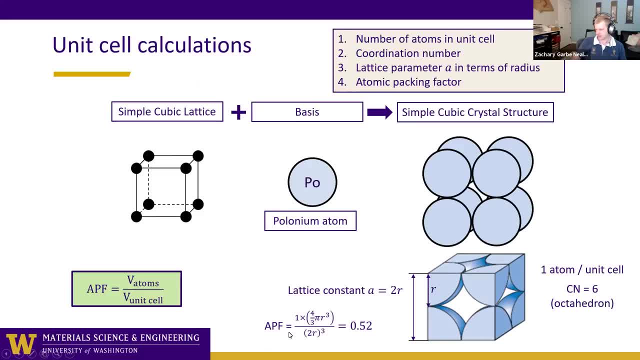 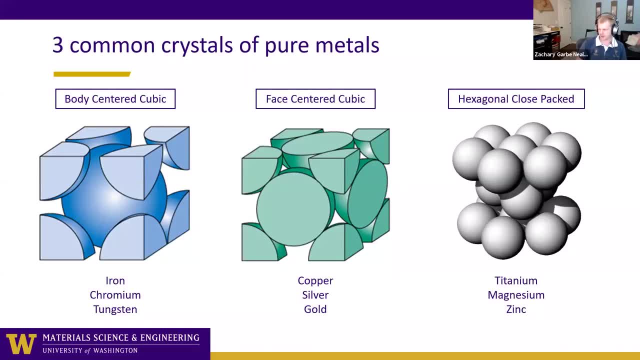 not very dense. It's a 50% atomic packing factor. All right, I wanted to do this. we're going to do it for body-centered cubic and face-centered cubic, but not hexagonal. It's a little bit more difficult. I wanted to do this. break you guys into breakout. 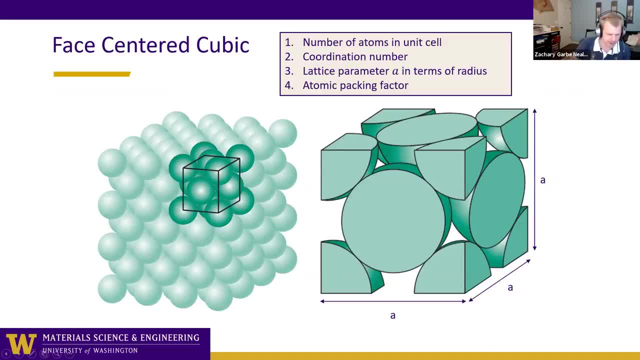 rooms. I haven't really prepared it, and then I'd give you about five or so minutes to do it. We're going to start with the face-centered cubic and then after five or so minutes, I'll call out on a group for the answer. So when I break you out into breakout rooms, I think you're going to lose. 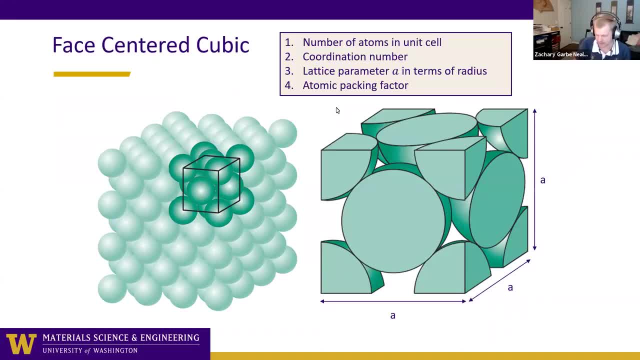 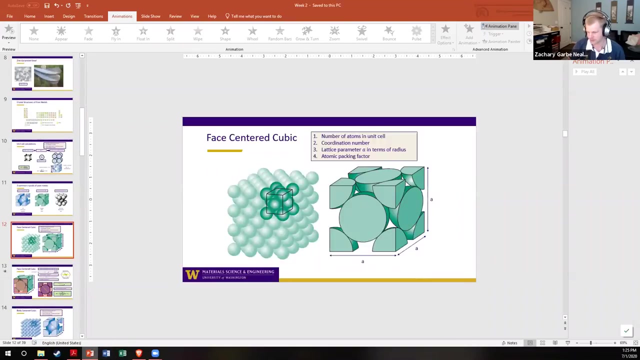 this page. So what I suggest you doing is, if you're on your computer, if you open up like PowerPoint or Word, you can quickly copy this slide. If you're on Windows, the shortcut for a screenshot is just Windows Shift S, and then it'll allow you to make a screenshot. I don't know if you can see what I see because of my screen: that gets frozen And then when you select the area you want to screenshot, it copies it to the clipboard. So, for example, I like to do: 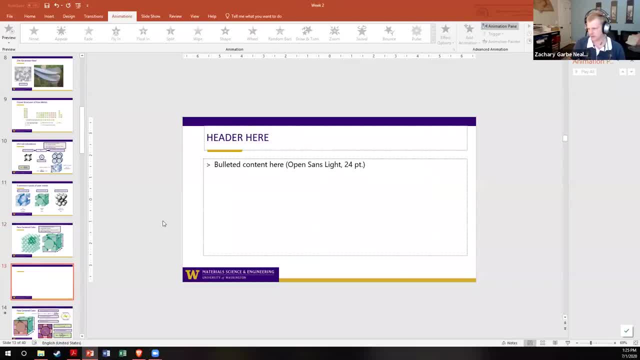 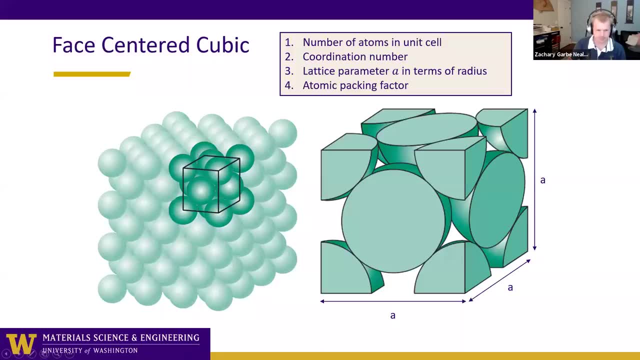 everything in PowerPoint. So yeah, there it is. So that way you have it when I break you out in the breakout room. So I'm going to go ahead and do that. I'll go back here real quick. This is gonna be a little bit of an experiment for me, because I haven't really done this before. Let's see we're going to have 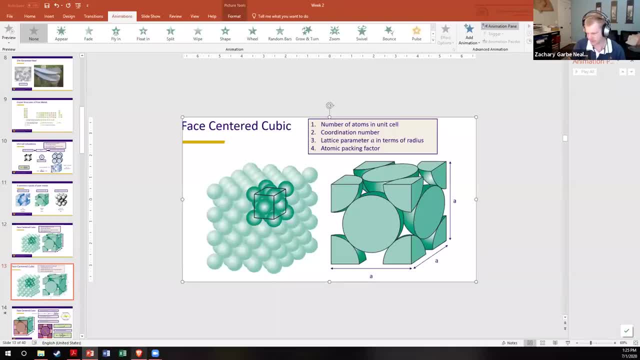 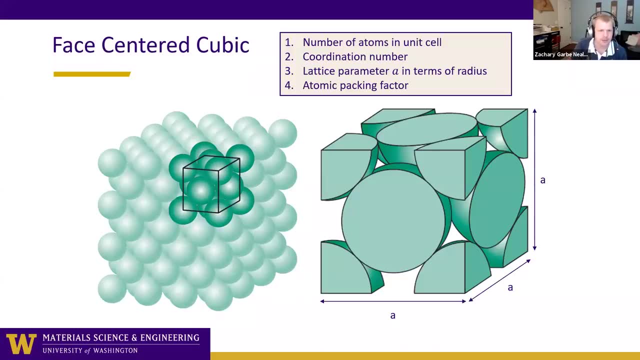 I'll go to edit. So yeah, there it is. So that way you have it when I break you out in the breakout room. So I'll go back here real quick. But this is going to be a little bit of an experiment for me, because I haven't really done this before. Let's see We're going to have 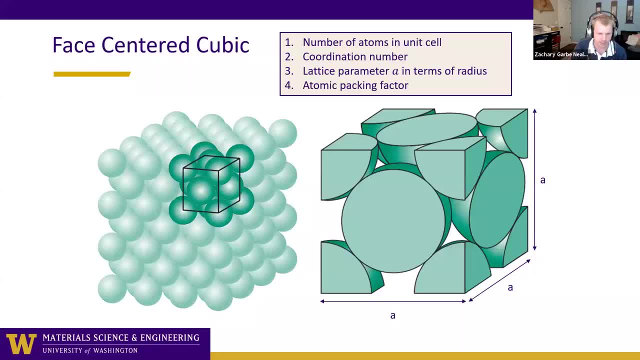 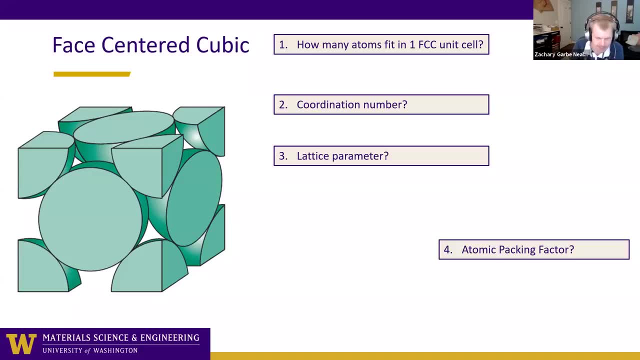 Let's try to get four participants per room. about three to four participants per room. Looks like everyone's back now, So we're gonna go over the answers. I'm gonna pick on people from different groups to give their answer Now, if you don't have an answer, that's okay. 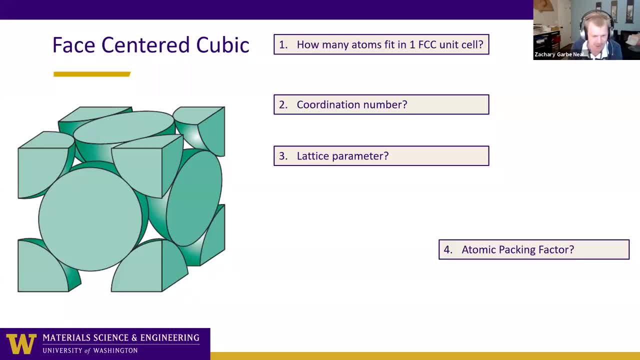 Just say you didn't come up with an answer or whatever excuse you wanna come up with, but it's totally fine. So let's start with from. let's see room one. If you're there, can you answer the first question? 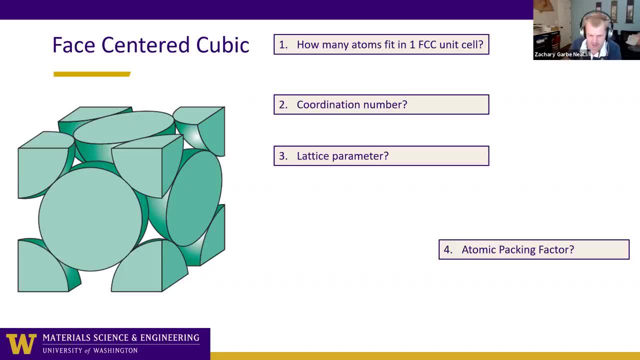 How many atoms fit in one FCC unit cell? Count the number of nearest neighbors or neighbors that are touching. So below it, directly below it, we should have four. right, We have one and two. we can see two here, but there's also two in the back that we can't see. 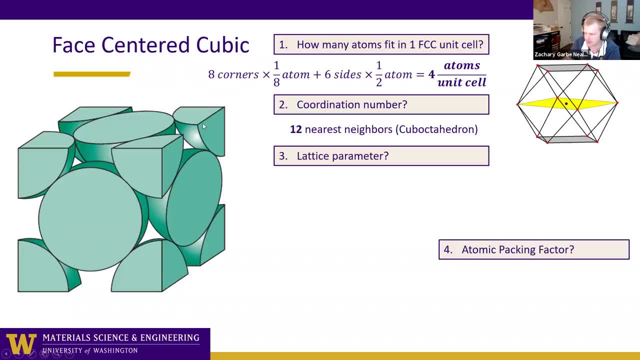 Then along the equator. here we have these four that we can see here, And then directly above it, there's gonna be another four. All right, so four times three is 12. And this makes this symmetry called a cubo-octahedron. 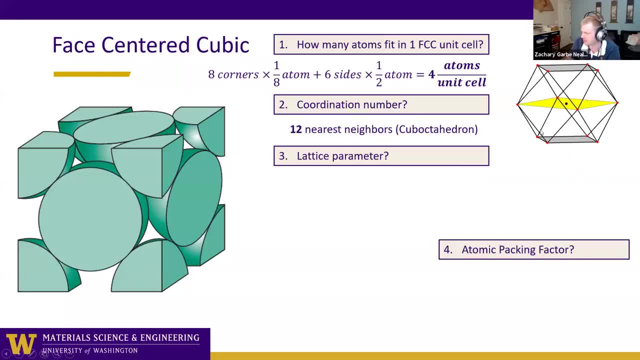 All right. so if you have your central atom and then this is the nearest neighbors, it makes 12 nearest neighbors. All right, how about the next question? last parameter A in terms of radius R. So in this diagram I drew here is just of the face. 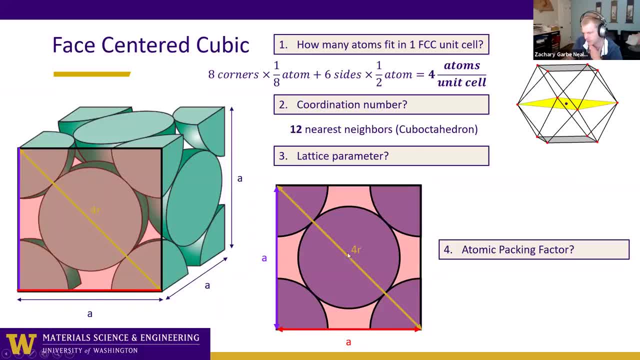 of the FCC unit cell, And we're looking for A in terms of R, the radius of the atom. So here we can draw the shape. We have a triangle where the what is this? The hypotenuse man? it's been a long time. 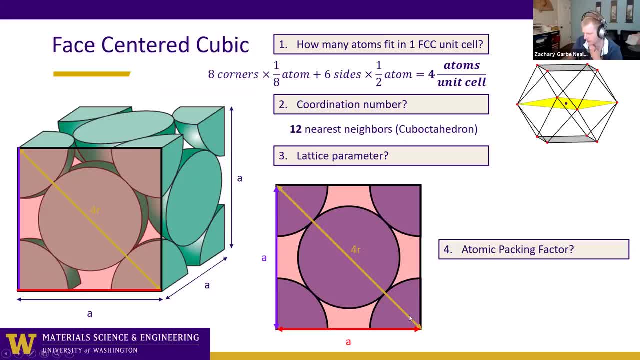 since trigonometry Is equal to four R, All right. and then the legs of the triangle are A, and we can use- what is that? Pythagorean's theorem: A squared plus A, B squared equals C squared, And then you can solve for A in terms of R. 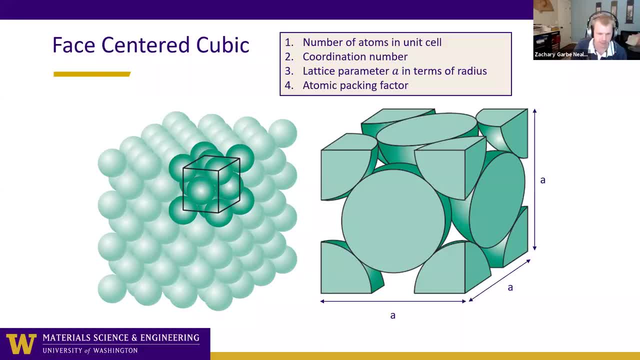 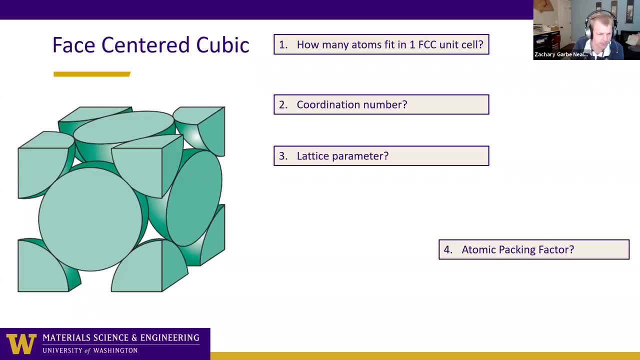 Let's try to get four participants per room. about three to four participants per room. Alright, looks like everyone's back now, So we're going to go over the answers. I'm going to pick on people from different groups to give their answer. Now, if you don't have an answer, that's okay. Just say you didn't come up with an answer or whatever excuse you want to come up with, but it's totally fine. 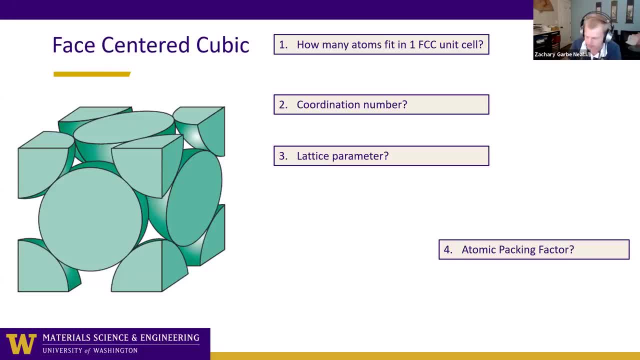 So let's start with from. let's see room one. If you're there, can you answer the first question: how many atoms fit in one FCC unit cell Count the number of nearest neighbors or neighbors that are touching. So below it, directly below it, we should have four. 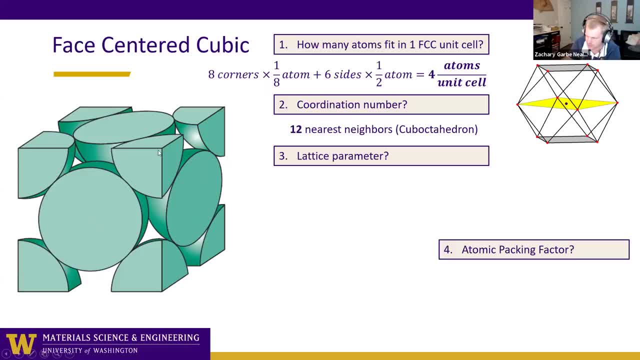 Right, we have one and two. we can see two here, but there's also two in the back that we can't see. Then along the equator. here we have these four that we can see here, and then, directly above it, there's gonna be another four. 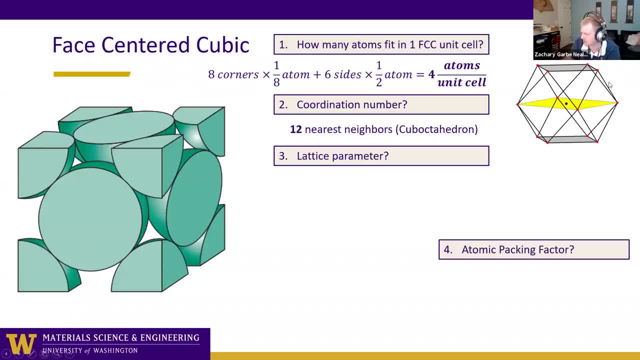 Alright. so four times three is 12. And this makes this symmetry called a cubo-octahedron. Alright. so if you have your central atom and then this is the nearest neighbors round, it makes 12 nearest neighbors, Alright. 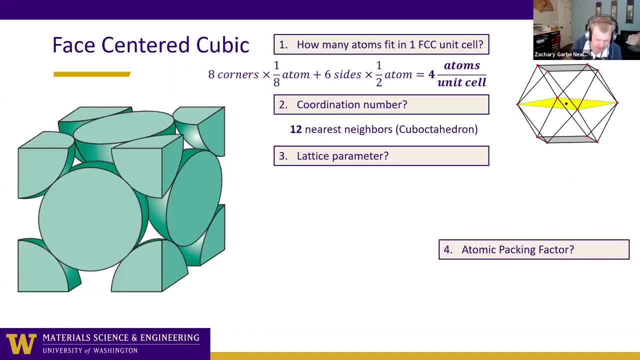 How about the next question? Alright, so we're looking for the last parameter, a in terms of radius r. So in this diagram I drew, here is just of the face of the FCC unit cell, And we're looking for a in terms of r, the radius of the atom. So here we can draw the shape. We have a triangle. 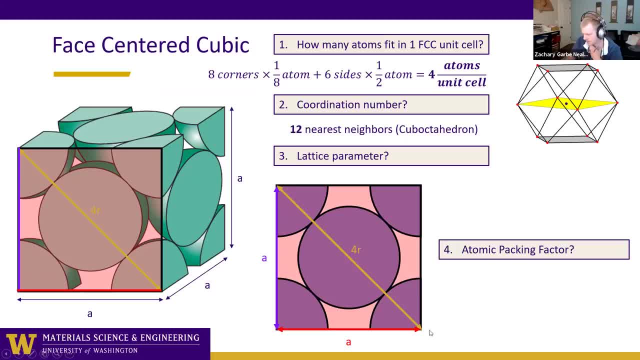 where the? what is this? the hypotenuse man? it's been a long time since trigonometry is equal to four r. Alright, and then the legs of the triangle are a, and we can use- what is that? Pythagorean's theorem: a squared plus a, b squared equals c squared, and then you can solve for a in terms of r. So a equals two r times the square root of two. 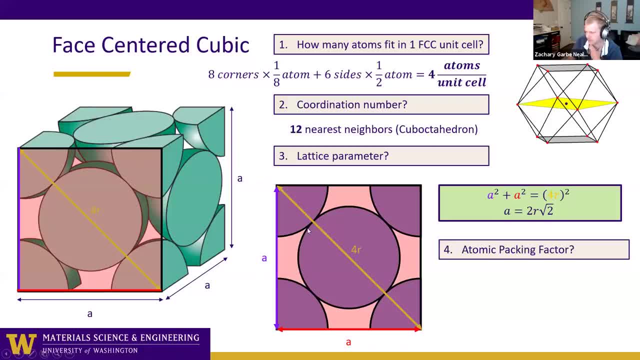 So if you know the radius of any atom, okay, you can calculate. and you know it's FCC crystal structure, then you can calculate its lattice parameter, a, Okay, and then from that you can use it to calculate the density of the material, if you know its molar mass. 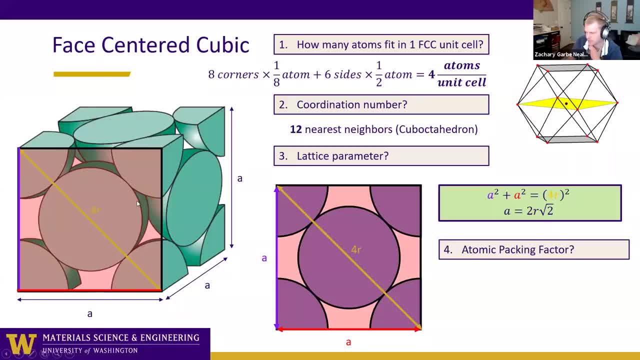 So A equals two R times the square root of two. So if you know the radius of any atom, okay, you can calculate. and you know it's FCC crystal structure, then you can calculate its lattice parameter, A- Okay, And then from that you can use it to calculate. 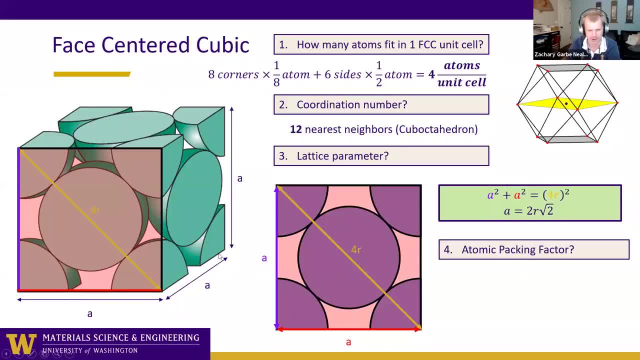 the density of the material if you know its molar mass, 0.74 is correct. yeah, So you just take the volume of the atoms in the unit cell. So we have four atoms times the volume of a sphere divided by the volume of the unit cell. 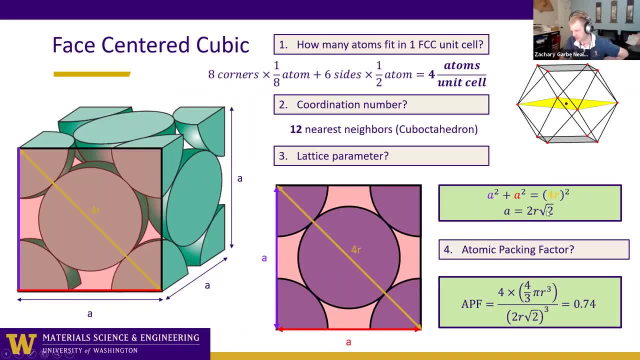 And if you've calculated the parameter- last parameter, just A squared or cubed- excuse me, A cubed- so it's that value cubed, 0.74.. So that's an important number to memorize: 0.74 for FCC, 0.74.. 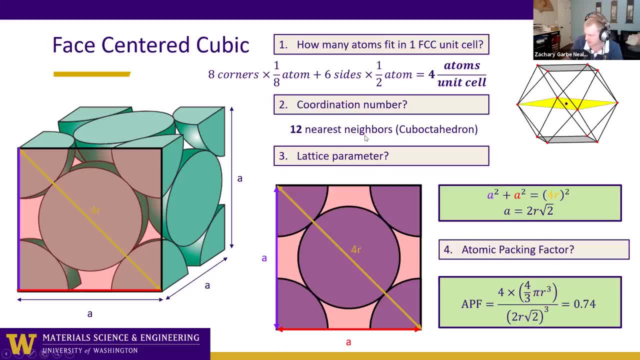 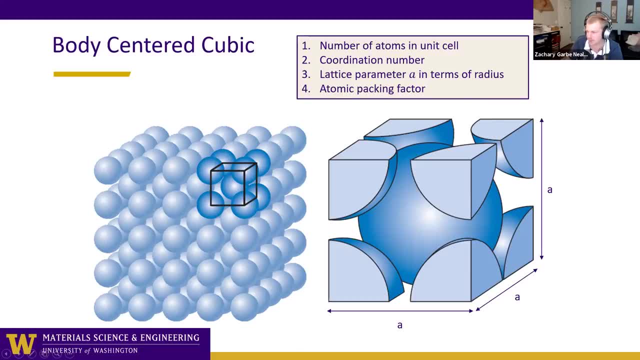 Also, 12 is an important number, and four. So those are the important numbers. Okay, let's move on, And we're kind of it takes a bit of time to go through all this. So I think, if it's okay with you guys, 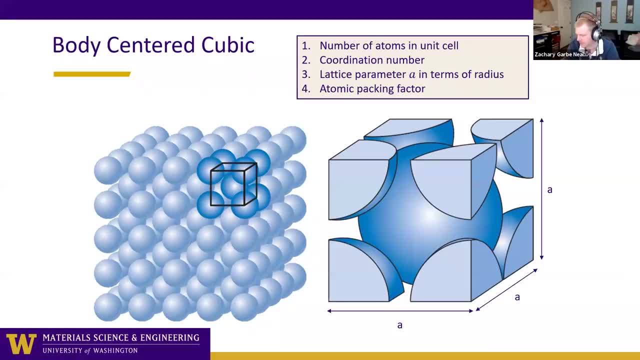 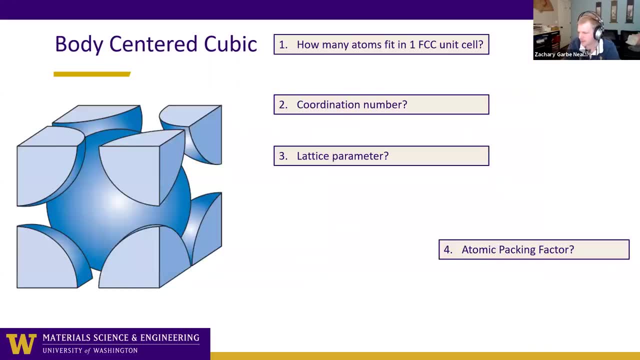 we're gonna just not break out into breakout rooms for this next one, so I can move on to the next content. But the same thing for BCC. So I'll go through it with you or we can just answer out loud. So how many atoms fit in one? this is a typo here. 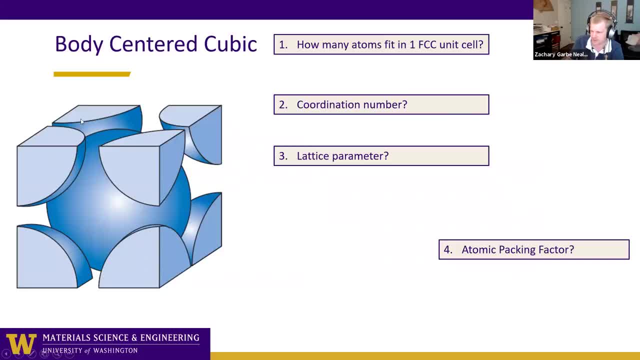 it should say: one BCC unit cell. How many atoms are inside one BCC unit cell? Anyone wanna shout out Two? I think that should be two. Yes, that is two. So how about the coordination number Eight? Eight is correct, right? 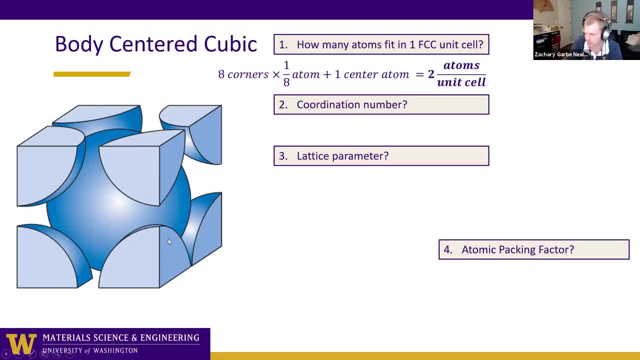 So just take this one atom in the center and it's got eight corners surrounding it. It makes a cubic geometry. How about the lattice parameter? This one's a bit more time consuming, so I'll just go through it. So here I've drawn a shape. 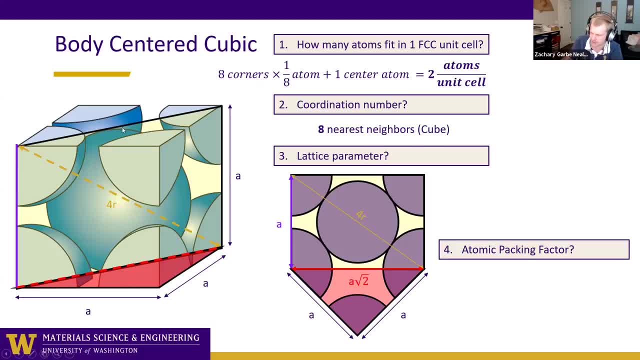 I've drawn a plane that cuts from edge to edge, right down the center of this cube, okay, And I've drawn out the two-dimensional projection of that plane of the atoms And you'll see that there's a continuous three atoms down the center here, and so that's equal to four R four. 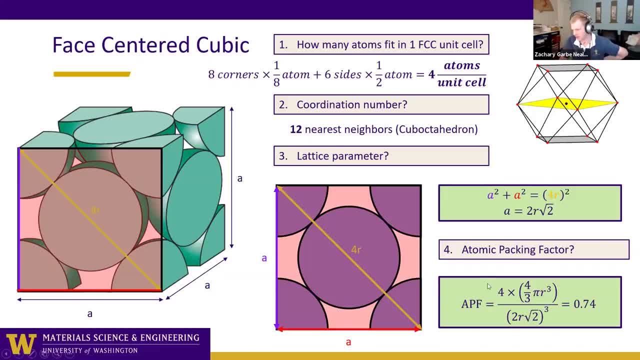 Yeah, so the important thing that we have to remember is that we have to require a constant denominator for any unit cell. 0.74 is correct. Yeah, so you just take the volume of the atoms in the unit cell, So we have four atoms times the volume of a sphere. 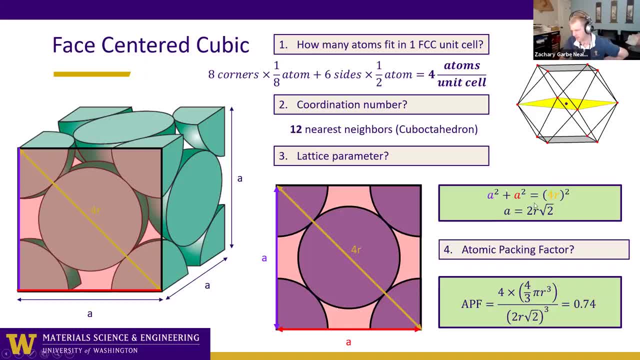 divided by the volume of the unit cell and if you've calculated the parameter- last parameter- just a squared or, excuse me, a cubed, so it's that value cubed, 0.74.. So that's an important number to memorize: 0.74 for FCC, 0.74.. 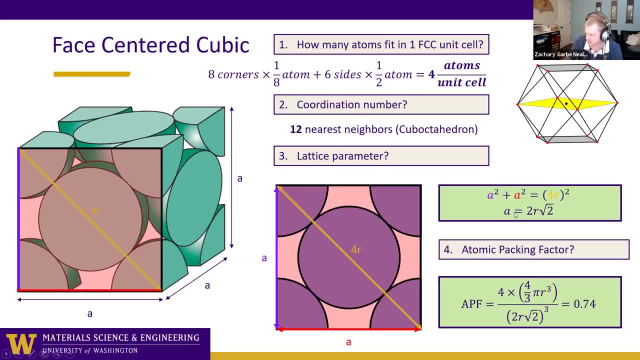 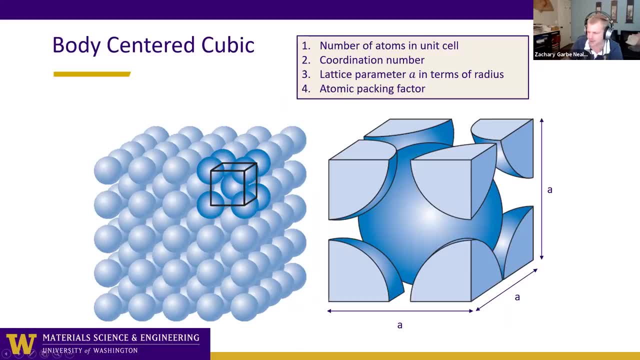 Also, 12 is an important number, and four. So those are the important numbers. are the important numbers? okay, let's move on. um, and we're kind of it takes a little bit of time to go through all this. so i think, uh, if it's okay with you guys, we're going to just not break out. 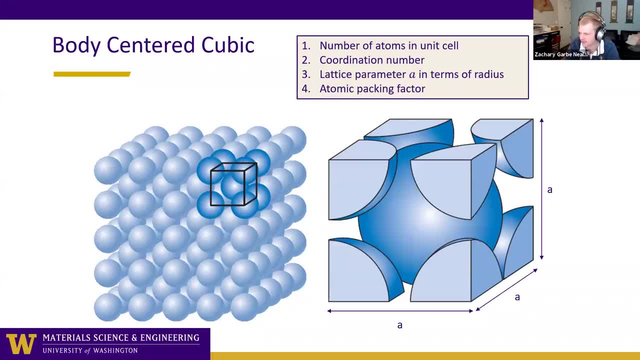 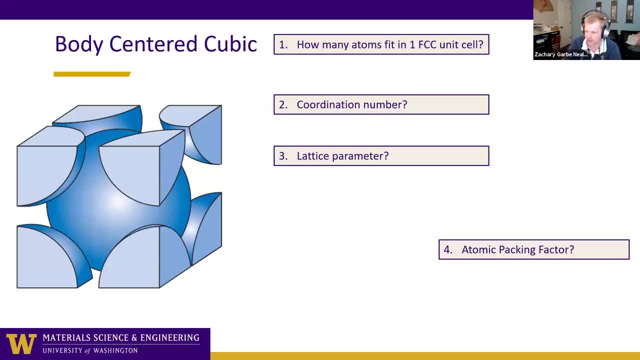 into breakout rooms for this next one, so i can move on to the the next content. um, but the same thing for bcc. so i'll go through it with you, or we can just uh answer out loud: uh, so how many atoms fit in one? oh, this is a typo here. it should say: one bcc unit cell. how many atoms are inside one? 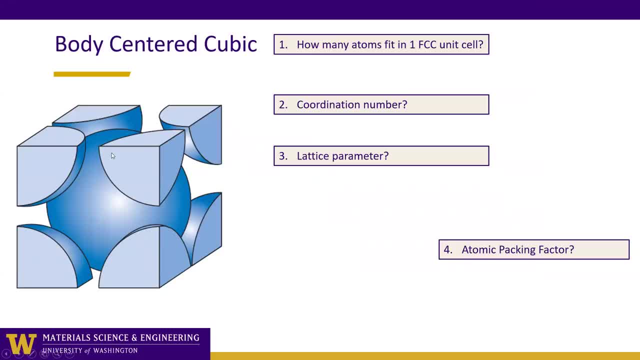 bcc unit cell. anyone want to shout out? i think that should be two. uh, yes, that is two. so how about the coordination number eight? eight is correct, right? so it's just take this one atom in the center and it's got eight corners surrounding it, so it makes a cubic geometry. um, how about the? 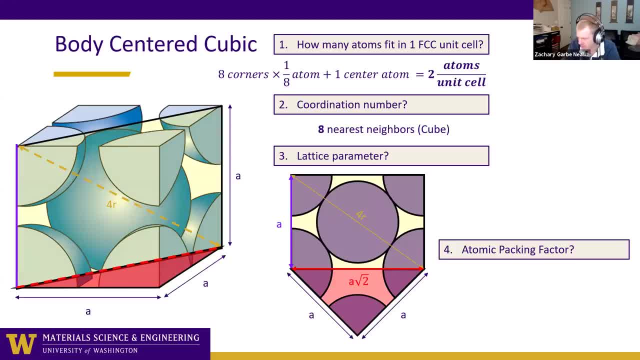 lattice parameter. this one's a bit more time consuming, so i'll just go through it. so here i've drawn a shape, i've drawn a plane that cuts from edge to edge, right down the center of this cube, okay, and i've drawn out the two, the two-dimensional projection of that plane of the atoms and 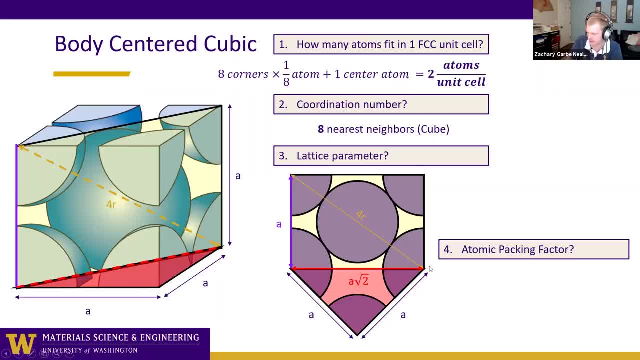 you'll see that there's a continuous uh three atoms down the center here, and so that's equal to four r, four times the radius, and then the edge is the last parameter, a. so that's what we're looking for in terms of r, and then i've also drawn this triangle, which is the. 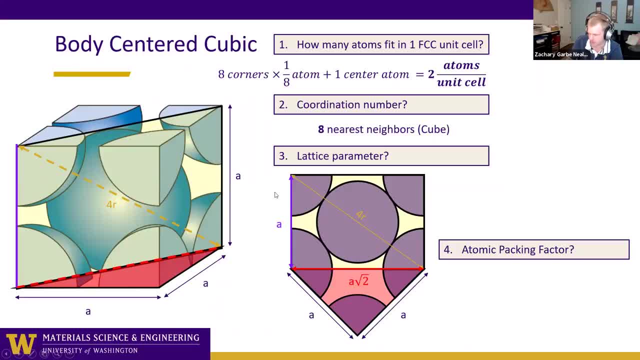 times the radius, And then the edge is the last parameter, A. so that's what we're looking for in terms of R, And then I've also drawn this triangle, which is the base of the square, and so I've kind of unfolded it out. 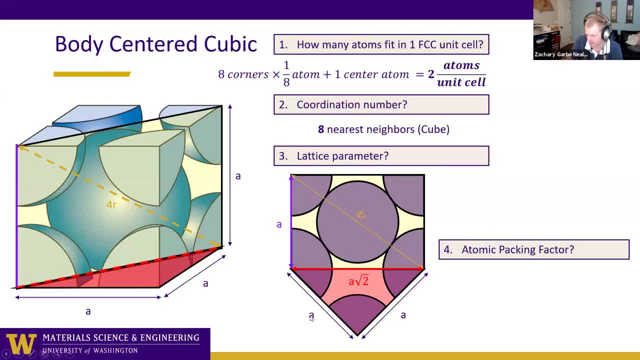 into this two-dimensional projection, kind of like origami here, and it has two last parameters as well, these two edges here. So again through Pyrethagorean's theorem: A squared plus A squared equals C squared, A squared, B squared equals C squared. 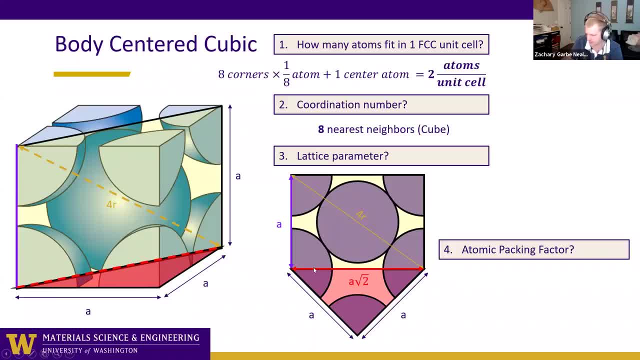 so that makes this edge length here along the diagonal. so that makes this edge length here along the diagonal. so that makes this edge length here along the diagonal A times the square root of two. So now we have our two legs, A and B, and that equals C. 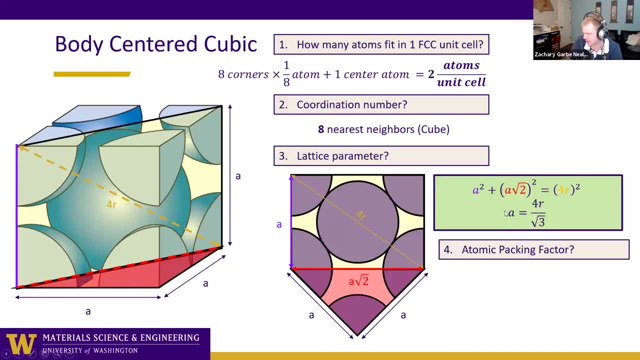 so again Pyrethagorean's theorem, and you get A in terms of R. So A equals four R over the square root of three. How about atomic packing factor? Does anyone know the answer on the top of their head? Yeah, 0.68,. Greece says. 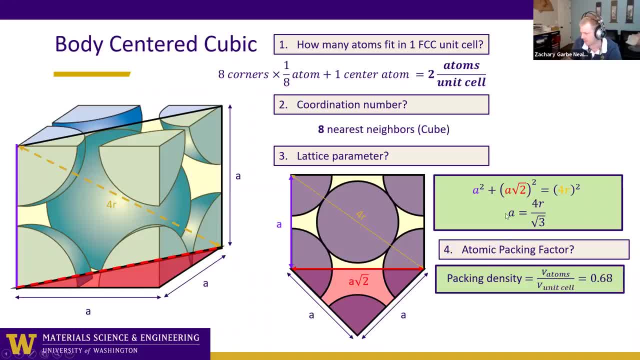 That's correct: 0.68.. So it's the same calculation. You have the information you need but, like I said for cubic, for FCC and BCC and HCP, you should memorize these numbers because they might come up in a test or something. 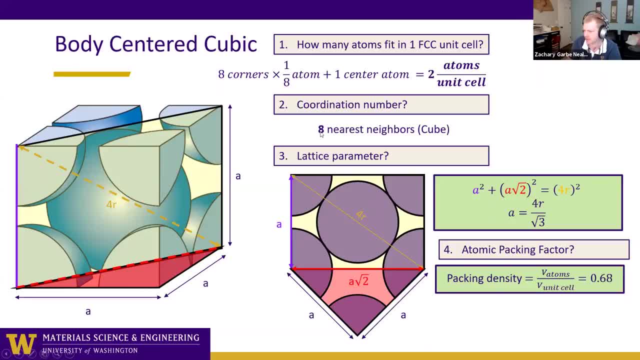 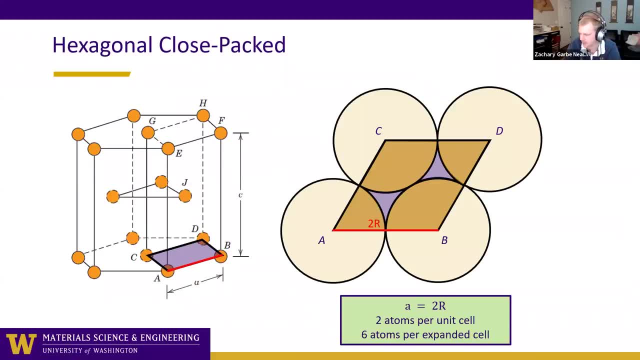 and you don't have to calculate it. Yeah, two atoms per unit cell, eight nearest neighbors, the coordination and 0.68, 68% Hexagonal close pack. not gonna do any calculations, really, but it's just to visualize how the atoms are packed right. 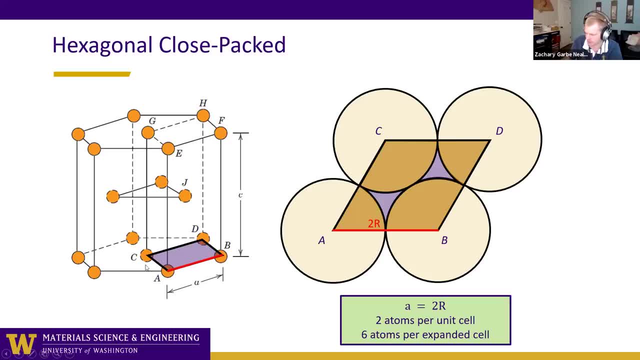 So here's again a two-dimensional projection of just this first layer here and then I move up to the layer above it. okay, So this is that J atom here on the layer above it and then the next layer on top of that. okay. 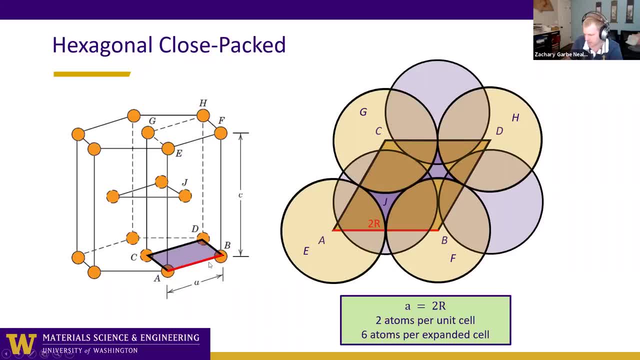 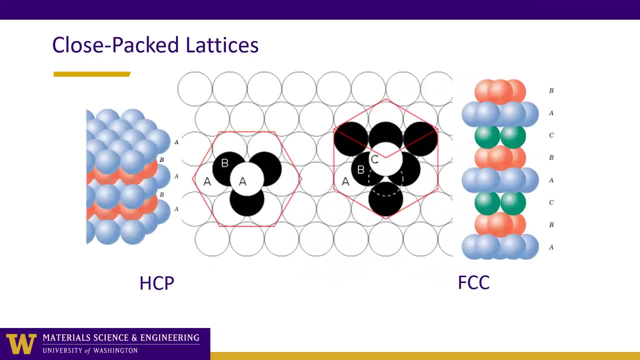 So you get the parameter last. parameter A is just two R and there's two atoms per this unit cell and the smaller unit cell. but the expanded unit cell, the hexagonal unit cell, there's six atoms. But what is important, like Dr Brush had mentioned in class, 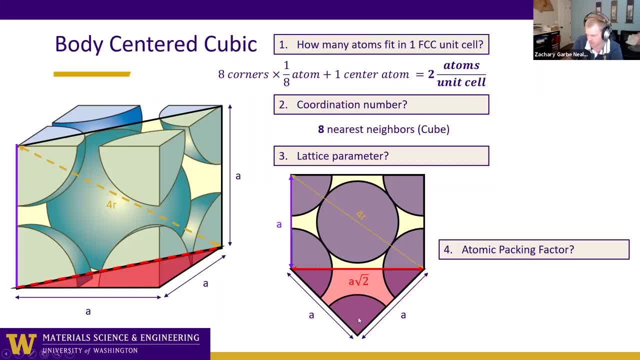 base of the square, and so i've kind of unfolded it out into this two-dimensional projection, kind of like origami here, and it has two last parameters as well, these two edges here. so again through pyrethagorean's theorem, a squared plus a squared equals c squared, a squared, b squared. 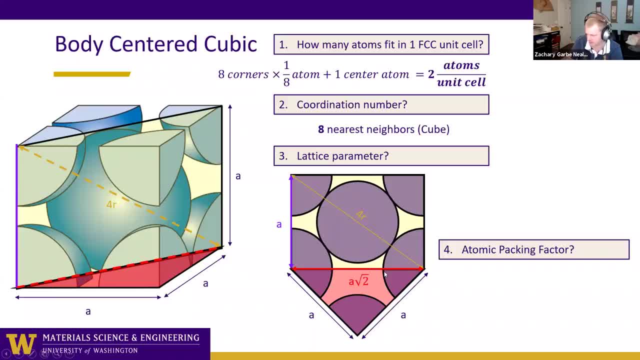 equals c squared. so that makes this edge length here along the, the diagonal, a times squared of two. so now we have our, our, our two legs, a and b, and that equals c. so again pythagorean's theorem. and um you get a in terms of r, so a equals four, r over square root three, um. how about atomic packing factor? 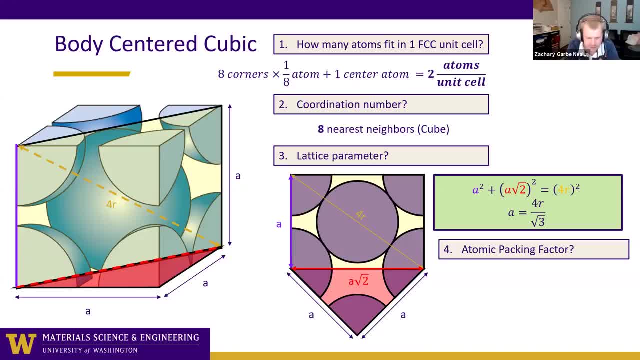 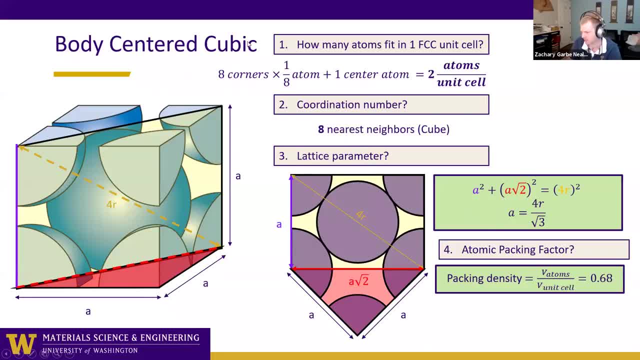 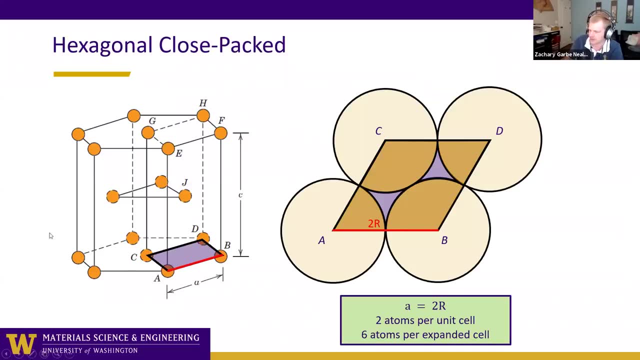 because they might come up in a test or something and you don't have to calculate it. yeah, two atoms per unit cell, eight nearest neighbors, the coordination, and 0.68, 68 hexagonal close pack. not going to do any calculations really, but it's just to visualize, uh, how the atoms are packed. 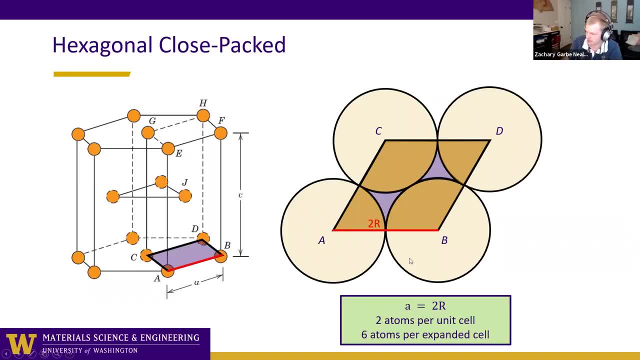 right, um, so here's a again, a two-dimensional projection of just this first layer here, and then i move up to this, the layer above it. okay, so this is that j atom here on the layer above it, and then the next layer on top of that. okay, so you get, uh, the parameter. last parameter, a is just 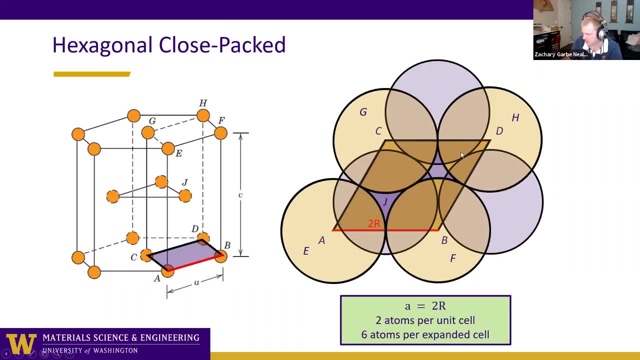 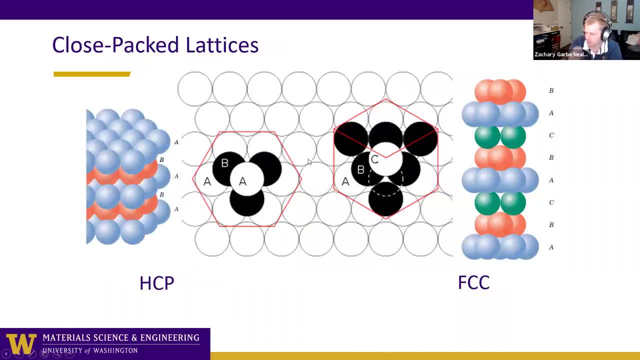 2r and there's two atoms per this unit cell in the smaller unit cell. but the expanded unit cell, this hexagonal unit cell, six non-expanded unit cell and then the last parameter, a, is just the atoms. But what is important, like Dr Brush had mentioned in class, is the similarity between 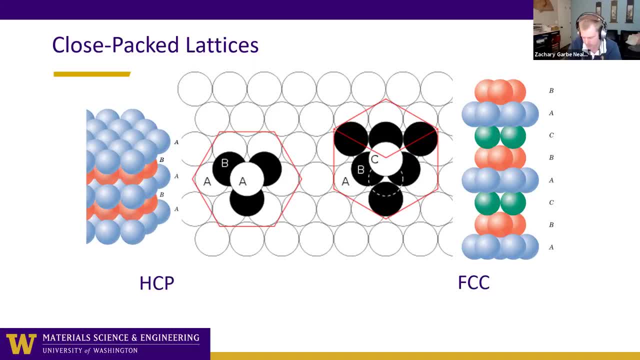 HCP and FCC. They are both closed-packed lattices and they both have the same atomic packing factor right, which was 0.74.. Did I get that one right? I always forget. I haven't memorized it myself. Yeah. 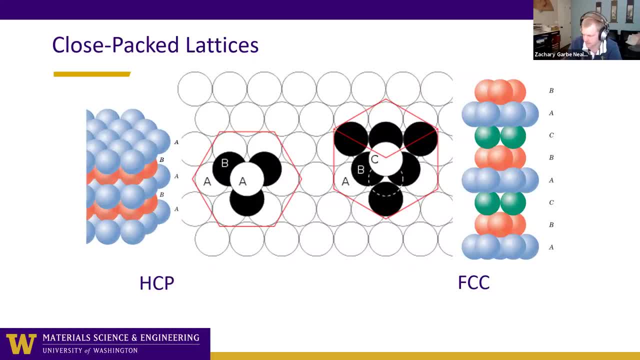 is the similarity between HCP and FCC. They are both close-packed lattices and they both have the same atomic packing factor right, Which was 0.74.. I get that one right. I always forget. I haven't memorized it myself. 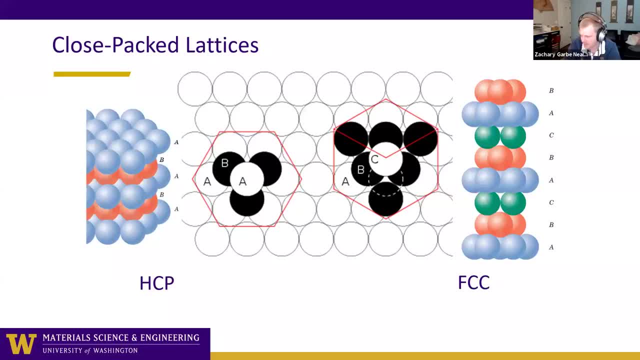 Yeah, 0.74.. Just double checking, All right, so they have the same packing factor and, like Dr Brush had mentioned, the only difference is the. you know, they have these close-packed planes of atoms and the layering sequence is different. 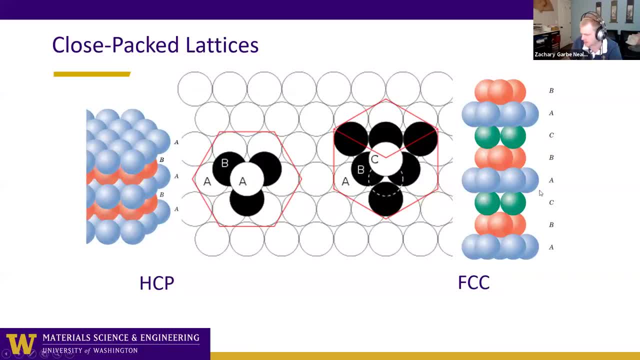 where HCP is ABA and FCC is ABC, And I've tried to visualize this further for the FCC so you can try to see where the cubic structure comes from in this orientation, right, So you can see where this is the FCC, right. 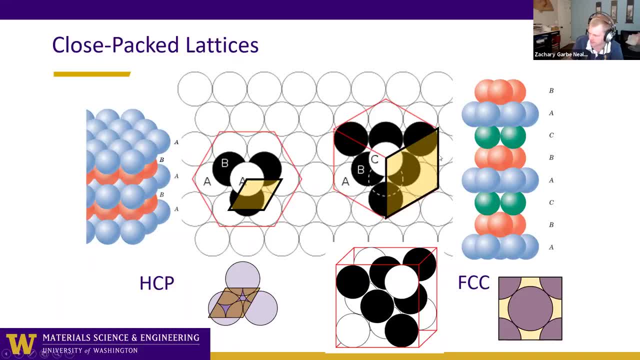 So you can see where. this is the FCC, right, This is the FCC cube. I've taken just this face and the two-dimensional projection of that face, and there's the face-centered face of it. Okay, And then the coordination is the same for both of them. 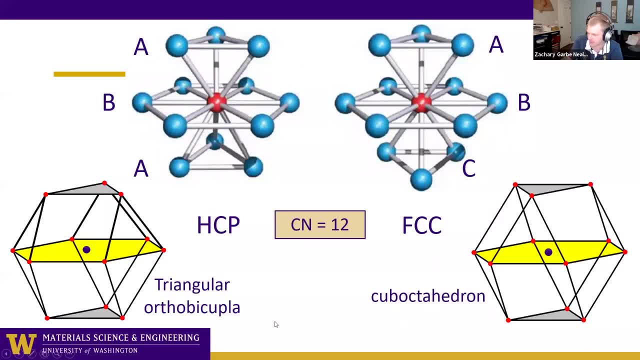 but what is different is the symmetry of that, the geometry, All right. so for HCP, which is ABA, it has this weird shape: triangular, ortho bicouple. You don't need to know the names of anything, This is the HCP. 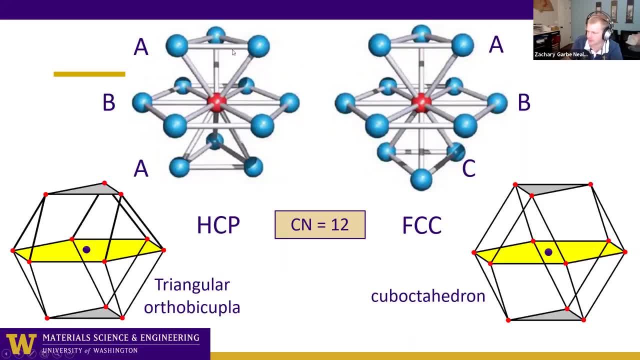 But you do need to know that the coordination is 12. And so this is that visualization of the 12.. And then FCC, because it's ABC, it has a different geometry: cubo-octahedron, And this is important, and I think the mechanical engineers 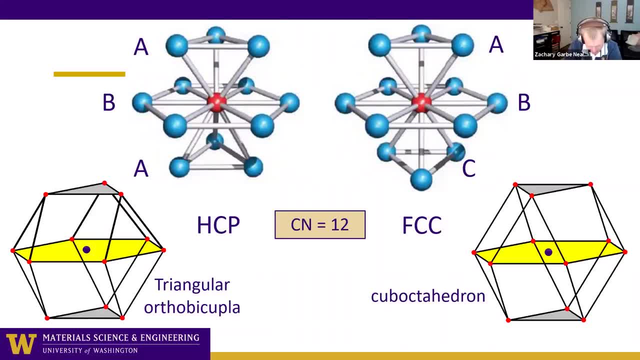 in the group will find this interesting. You know, even though they have the same coordination, the same atomic packing factor, but because the difference in the stacking between HCP and FCC, their mechanics, their mechanical properties, are much different. in general, For metals that are FCC crystal structure, that's aluminum. 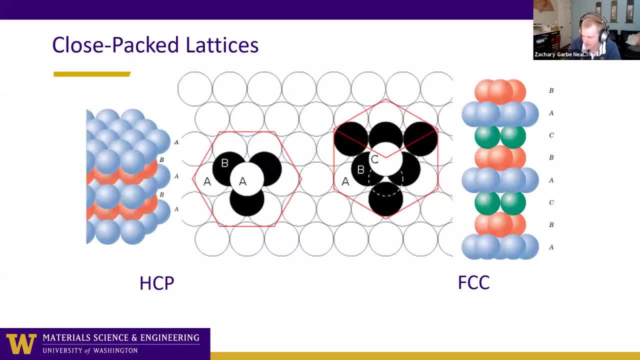 0.74.. Just double-checking. All right, so they have the same packing factor and, like Dr Brush had mentioned, the only difference is the. you know they have these closed-packed planes of atoms and the layering sequence is different, where HCP is ABA and FCC is ABC, And I've tried. 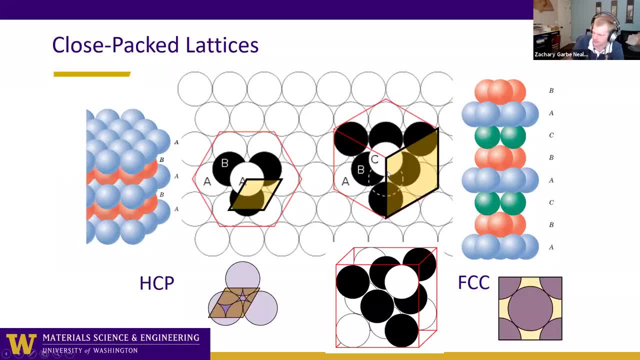 to visualize this further for the FCC so you can try to see where the cubic structure comes from in this orientation. right, So you can see where this is the FCC cube. I've taken just this face and this The two-dimensional projection of that face, and there's the face-centered face of it. okay, And 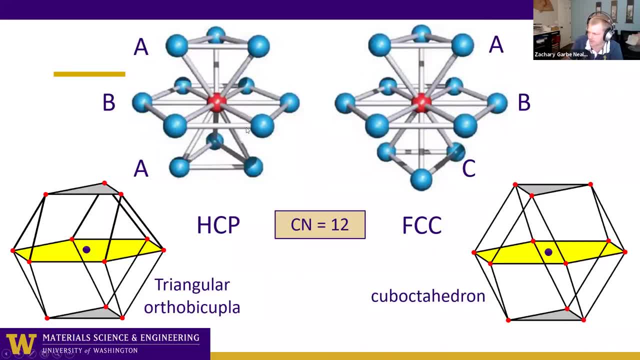 then the coordination is the same for both of them, but what is different is the symmetry of that, the geometry, all right. So for HCP, which is ABA, it has this weird shape: triangular ortho bicouple. You don't need to know the names of anything, but you do need to know that coordination. 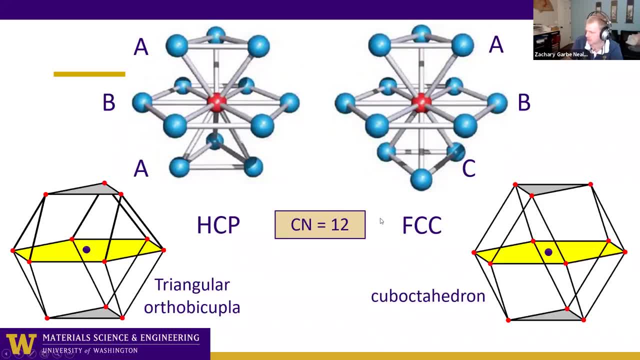 is 12.. And so this is that visualization, And then you have the two-dimensional projection of that 12.. And then FCC, because it's ABC, it has a different geometry: cubo-octahedron, And this is important, and I think the mechanical engineers in the group will find this interesting, You know. 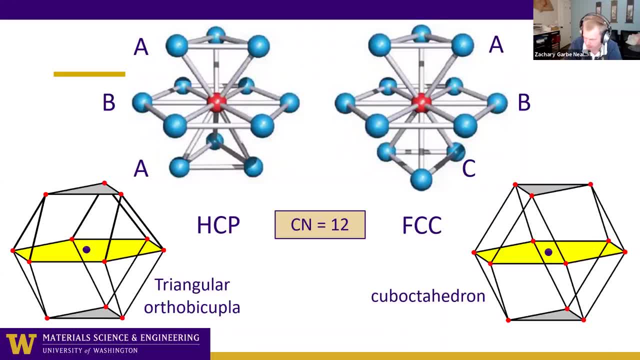 even though they have the same coordination, the same atomic packing factor, but because the difference in the stacking between HCP and FCC, their mechanical properties are much different in general For metals that are: you know they're, you know they're, you know they're. 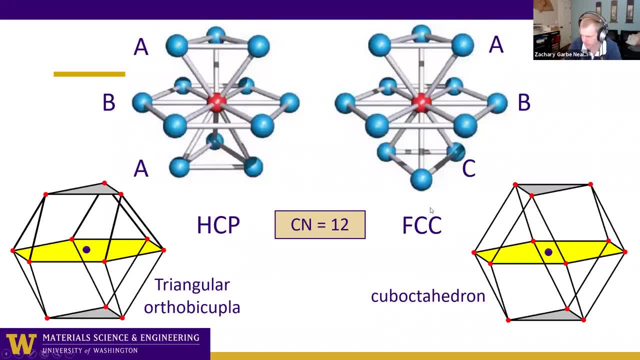 FCC crystal structure that's aluminum, copper, nickel, gold. They are very malleable metals. But metals that are HCP- primarily titanium- are not very malleable. okay, And that's because of the crystal structure. the arrangement of these layers To make a metal malleable means we're. 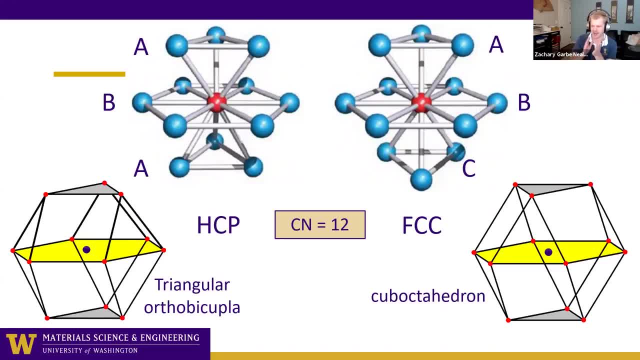 plastically deforming the material. It means we're physically having the atoms slide past each other when we pull a metal apart, all right, And so the crystal structure is not very malleable. The question is, how easy is it for atoms to slide past each other between these two different? 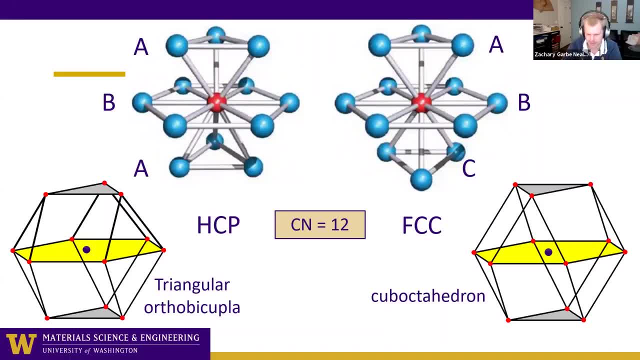 copper, nickel, gold. they are very malleable metals, But metals that are HCP- primarily titanium- are not very malleable. Okay, And that's because of the crystal structure. the arrangement of these layers To make a metal malleable means we're plastically deforming the 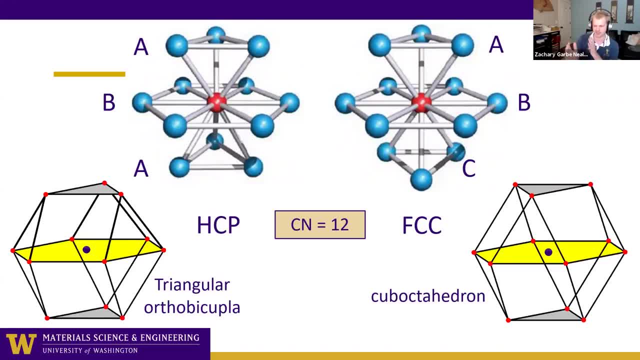 material. it means we're physically having the atoms slide past each other when we pull a metal apart. All right, And so the question is: how easy is it for atoms to slide past each other between these two different crystal structures? And it depends on the number of directions that the plane 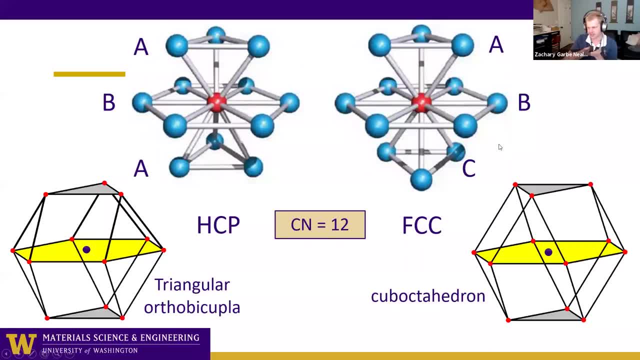 that we're talking about a plane of atom, like an A plane, B plane that can slide, Okay, So I try to visualize this. This is a little bit beyond the scope of the class, although I think we might talk a little bit more about it. 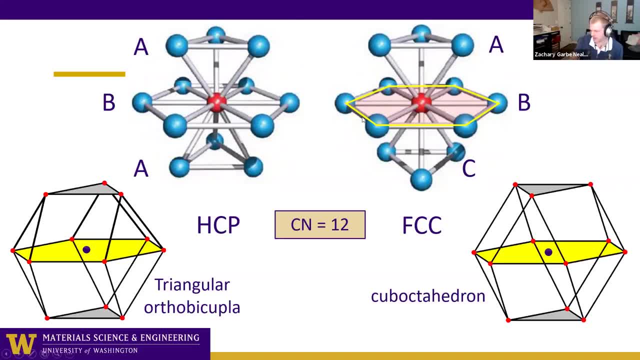 when we discuss mechanical properties. But at this point you don't really need to know. But so I've drawn out a plane of atoms. All right, This is a closed-packed plane For FCC and HCP. they both have these same closed-packed planes. 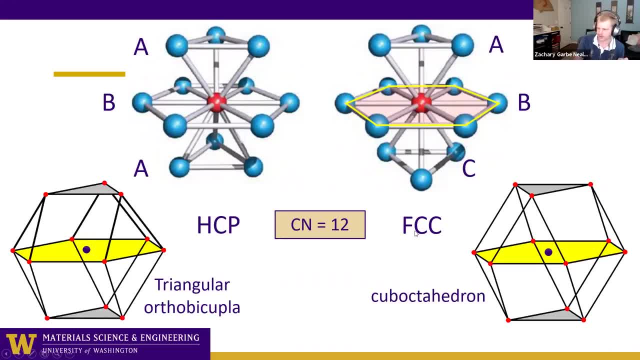 But FCC has more than one of the same closed-packed planes, So I'm going to draw another one here. Here's another plane of closed-packed atoms. Okay, The same shape, the same arrangement of atoms. Where HCP does not have that arrangement, you can't make an. 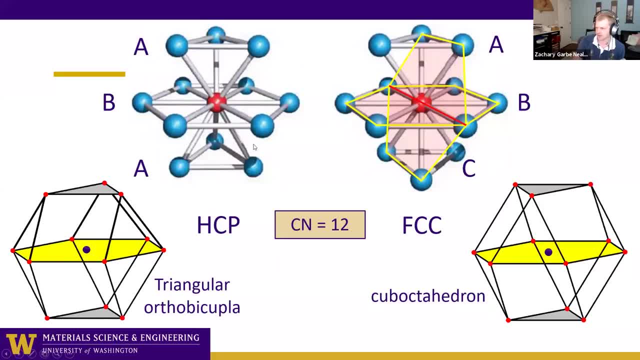 arrangement with another one of these hexagons in this geometry? Okay, And then actually, FCC has two more, So it has a total of four closed-packed planes. Okay, And so later on you'll talk about slip systems. This is, these are the systems of how atoms can slide past each other. 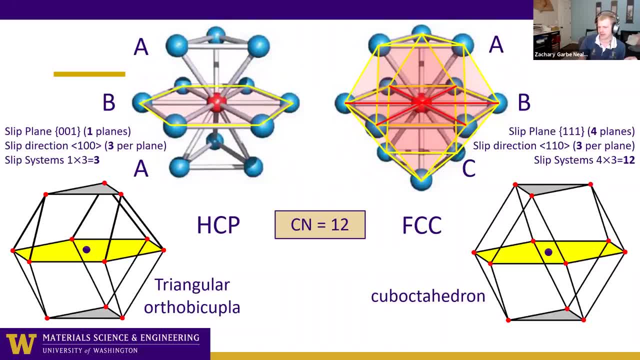 All right, And so FCC has many more slip systems than HCP does. HCP only has three slip systems. FCC has 12.. FCC metals are, in general, are, more malleable than HCP. Okay, All right, Let's move on. 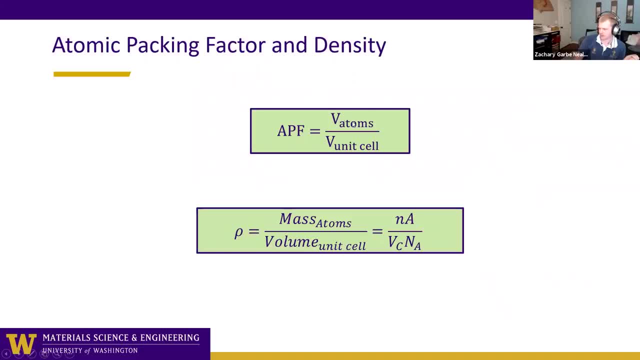 So yeah, the equations to know APF, atomic factor, the volume of the atoms divided by the unit cell. This will also come up the density- I think you've already probably seen it in last homework- is, of course, mass over volume. 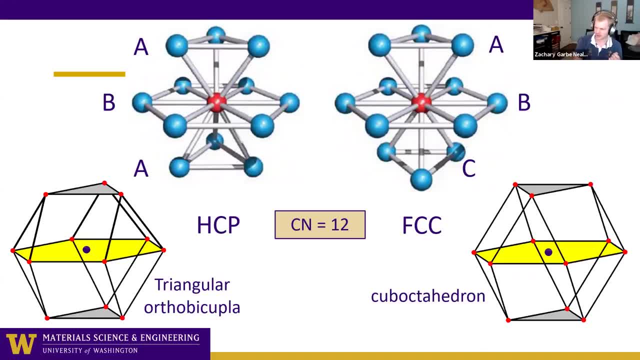 crystal structures And it depends on the number of directions that the plane that we're talking about, a plane of atom, like an A plane, B plane, that can slide okay. So I try to visualize this. This is a little bit beyond the scope of the class, although I think we might talk a little bit more. 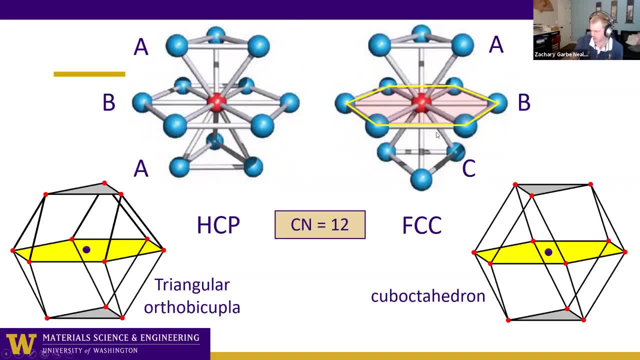 about it when we discuss mechanical properties, But at this point you don't really need to know. So I've drawn out a plane of atoms. all right, This is a closed-packed plane For FCC and HCP. they both have these same closed-packed planes. 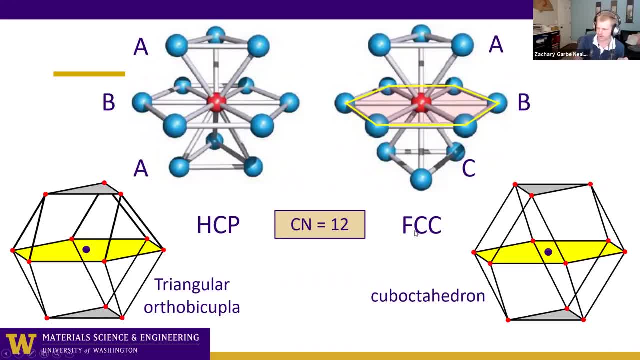 but FCC has more than one of the same closed-packed planes, So I'm going to draw another one here. Here's another plane of closed-packed atoms. okay, The same shape, the same arrangement of atoms. where HCP does not have that arrangement. You can't make another one of these hexagons in this. 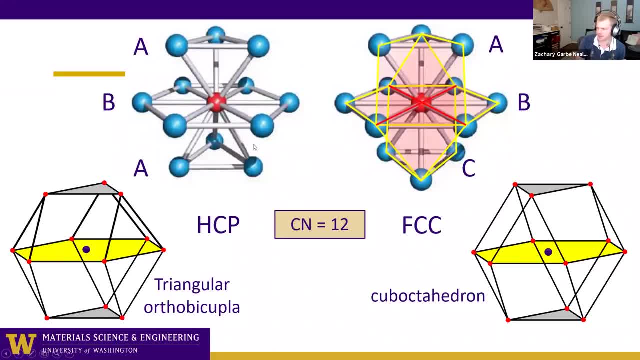 geometry, okay, And then actually FCC has, So it has two more, So it has a total of four closed-packed planes, okay, And so later on you'll talk about slip systems. This is, These are the systems of how atoms can slide past each other. all right. 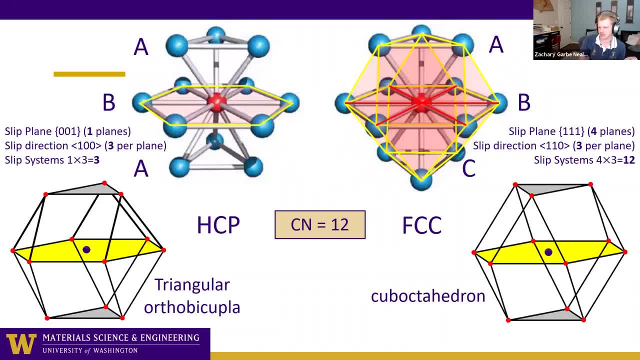 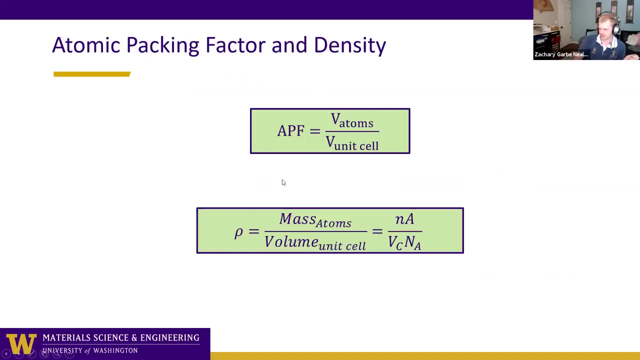 And so FCC has many more slip systems than HCP does. HCP only has three slip systems, FCC has twelve. That's why FCC metals are, in general, are more malleable than HCP. okay, All right, Let's move on. So yeah, the equations to know APF: atomic pack factor, the volume of the atoms divided by the unit cell. 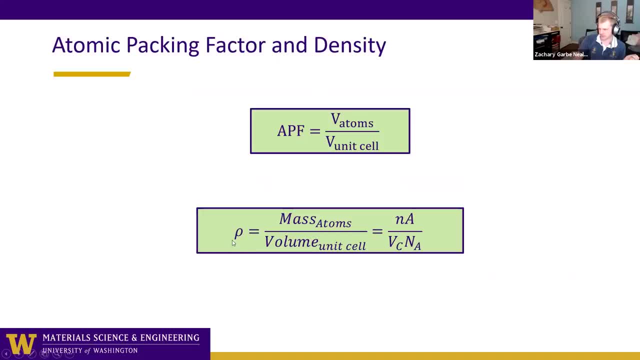 This will also come up. The density- I think you've already probably seen it in last homework- is of course mass over volume. But when you're calculating using the atoms and the crystal structure, you can use this equation here: N is the number of atoms in the unit cell, A is the molar mass of the atom. 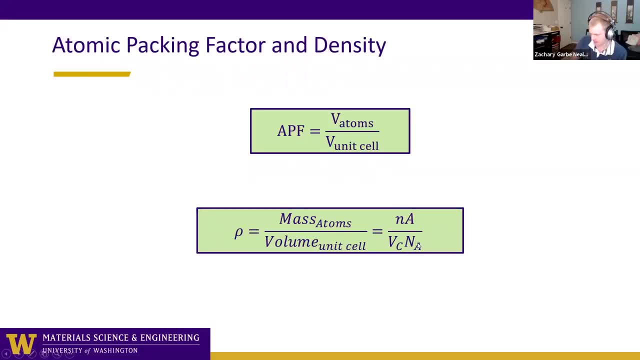 Or atomic mass of the atom. N is Avogadro's number, VC is the volume of the unit cell. Okay, So as long as you know those parameters like the A and R, then you should be able to calculate density if you're given molar mass, And you should also know the number of atoms in the molar unit cell. 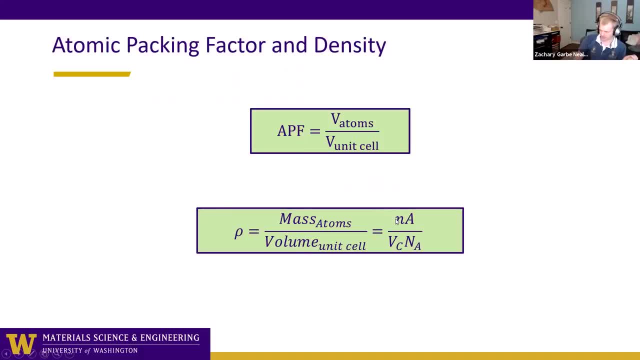 But when you're calculating using the atoms and the crystal structure, you can use this equation here. Here we go. This is the number. N is the number of atoms in the unit cell. A is the molar mass of the atom, Or atomic mass of the atom. 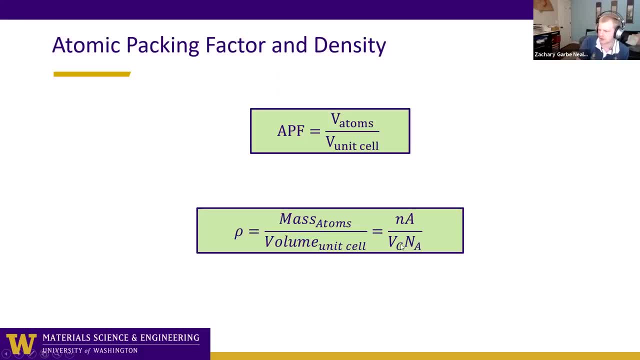 N is Avogadro's number, VC is the volume of the unit cell. Okay, So as long as you know those parameters like the a and r, then you you should be able to calculate density if you're given a molar mass. 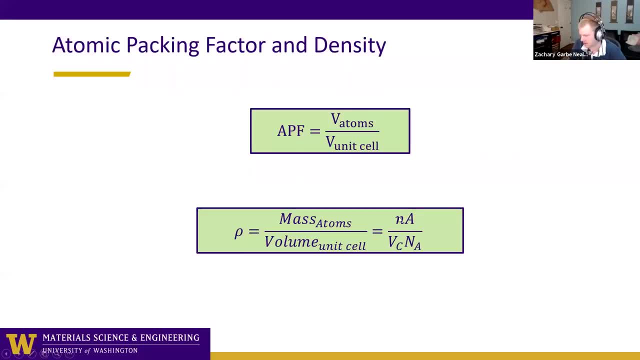 And you should also know the number of atoms in the molar unit cell, atoms in the unit cell. So we calculated that for FCC it was four atoms, BCC it was two atoms, and so on. A is the molar mass, so it's going to be in grams per mole. N sub A is just Avogadro's. 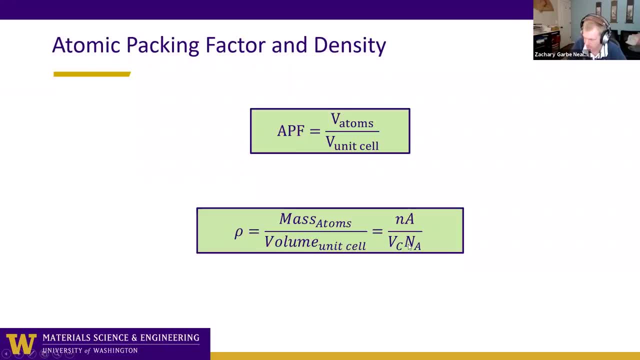 number. What is that? 6.022 times 10 to 23.. What is that? Atoms per molecule, just atoms, right Per mole? atoms per mole. excuse me, So then that will cancel out the moles and you're left with 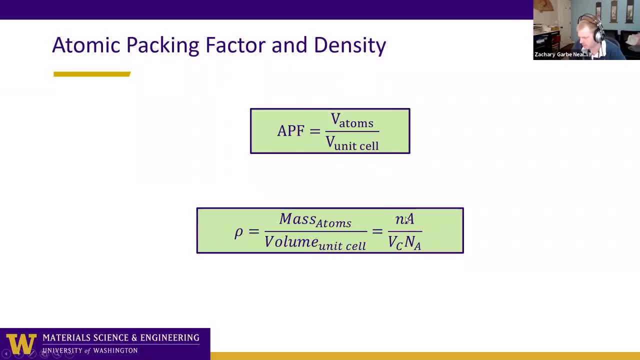 grams per atom times. the number of atoms divided by VC is the volume of the unit cell. So you're left with, you know, the mass of the atoms in the unit cell divided by the volume of the unit cell, and that's density. Okay, so we're going to move on and talk about some symmetry of crystal. 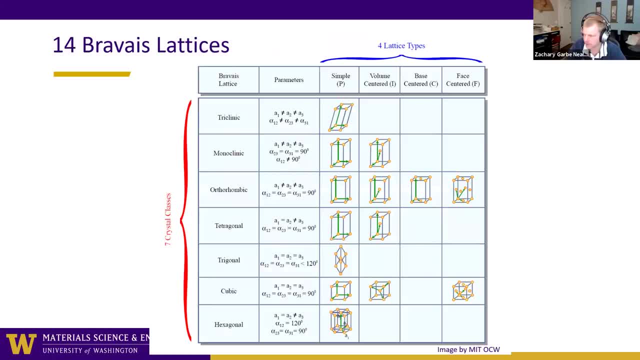 structures- and Dr Brush had briefly mentioned this, the Bravais lattices. So, like he said, all crystals can be arranged or categorized into one of these 14 Bravais lattices. okay, And so the ones that we typically deal with are the cubic system, because the symmetry is easy. 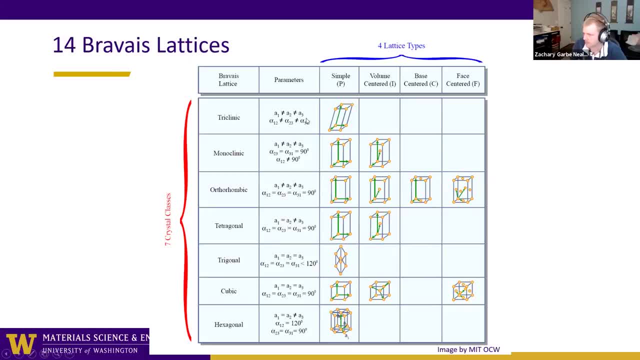 mathematically it's easy to work with. But again, there's different lattice types and these are just lattices. okay, These are not crystal structures. Lattices are just a set of points In space. It doesn't mean where the- I mean atoms- can be put onto these lattice points or a. 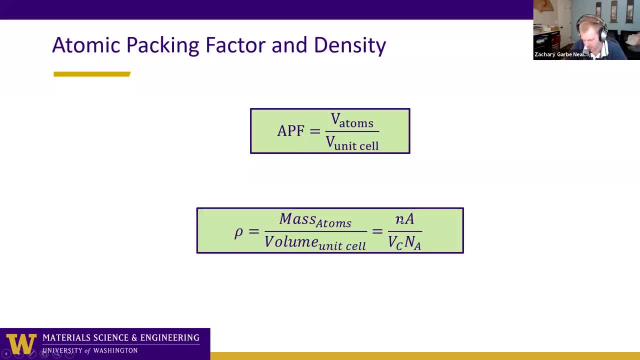 N is the number of atoms in the unit cell. So we calculate that for FCC it was four atoms, BCC it was two atoms, and so on. A is the number of atoms in the unit cell, BCC is the number of atoms, BEC is two atoms�. So that likes to point out that other kinds of things areч. 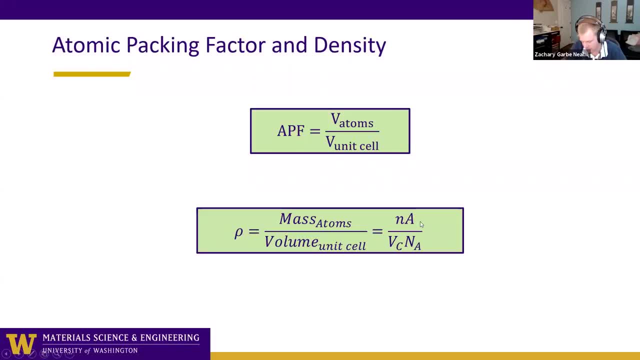 A and F is the number of atoms in the unit cells, So that likes to point out that other kinds of things arech is the molar mass, So it's going to be in grams per mole. Okay, N sub A is just Avogadro's number. 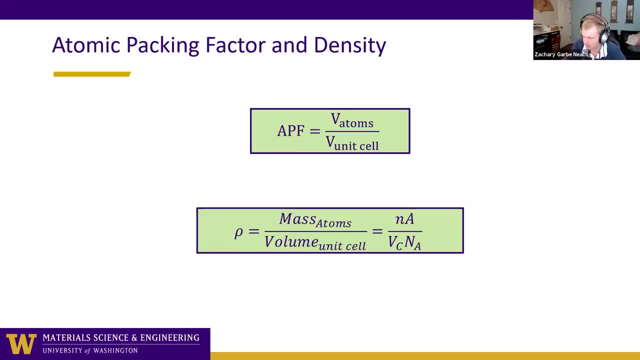 What was that? 6.022 times 10 to 23.. What is that? Atoms per molecule, just atoms right Per mole? atoms per mole, excuse me? So then that will cancel out the moles and you're left with. 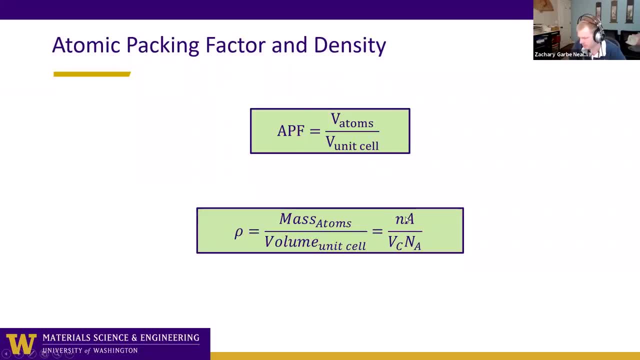 grams per atom times. the number of atoms divided by VC is the volume of the unit cell. So you're left with, you know, the mass of the atoms in the unit cell divided by the volume of the unit cell, And that's density. Okay, So we're going to move on and talk about some symmetry of crystal. 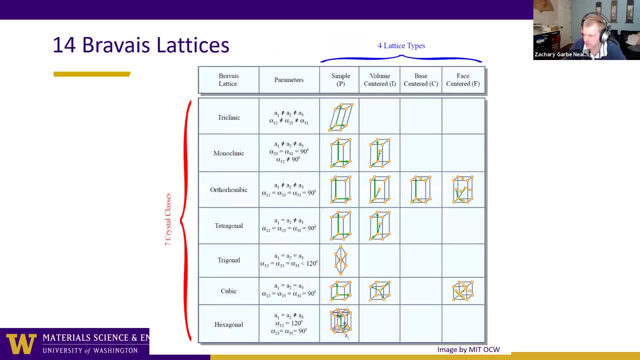 structures, And Dr Brush had briefly mentioned this, the Bravais lattices. So, like he said, all crystals can be arranged or categorized into one of these 14 Bravais lattices. Okay, And so the ones that we typically deal with is are the cubic system, because the symmetry is. 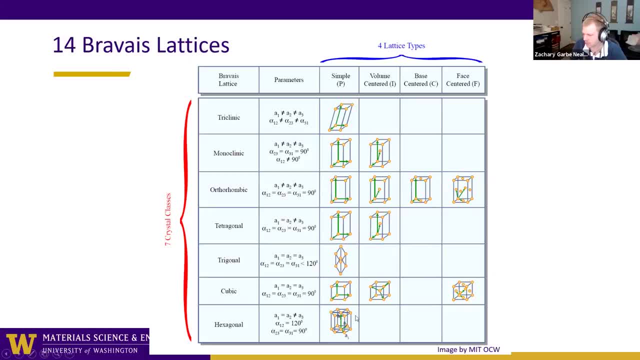 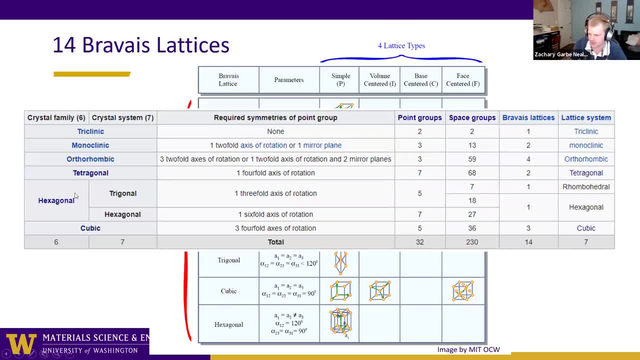 it's. And then there's a bit of complexity, you know, especially in the hexagon. So I just screen clip this from Wikipedia: If you look up like crystal structure or something you know between hexagonal, the crystal family system and the lattice system and and trigonal hexagonal, 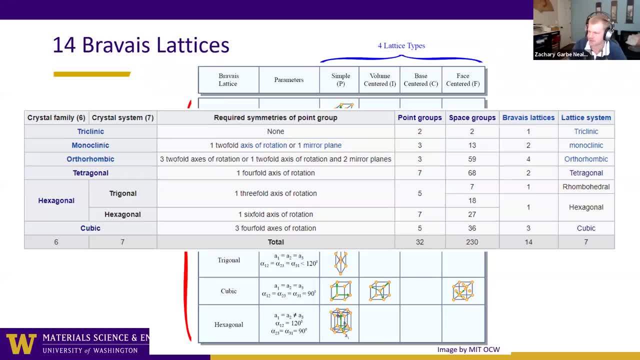 group of atoms can be put onto these lattice points. And then there's a bit of complexity, you know, especially in the hexagon. So I just screen clipped this from Wikipedia: if you look up like crystal structure or something you know, between hexagonal, the crystal family system, 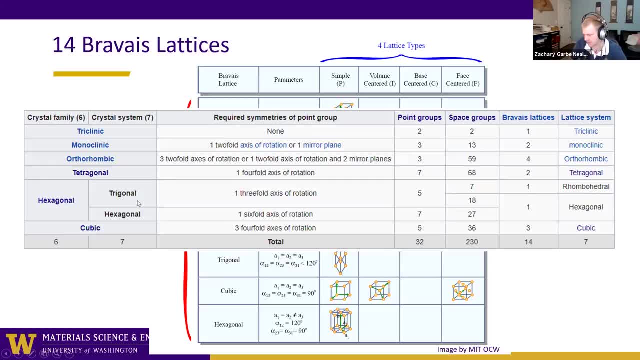 and the lattice system and trigonal hexagonal. It's not. you know, you don't need to know, it's not too important. We'll talk a little bit when we start looking at hexagonal, closed-packed, and which system is it in? 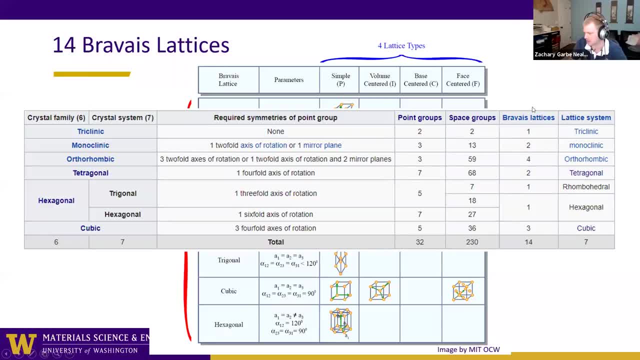 But what this is showing is the Bravais lattice and it's just a way to categorize the symmetries of these crystals. In a graduate level courses we talk about space group symmetries, which are just further ways of defining the symmetry of the the different crystals and so on. 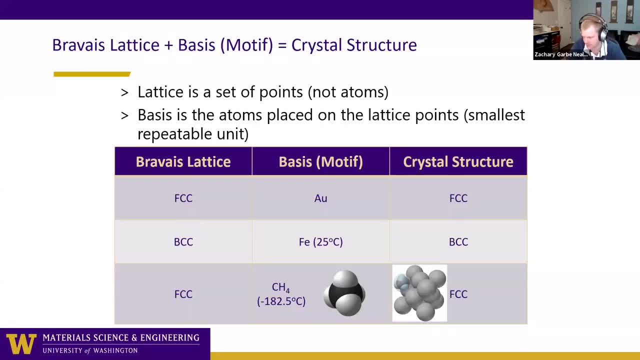 lot of students miss this and even I've even had some professors that have incorrectly said this. but I want to emphasize that the crystal structure is made up of the lattice plus a basis and something this oftentimes this is also called the motif, so I use these interchangeably, motif and basis. so the 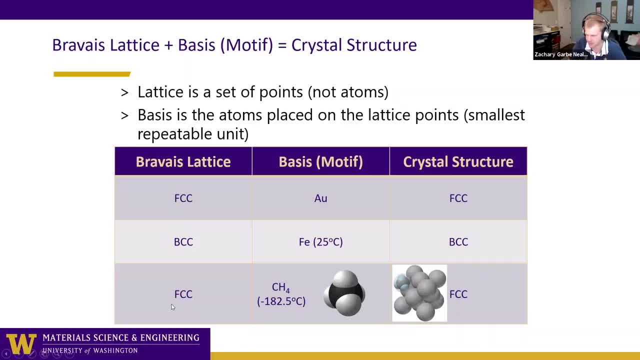 lattice, like I said, is just a group of points in space. it doesn't represent, you know, the crystal structure. physically it's just a group of points. so FCC is a lattice, it's a Bravais lattice and, for example, gold, the metal, has the FCC crystal structure. so in this case the lattice and crystal structure have the 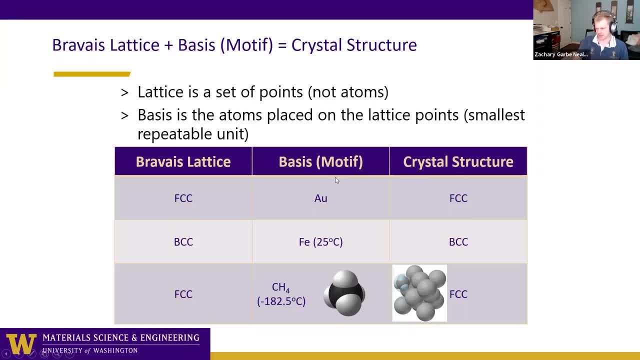 same name. okay, but it's not the same. it's not necessary for other crystals. here's another example: BCC of iron has a BCC crystal structure, and then inert gases. this is methane and other noble gases if you cool it down to solidified. and then inert gases. this is methane and other noble gases if you cool it down to solidified. 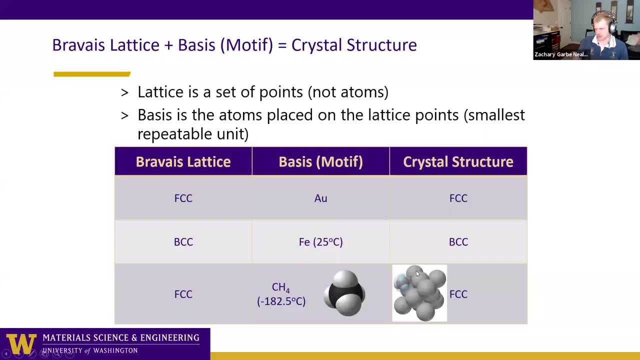 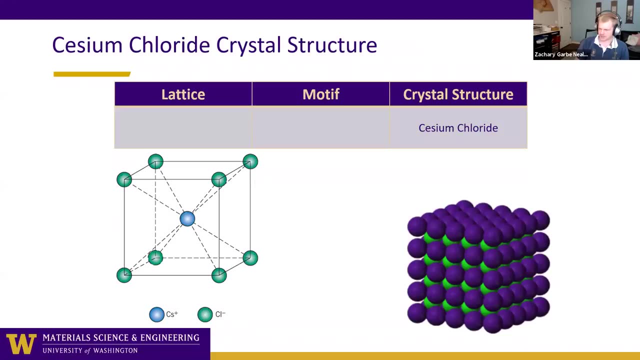 them generally form in the FCC crystal structure. so in this case the basis is a group of atoms, it's a, it's a molecule, and if you cool it down enough, it forms the FCC crystal structure. but then it can get more complex. so here's an example. this is the cesium chloride crystal structure. so what do you think? 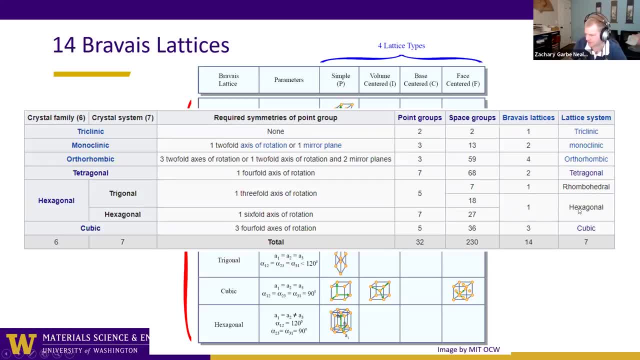 it's not. you know, you don't need to know, It's not too important, but we'll talk a little bit when we start looking at hexagonal closed pact in which system it's in. But what this is showing is the Bravais lattice And it's just a way to categorize the symmetries of these crystals. 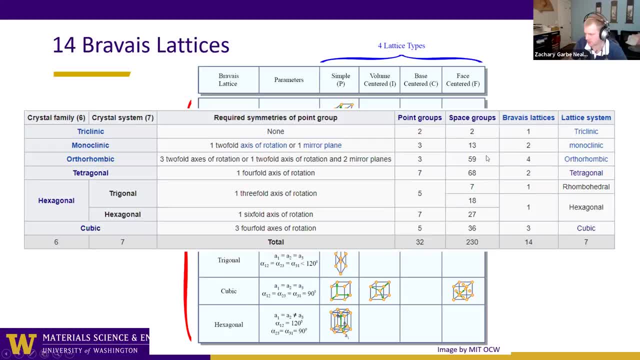 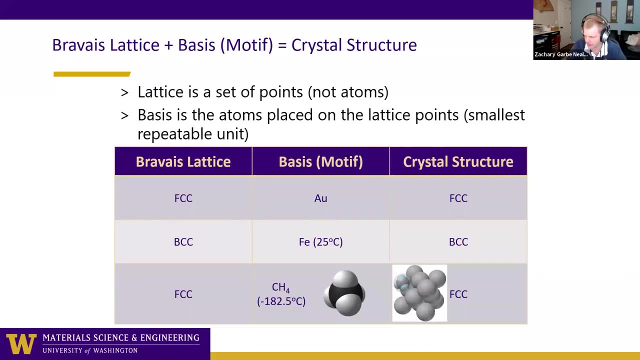 In a graduate level courses, we talk about space group symmetries, which are just further ways of defining the symmetry of the, the different crystals and so on, And so what I want to emphasize- and a lot of students miss this, and even I've- I've even had some professors that have 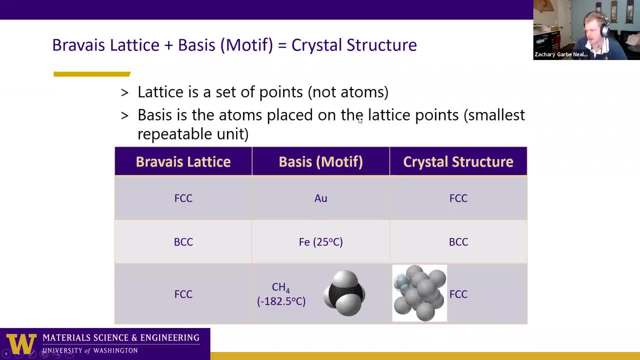 have incorrectly said this, But I want to emphasize that the crystal structure is made up of the lattice plus a basis, And so this, oftentimes this is also called the motif. So I use these interchangeably, motif and basis. So the lattice, like I said, is just a group of points in space. It doesn't represent. 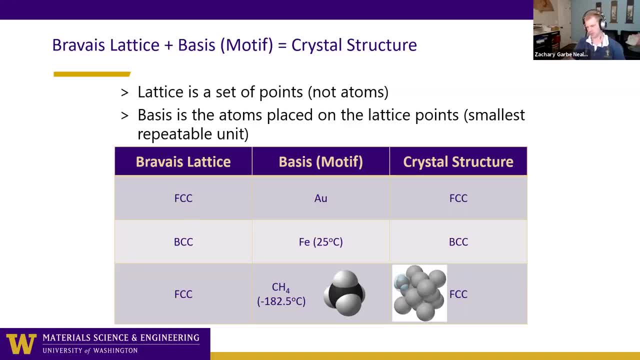 you know the crystal structure. physically It's just a group of points. So FCC is a lattice, It's a Bravais lattice And, for example, gold, the metal, has the FCC crystal structure. So in this case the lattice and crystal structure have the same name. 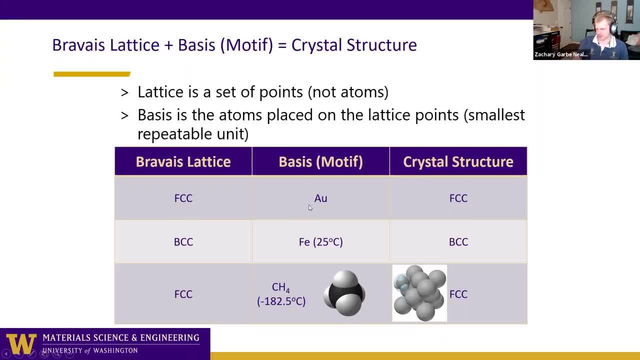 Okay, but it's not the same. it's not necessary for other crystals. Here's another example: BCC of iron has a BCC crystal structure, and then inert gases. this is methane and other noble gases if you cool it down to solidify them. 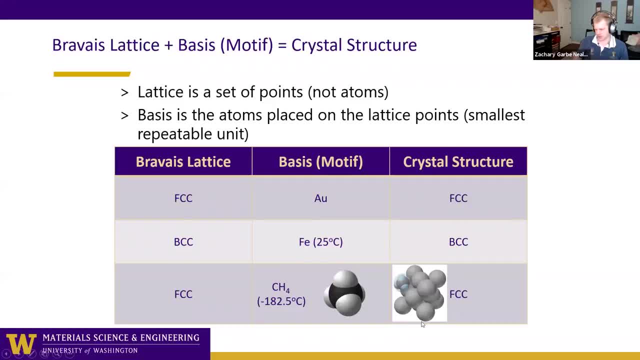 generally form in the FCC crystal structure. So in this case the basis is a group of atoms, it's a molecule, and if you cool it down enough it forms the FCC crystal structure. But then it can get more complex. so here's an example. 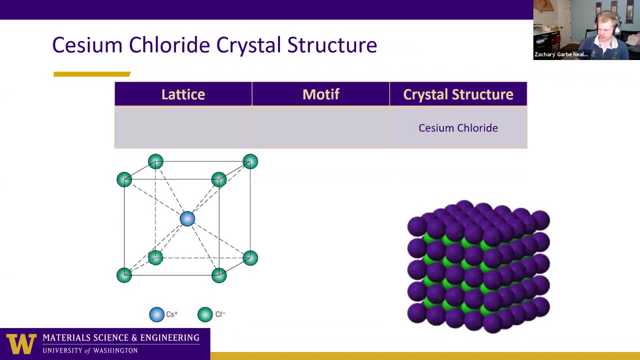 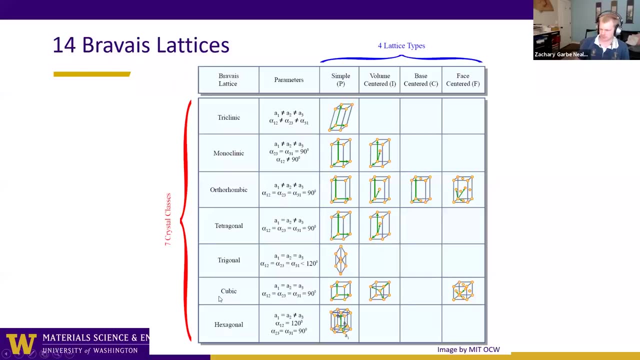 This is the cesium chloride crystal structure. So what do you think the base? excuse me, what do you think the lattice is of this crystal structure? What is the lattice? And specifically, what is the Bravais lattice right? So it's going to be one of these cubic. 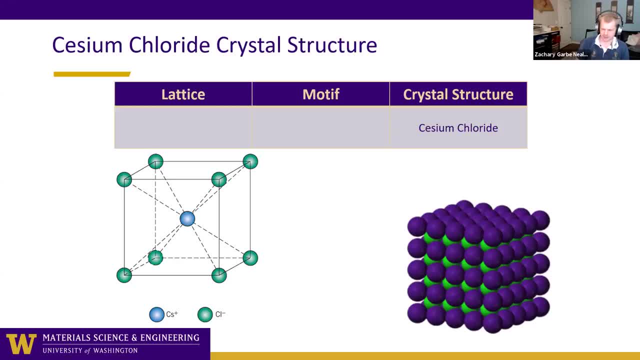 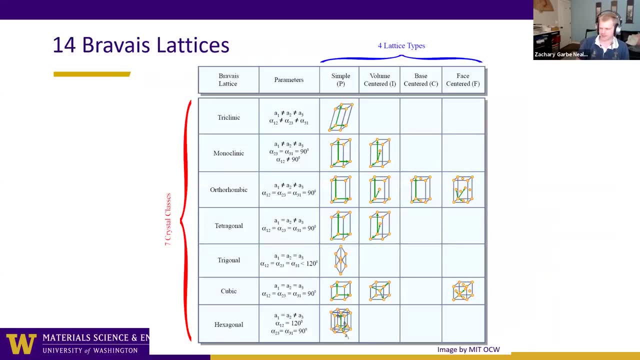 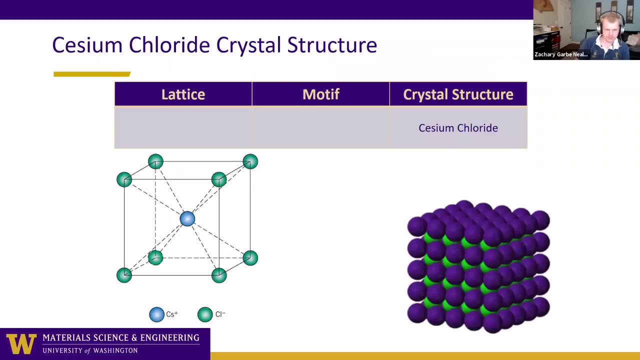 the base. excuse me, what do you think the lattice is of this crystal structure? what is the lattice? you know specifically what is the lattice and what is the Bravais lattice, right? so it's going to be one of these cubic saying BCC, because it's incorrect and this is the point I'm trying to make. the 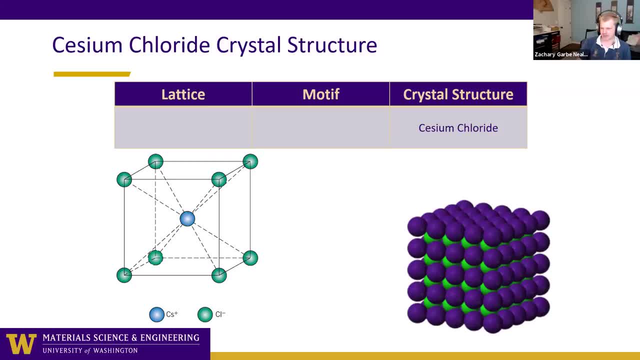 lattice in for this crystal structure is not BCC, it's actually simple cubic. okay, so I have drawn this out. the motif is cesium chloride. it's a group of two atoms. okay, so that's the motif. that's the motif. that's the group of atoms, okay. 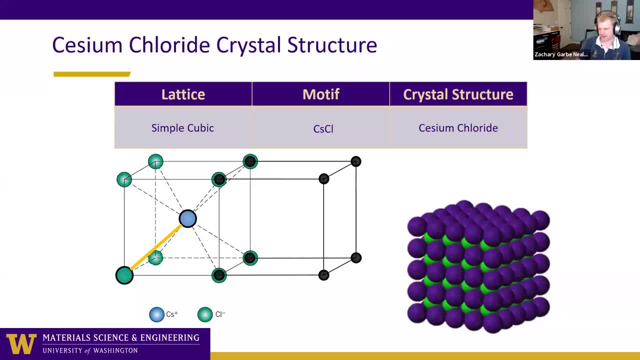 so theangelic, and this is the motif that we're going to draw on- it's a single lattice and the lattice point is just in the middle of the hexagon. I drew that line to give you an idea of what a just say: oh this is BCC. No, it's not BCC. BCC would be if the atom in the center is the same. 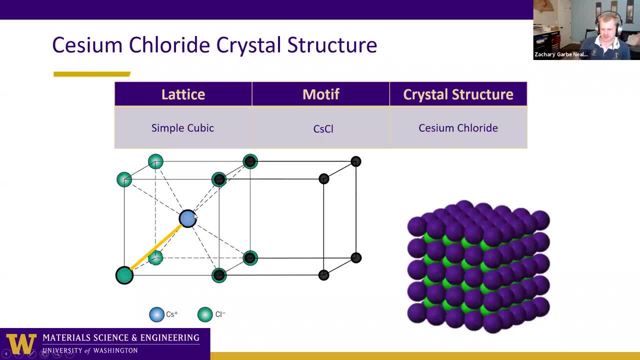 as the atoms at these lattice points, But the atom in the center is not the same. The lattice structure is simple, cubic. The Bravais lattice is simple cubic. It has a motif of two atoms. So if you translate this motif to all of these different lattice points, that's how you. 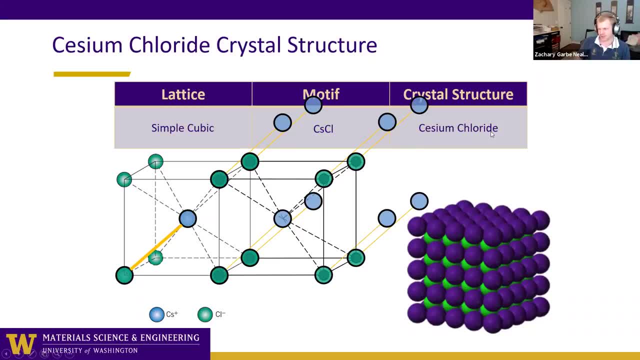 build up the crystal, And the crystal structure is called cesium chloride. It's other like cesium bromide, cesium iodide. I think they all make the cesium chloride crystal structure. So does that make sense? Why does the central atom not count? So in BCC I should have included this. I had a 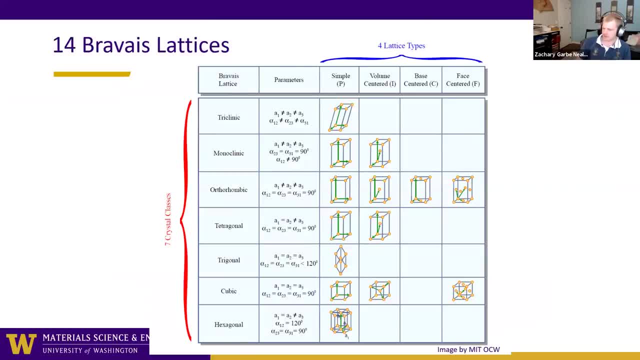 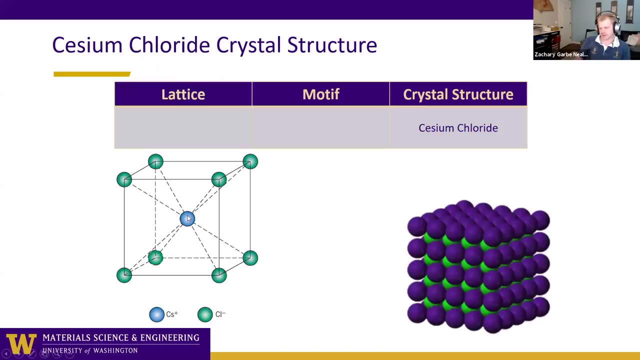 picture of what it would look like if it was BCC. In BCC all the atoms are the same, Like iron is BCC. Okay, But in this case the atom in the center is not the same as the atom on the. 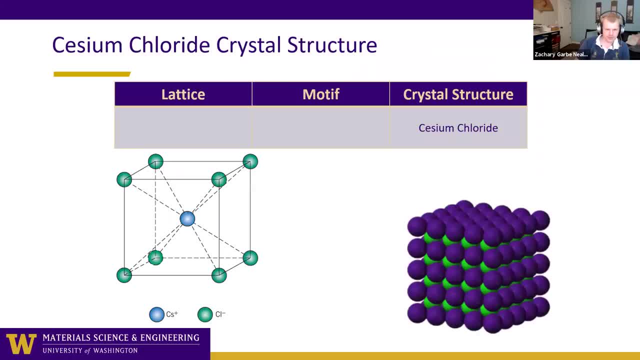 lattice points. okay, So it has these two points. see these two points here. They're going to be in the smooth كل Ober Kang BCC, because it's incorrect, And this is the point I'm trying to make. The lattice in for this crystal structure is: 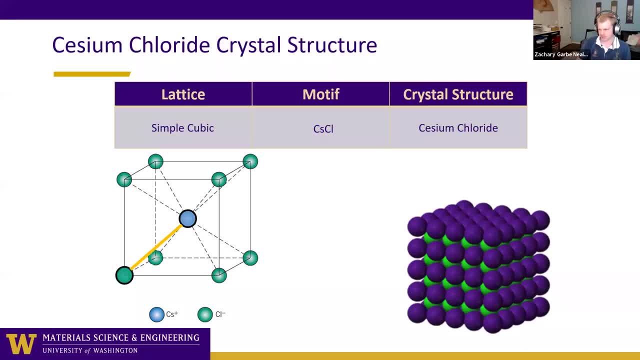 not BCC, it's actually simple cubic, okay. So I've drawn this out. the motif is caesium chloride, it's a group of two atoms, okay, So that's the motif there. There's the simple cubic lattice points, okay. So if you could to the matrix, will you count these three points? 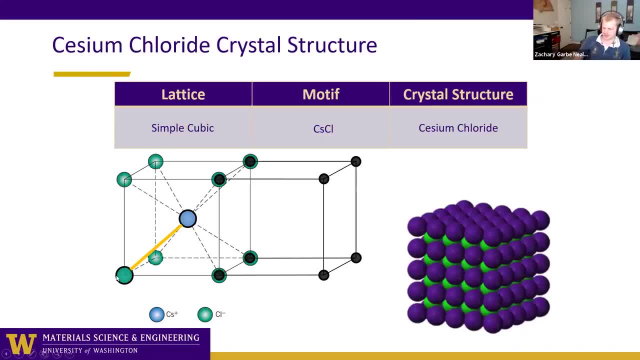 Okay, you were to take this motif. let's take this chlorine ion with the cesium attached. you move, you translate it to each one of these lattice points. That's how you expand to this cesium chloride crystal structure. So the crystal structure is not BCC. That's what I've heard. 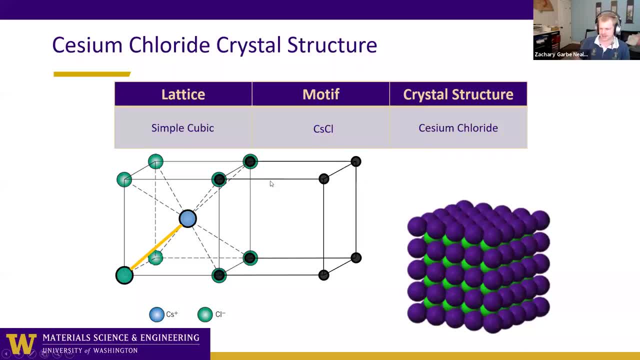 I've heard some professors say: oh, this is BCC. No, it's not BCC. BCC would be if the atom in the center is the same as the atoms at these lattice points. But the atom in the center is not the same. 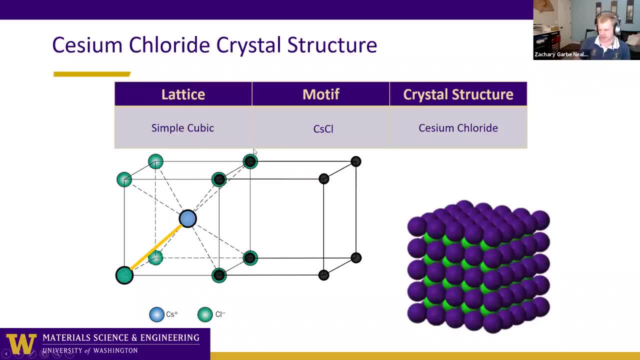 The lattice structure is simple cubic. The Bravais lattice is simple cubic. It has a motif of two atoms. So if you translate this motif to all of these different lattice points, that's how you build up the crystal. And the crystal structure is called cesium chloride. It's the other. 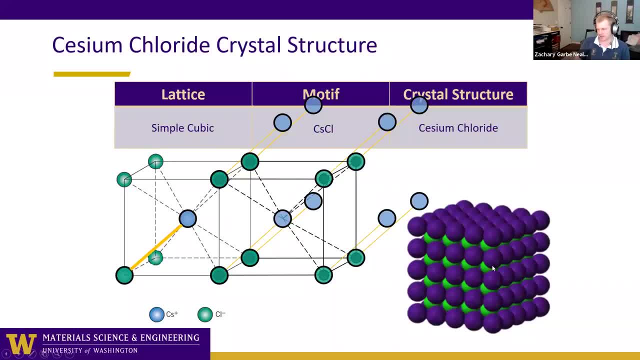 like cesium bromide, cesium iodide- I think they all make the cesium chloride crystal structure. So does that make sense? Why does the central atom not count? So in BCC I should have included this. I had a picture of what it would look like if it. 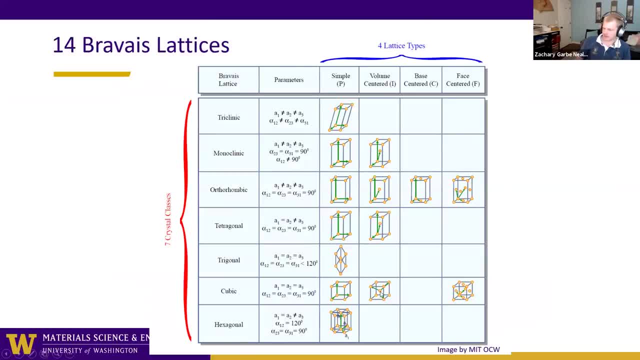 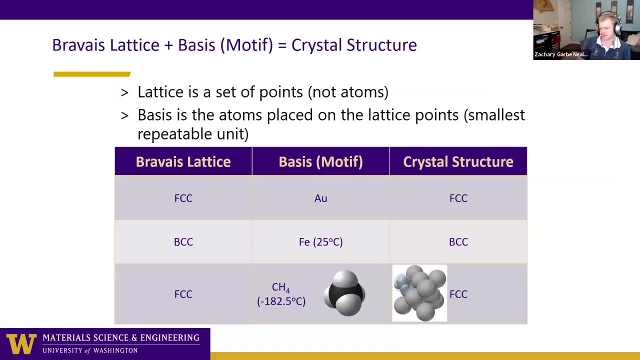 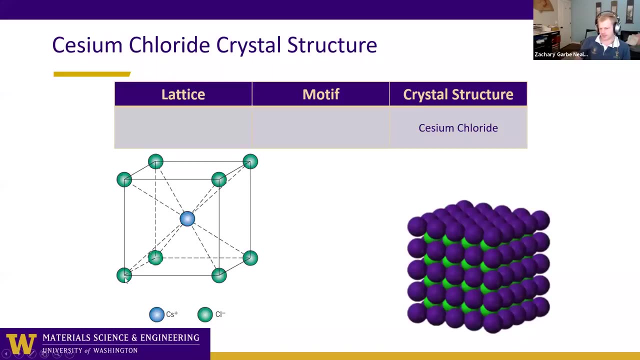 was BCC. In BCC all the atoms are the same, Like iron is BCC, But in this case the atom in the center is not the same as the atom on the corner. So if you translate this motif to all of these, 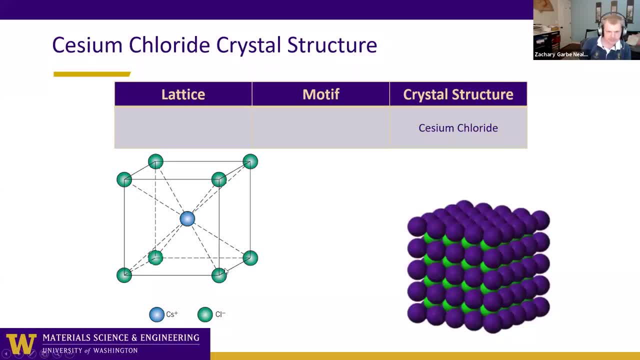 lattice points. it's the same as the atom on the corner. Yeah, it's simple cubic of cesium chloride, like of the cesium chloride molecule. I guess you could say All right. So this is why I wanted to emphasize that this is not the BCC structure. 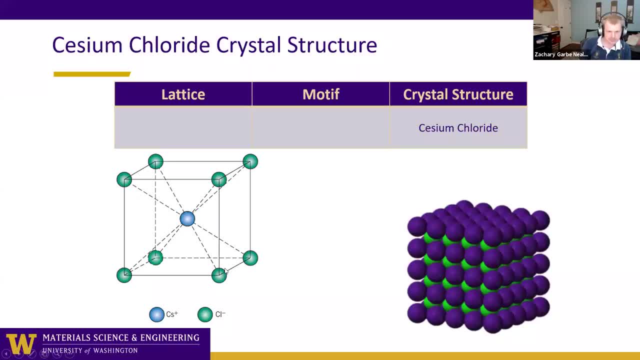 corner. Yeah, it's simple cubic of cesium chloride, like of the cesium chloride molecule. I guess you could say: All right. So this is what I wanted to emphasize: That this is not the BCC structure, And I have some more examples that should make it clear. So here are a set of 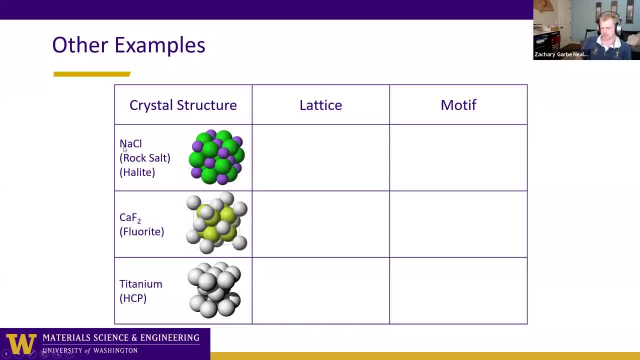 different crystal structures and their respective names. So sodium chloride is called the rock salt crystal structure. It's also called the halite crystal structure. It's the same thing. So what is the lattice? What is the Bravais lattice for sodium chloride? What do you guys think? 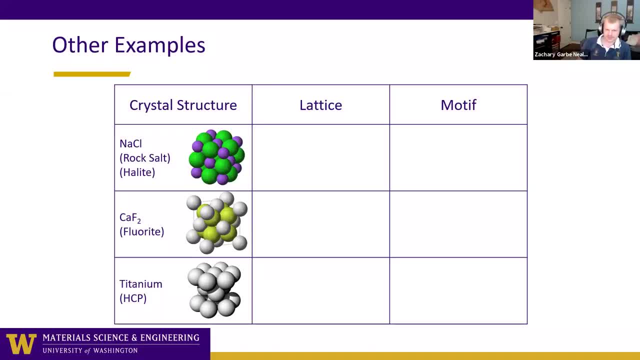 All right, it's not BCC this time. This time it's FCC. Yeah, And the motif? what do you think the motif is for FCC? And you can see here, you know, just look at these blue atoms, Right blue. which atom is the blue atom? It is a smaller, so it's going to be the cation. Typically, cations are: 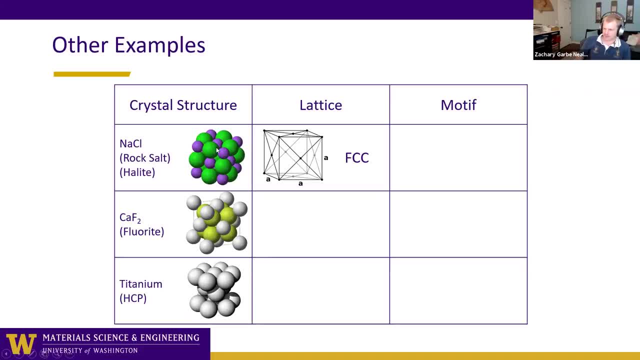 smaller right, We're giving away like electrons. So so you see, the sodium chloride, It's, it's in the background, makes this FCC lattice here. So what is the basis? Yeah, so sodium chloride is right, two atoms, So sodium chloride is the basis. So if you took this sodium 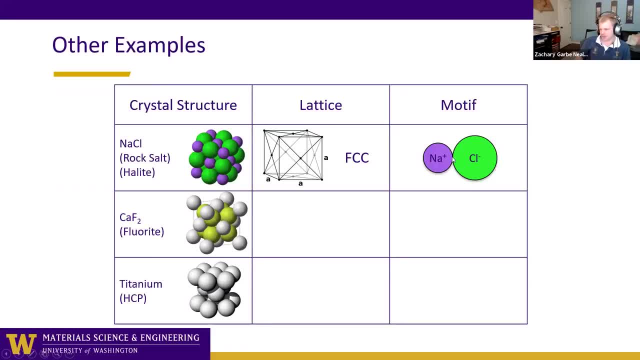 attached to this chlorine. even if you just took the middle or the center of mass and you put it at each one of these lattice points, you're going to construct the sodium chloride crystal structure. Okay, how about calcium fluoride or fluoride crystal structure? What's the lattice? 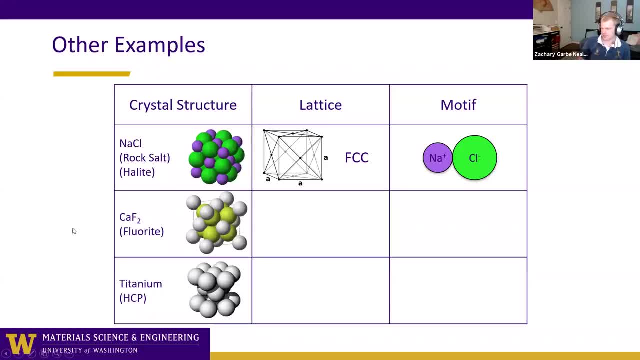 Yeah, this one's also FCC. and how about the basis for this one? Yes, so this one is as you see. here's the FCC lattice, right here. what is this? the calcium makes that FCC structure. All right, I'm going to move on. The motif for this is just a group of three atoms: calcium and 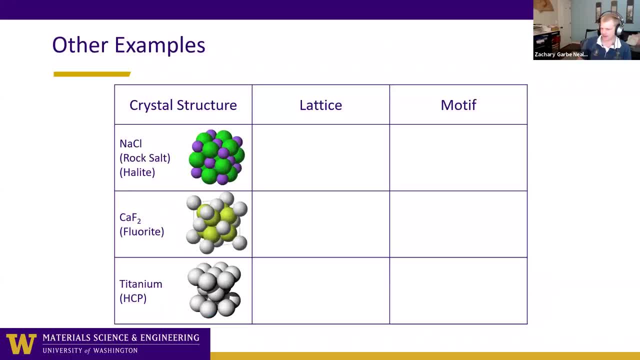 And I have some more examples that should make it clear. So here are a set of different crystal structures And I'm going to show you a few of them. So here are a set of different crystal structures And I'm going to show you a few of them. So here are a set of different crystal structures And I'm 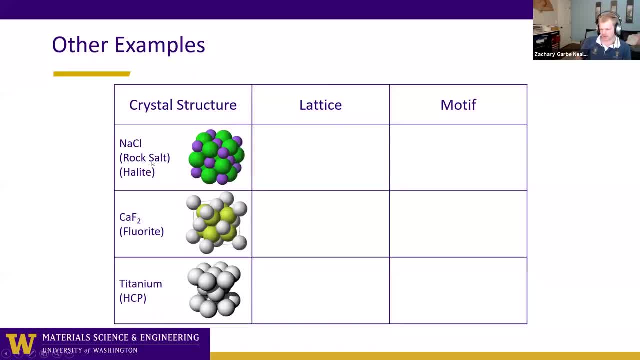 and their respective names. So sodium chloride is called the rock-salt crystal structure. It's also called the halite crystal structure- the same thing. So what is the lattice? What is the Bravais lattice for sodium chloride? What do you guys think? 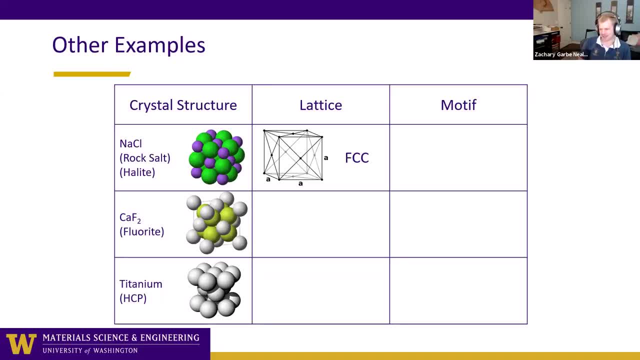 All right, it's not BCC this time. This time it's FCC. yeah, And the motif? what do you think the motif is for FCC? And you can see it here. just look at these blue atoms. Which atom is the blue atom? 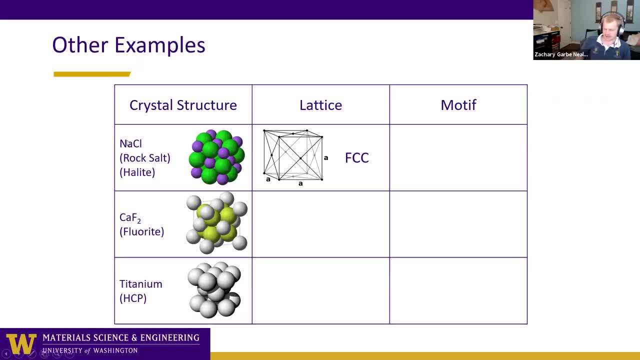 It is smaller. so it's gonna be the cation. Typically, cations are smaller. right, We're giving away electrons. So you see, the sodium makes this FCC lattice here. So what is the basis? Yeah, so sodium chloride is right, two atoms. 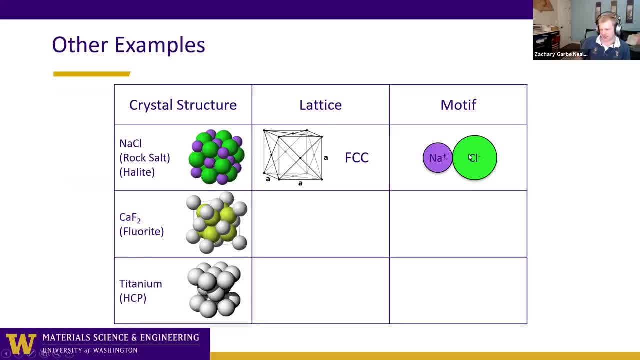 So sodium chloride is the basis. So if you took this sodium attached to this chlorine, even if you just took the middle or the center of mass and you put it at each one of these lattice points, you're gonna construct the sodium chloride crystal structure. 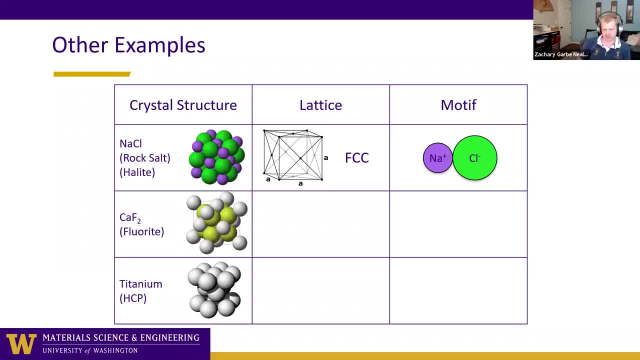 Okay, how about calcium fluoride or fluoride crystal structure? What's the lattice? Yeah, this one's also FCC. And how about the basis for this one? Yeah, so this one was. you see, you know, here's the FCC lattice, right here. 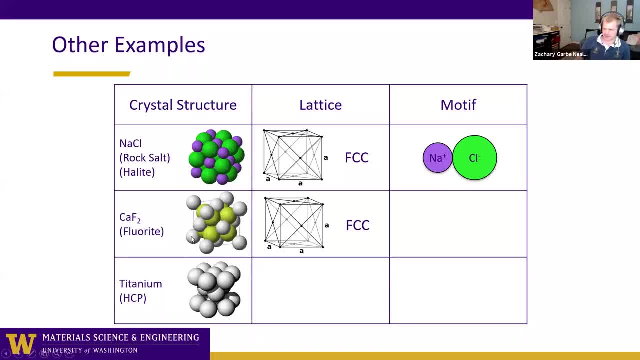 The. what is this? The calcium makes that FCC structure. The calcium makes that FCC structure. All right, I'm gonna move on. The motif for this is just a group of three atoms: calcium and two fluorines. So if you were to take calcium and two fluorines, 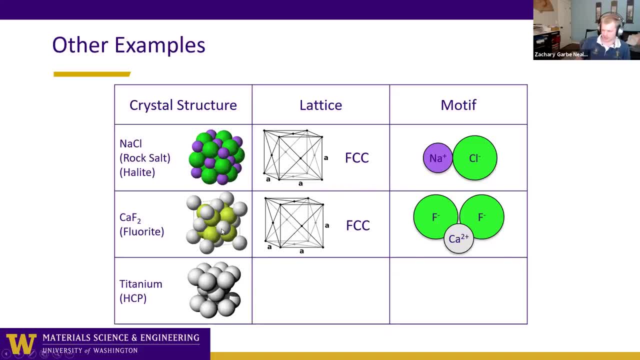 two fluorines. So if you were to take calcium and two fluorines and translated it to every lattice point in the FCC, you're going to make the fluorite structure. So if you took, say, these three atoms right here, calcium and two fluorines, you translate this over to the next. 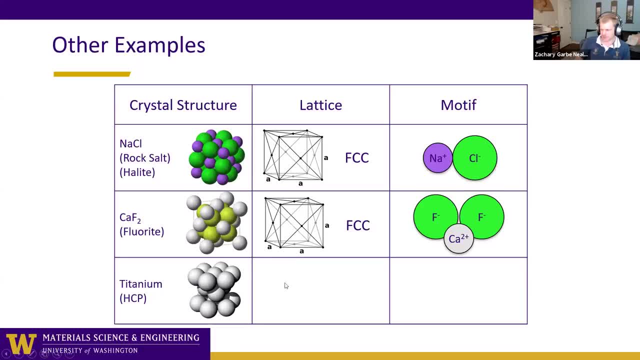 one. you're going to build up the symmetry And there shouldn't be any overlapping When you translate it. there's no duplicates, That wouldn't work, They're all unique. Okay, now we get to titanium, the HCP. So I want to emphasize this as well, because a lot of students get this incorrect. 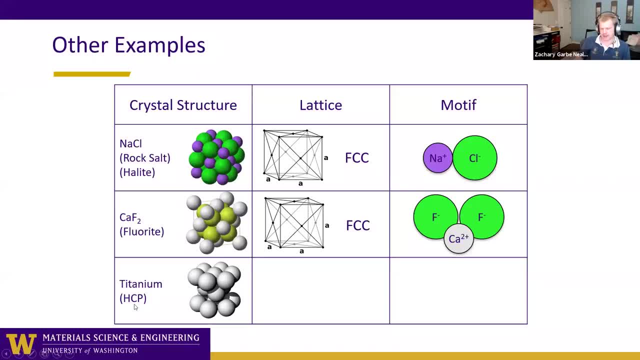 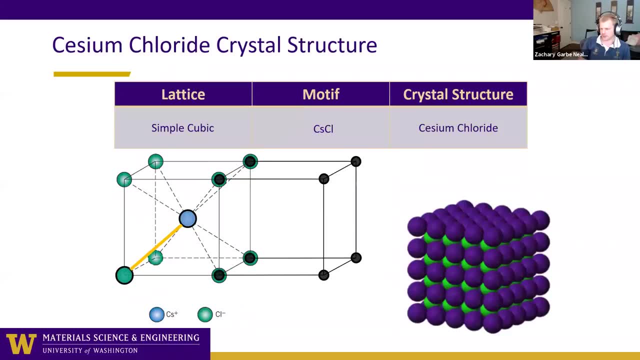 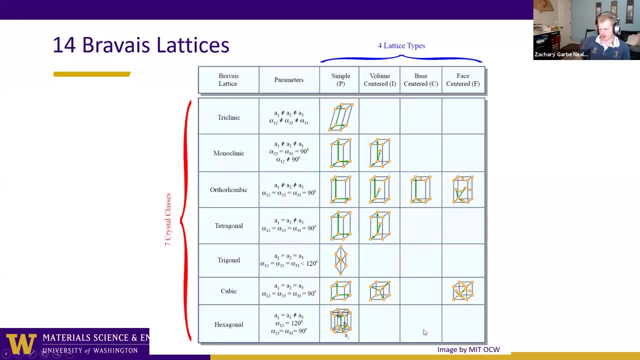 HCP is a crystal structure, It is not a Bravais lattice. Okay, if you go back to the Bravais lattices and this will give away the next answer: hexagonal doesn't have face center, doesn't have body center. All right, there's only simple: hexagonal is the only Bravais lattice for. 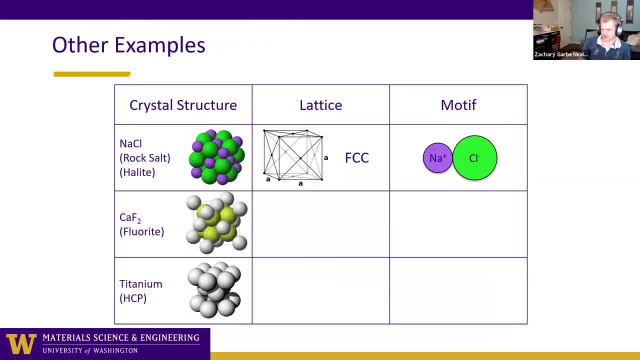 hexagonal, So the crystal structure is HCP. What is the lattice? I already gave away It's hexagonal. Tief is actually two titanium atoms. Okay, so that's the point I want to make: that lattice points and crystal structure are different. Okay, they're not the same. Lattice is just a set of. 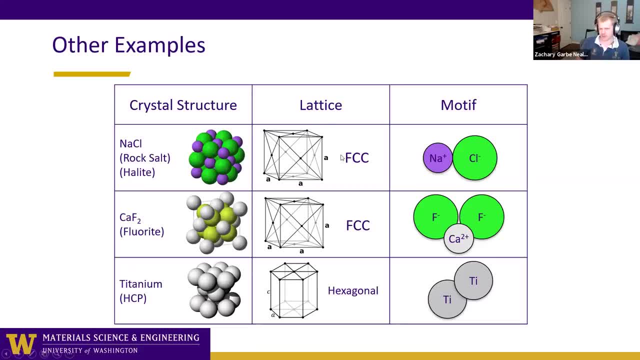 points in space and depends on what you put onto those points in space And that can build up and that's how we get so many different types of crystal structures, not just 14. There's way more than 14 crystal structures, but there's only 14- Bravais, lattices, Okay, yeah, simple, hexagonal. 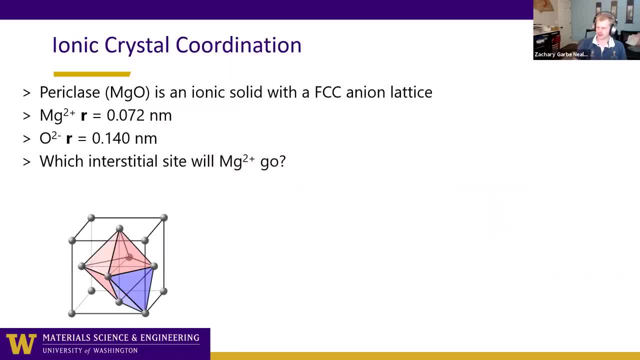 Let's move on. So here's a question, And I don't. I don't remember if Brush got to this in his lecture, but it's definitely part of the reading, I believe. Now here's an example of a ionic. 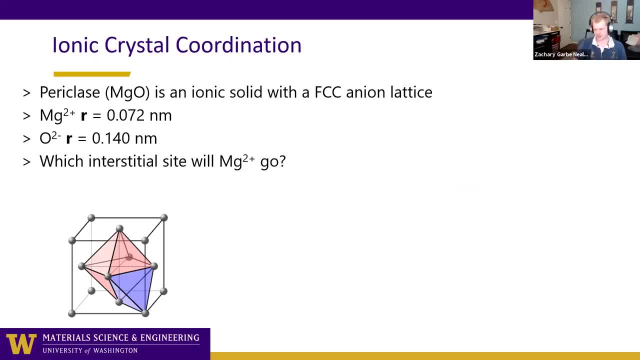 solid magnesium oxide. So magnesium is a cation: 2 plus oxygen is anion, 2, minus It the ionic solid. so oxygen arranges itself into an FCC anion lattice. So here are the lattice points for oxygen. So you can assume that oxygen is going to be on each one of these points. Okay, The question: 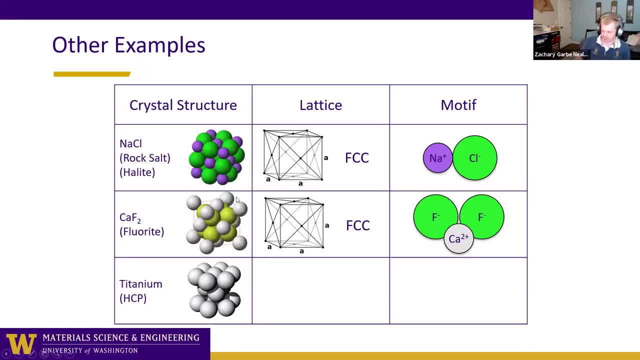 and translated it to every lattice point in the FCC, you're gonna make the fluoride structure right. So if you took, say, these three atoms right here, calcium and two fluorines, you translate this over to the next one, you're gonna build up the symmetry right. 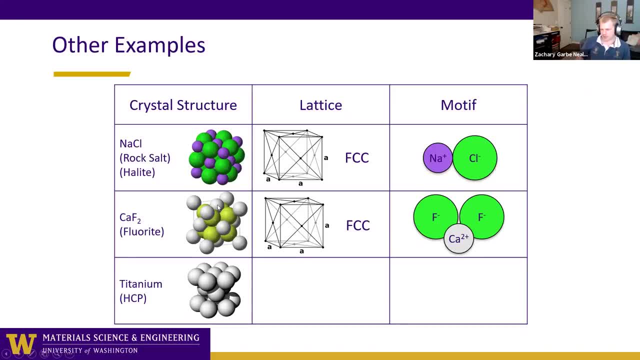 Okay, And there shouldn't be any right. There shouldn't be any overlapping When you translate it. there's no like duplicates, That wouldn't work. They're all unique. Okay, now we get to titanium, the HCP. 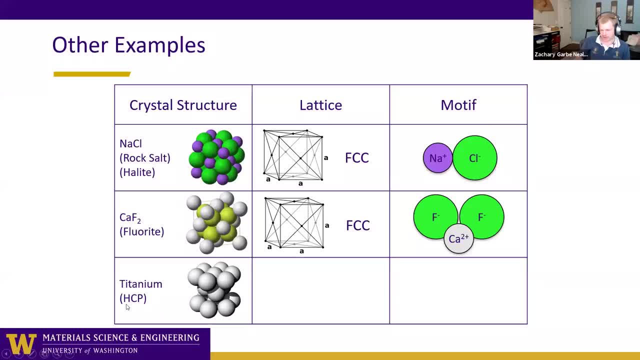 Yeah, so I wanna emphasize this as well, because a lot of students get this incorrect. HCP is a crystal structure. It is not a Bravais lattice. Okay, if you go back to the Bravais lattices and this will give away the next answer. 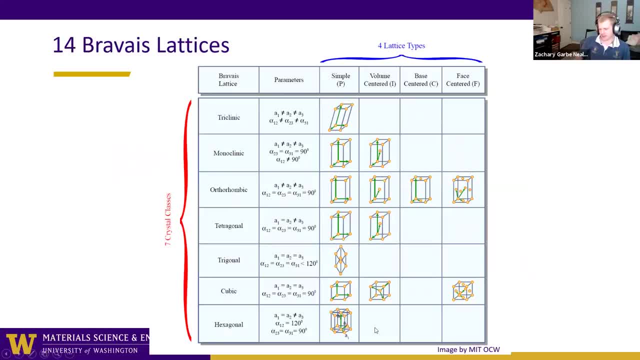 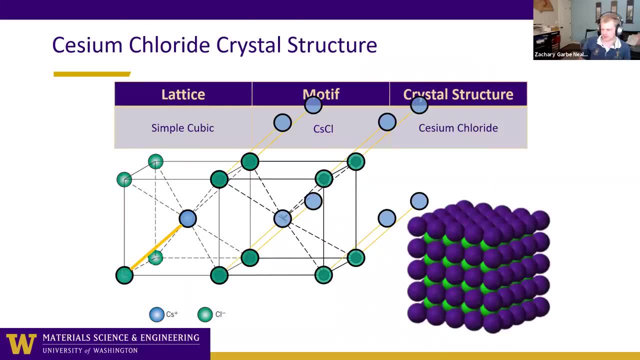 you know, hexagonal does not have any. it doesn't have face center, it doesn't have body center. All right, there's only simple. hexagonal is the only Bravais lattice for hexagonal. So the crystal structure is HCP. 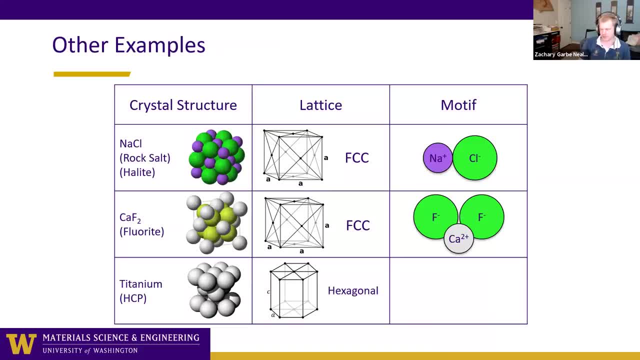 What is the lattice? I already gave away: it's hexagonal. The motif is actually two titanium atoms. Okay, So that's the point I wanna make: that lattice points and crystal structure are different. Okay, they're not the same. Lattice is just a set of points in space. 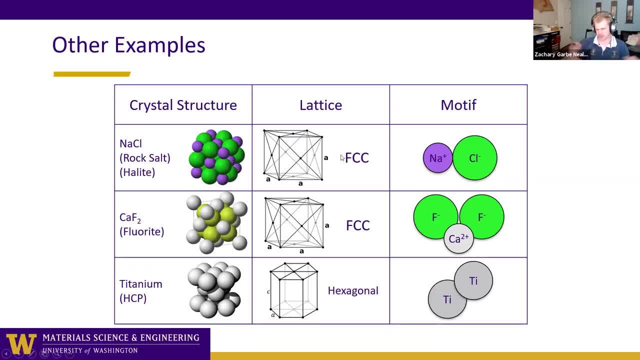 and depends on what you put onto those points in space. Okay, And that can build up, And that's how we get so many different types of crystal structures, not just 14. There's way more than 14 crystal structures, but there's only 14: Bravais, lattices. 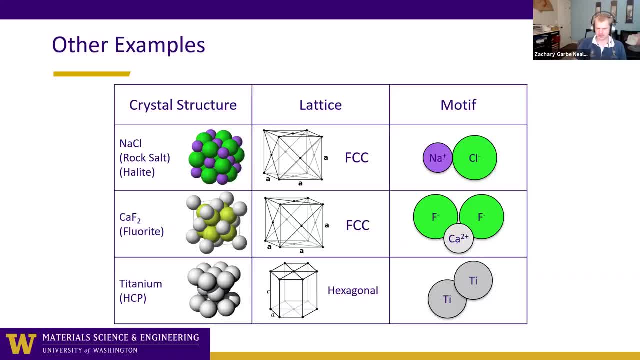 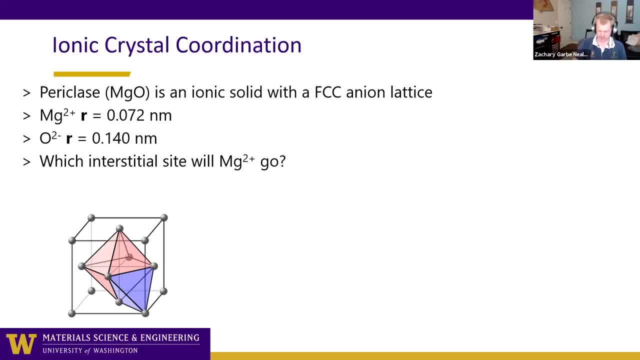 Okay, Yeah, simple, hexagonal, Let's move on. So here's a question, And I don't remember if Brush got to this in his lecture, but it's definitely part of the reading, I believe. Now here's an example of a ionic solid magnesium oxide. 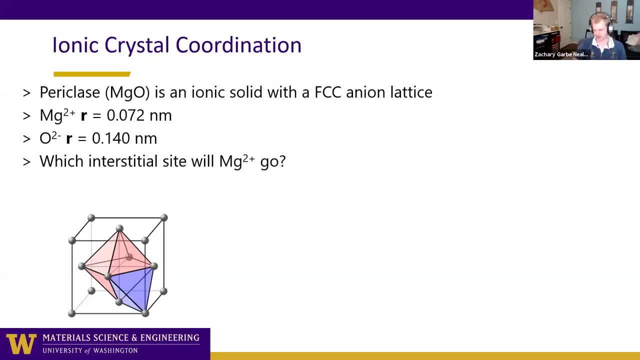 So magnesium is an ionic solid, Oxygen is a cation. two plus Oxygen is anion, two minus It the ionic solid. So oxygen arranges itself into an FCC N ion lattice. So here are the lattice points for the oxygen. 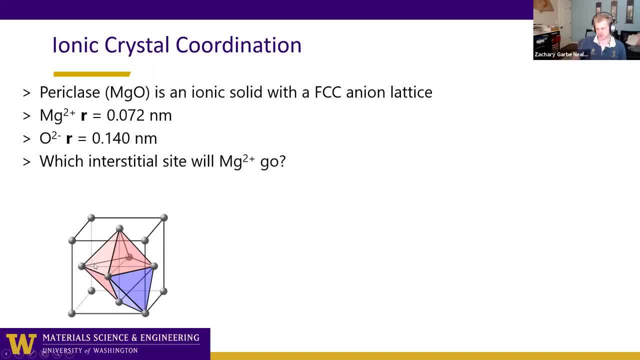 So you can assume that oxygen is gonna' be on each one of these points. Okay, the question is, where will the magnesium go? And this deals with what we call interstitials. Interstitials are the spaces in between, So in FCC. 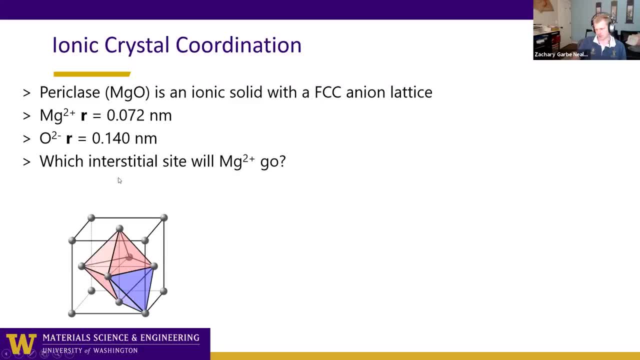 is where will the magnesium go? And this deals with what we call interstitials. Interstitials are the spaces in between. So in FCC there are two different types of interstitials. There is this red one. here is the octahedral interstitial- interstitial right That's made up from the faces. 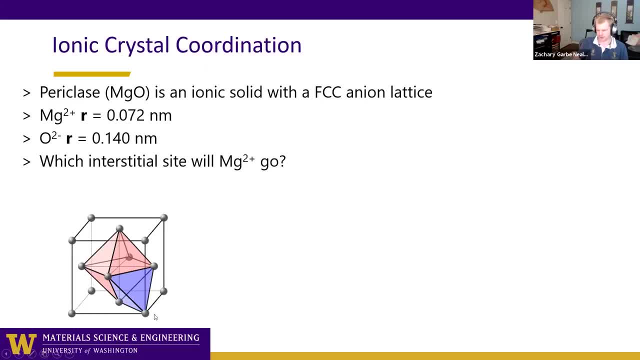 And then on the corners is the tetrahedral interstitial. So for each unit cell, well, there should be eight, there should be eight octahedral- excuse me, there should be eight tetrahedral interstitial sites, And I believe there's also. 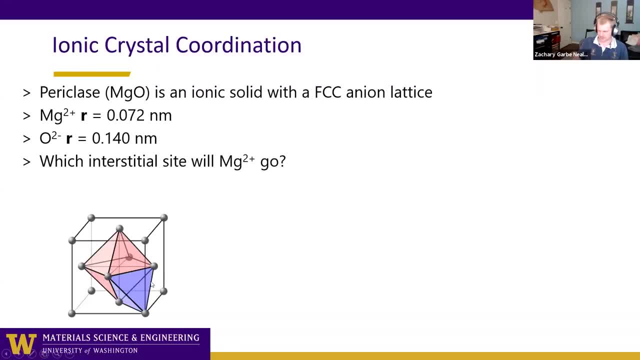 let's see: there's one on each face, seven, No, it's each edge. So there's what? one, two, three, four, that's eight, that's 12,, 13.. And oh yeah, I forgot to divide by 10.. 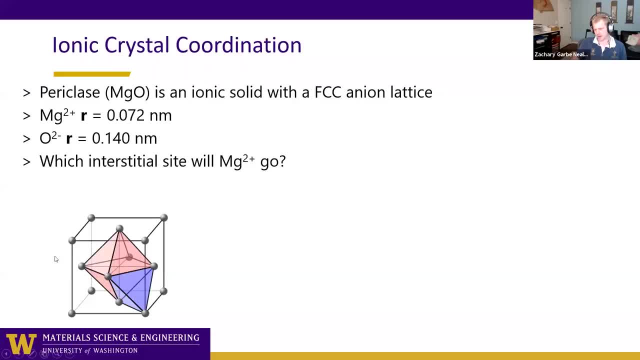 Two. Anyways, the question is: where will magnesium go? Will magnesium go into the octahedral sites or will go into the tetrahedral sites? Does anyone know how to go about solving the problem? What do we have to look at? And I believe this was part of the reading for this. 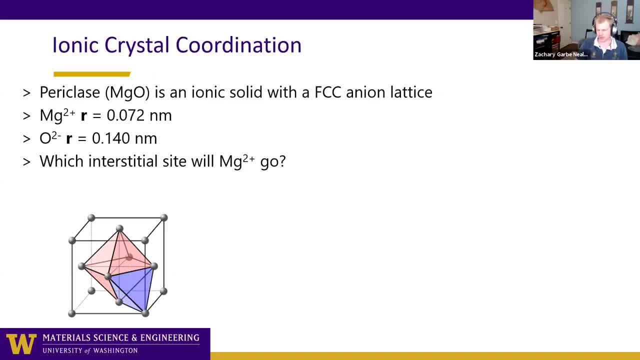 week? Yeah, the radii. So we look at the atomic radii and what do we look about? What do we need to do? Make sure they don't overreact? So what do we need to do Make sure they don't overlap? I think there's a. it's a more general. 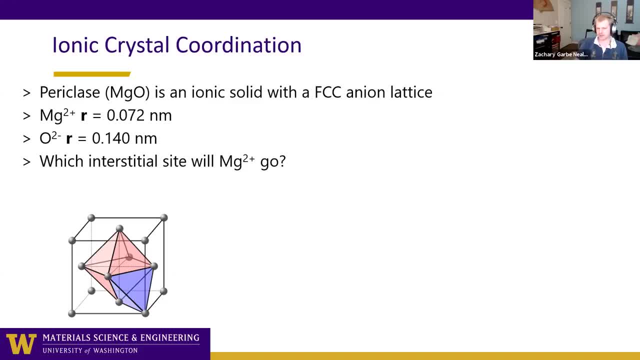 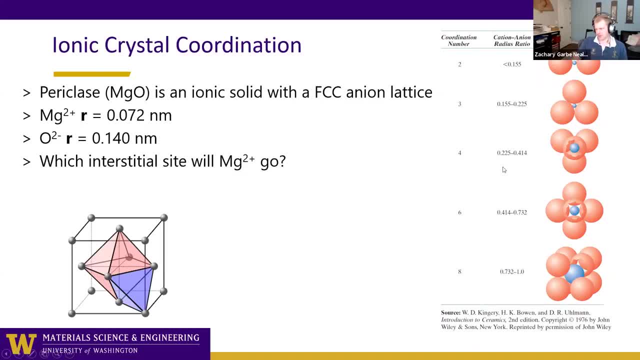 ratio of the cation to the anion ratio And you take the ratio of the cation to the anion ratio. Okay, And it's a general rule of thumb, If they fall in one of these ranges, that will be the coordination of the cation to the anion. And remember, usually the cation is the smaller. 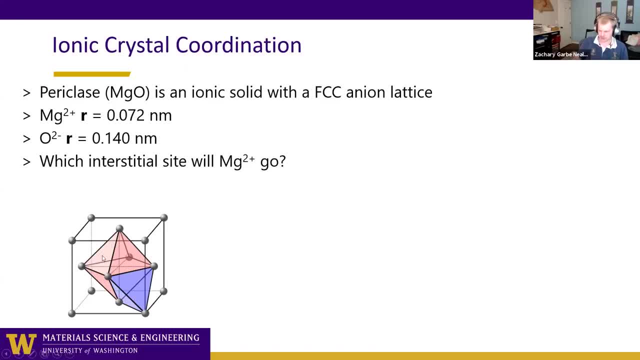 there are two different types of interstitials. There is this red one, here is the octahedral interstitial- interstitial right, That's made up from the faces, And then on the corners, is the tetrahedral interstitial. So for each unit cell, well, there should be eight. 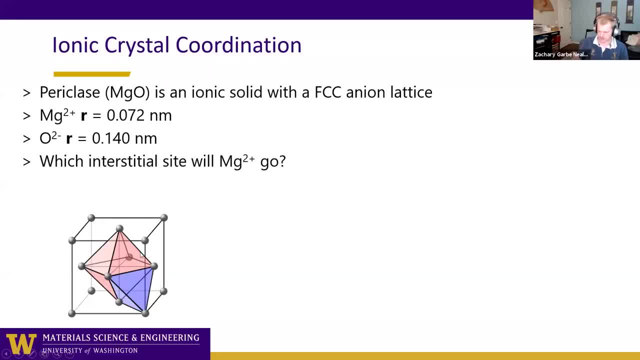 there should be eight octahedral- excuse me, there should be eight tetrahedral interstitial sites, And I believe there's also, let's see, there's one on each face, seven, No, it's each edge. So there's what? one, two, three, four, that's eight. 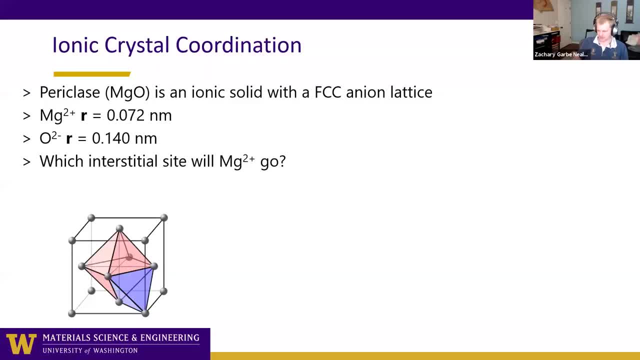 there's 12, 13.. Oh yeah, I forgot to divide by two. Anyways, the question is: where will magnesium go? Will magnesium go into the octahedral sites or will go into the tetrahedral sites? Does anyone know how to go about solving the problem? 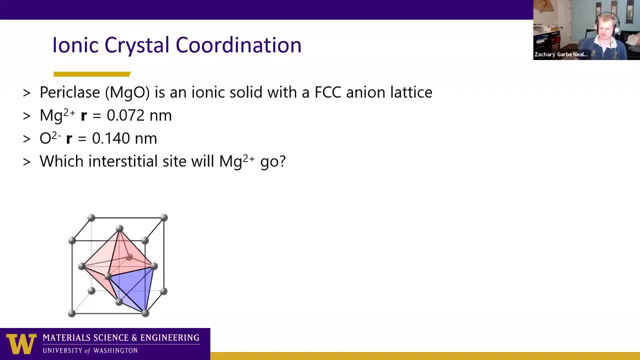 What do we have to look at? Okay, so here's aě, Here's aě over here, And I believe this was part of the reading for this week. Yeah, the radii. so we look at the atomic radii. 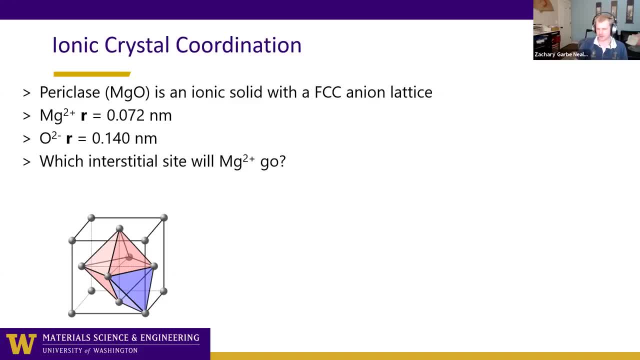 and what do we look about? What do we need to do? Make sure they don't overlap. I think there's a. it's a more general rule- coordinate- so I'll go into that. so this is from Callister. it might be chapter 14. 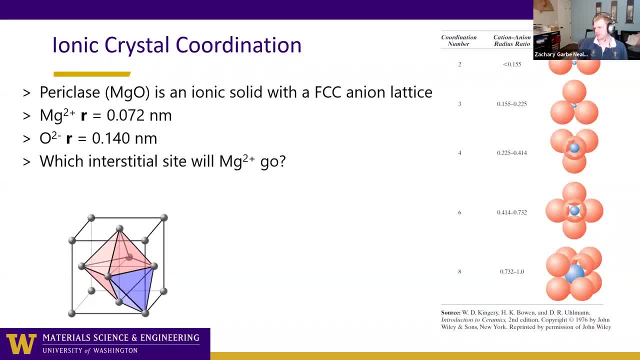 actually, which is part of your reading assignment- and you, what you do is take the ratio of the cation to the anion radius. okay, and it's a general rule of thumb, if they fall in one of these ranges, that will be the coordination of the anion or the cation to the anion and, remember I, usually the cation is the. 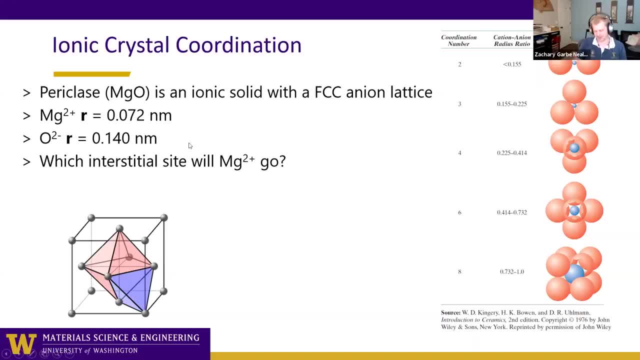 smaller anion. excuse me, I'm getting my words messed up. cation is usually the smaller ion because you're giving away electrons, your electron shell is getting smaller. the anion is usually the bigger ion because it's receiving electrons. it's it's a less, it's more loosely bounded to that atom, and so in this case, 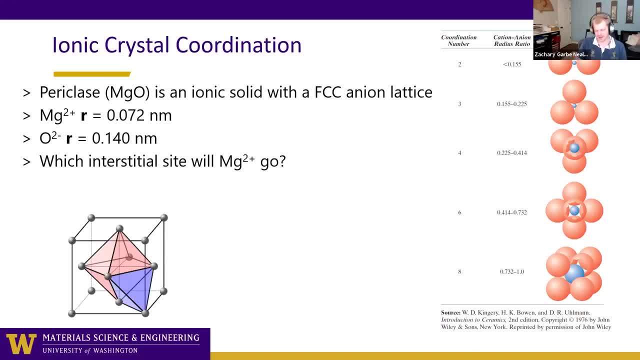 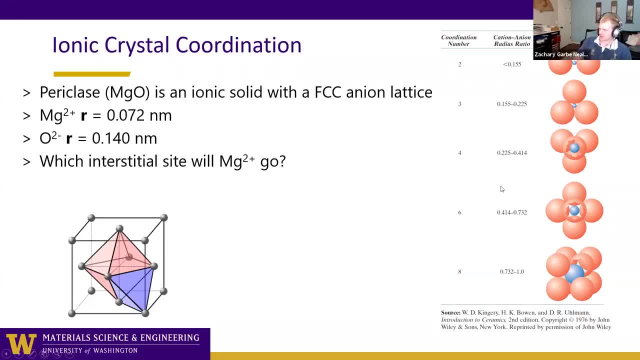 it's more loosely bounded to that atom, and so in this case you just take the ratio between the two. okay, and so the ratio between magnesium and oxygen: 0.51. so that falls into here. coordination number six, which is an octahedral. all right, so magnesium is going to fit into the octahedrals. 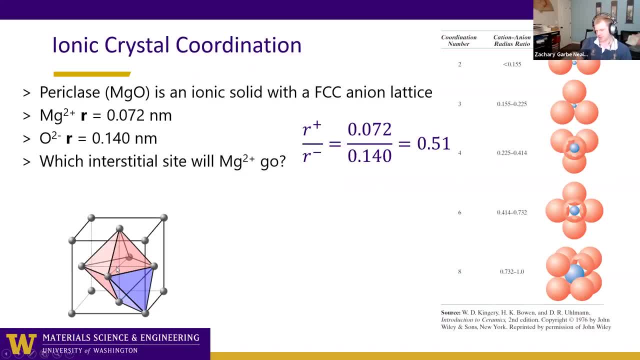 not into the tetrahedrals. it's it's more energetically favorable and that's why these these numbers are determined. it's it's which coordination makes it more energetically favorable. if you have a too small of an atom inside the octahedral, it's not very energetically. 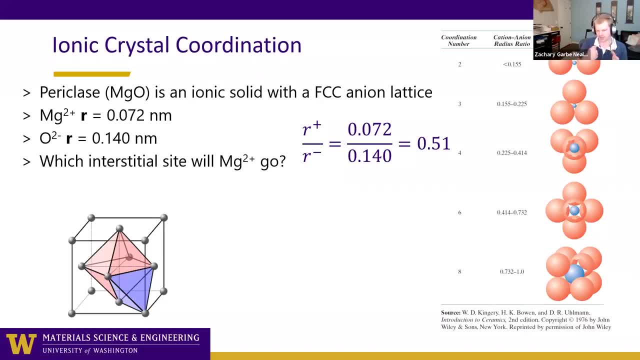 stable you can think of like a small atom rattling around in a cage. it'd rather be too big than it than too small. so this is what that looks like if we take the magnesium, put it at each of these edges and inside the center, and then if we expand this octahedral. this is the next door neighbor. 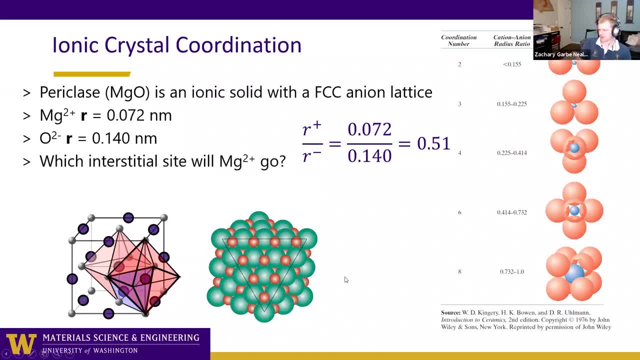 octahedral interstitial site. i think there was another question i had. yeah, what's the crystal structure of magnesium oxide? what do you guys think? and you should be able to just look at this and know right away what the crystal structure- and it's one of the crystals that we already talked. 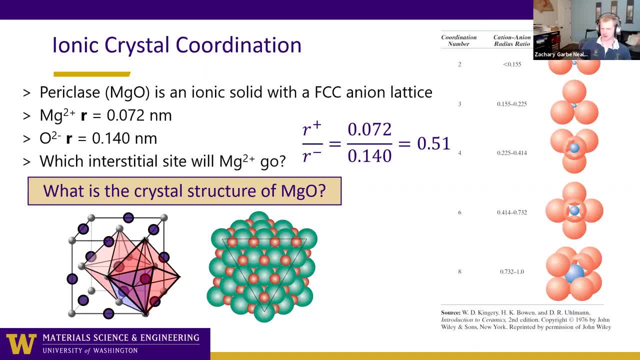 about what is the crystal structure, and what i'm looking for is the name of the crystal structure, right? so not bcc. bcc is only a crystal structure if the entire material is the same. uh, composition like iron. it's all made of iron. that can, that's the only. 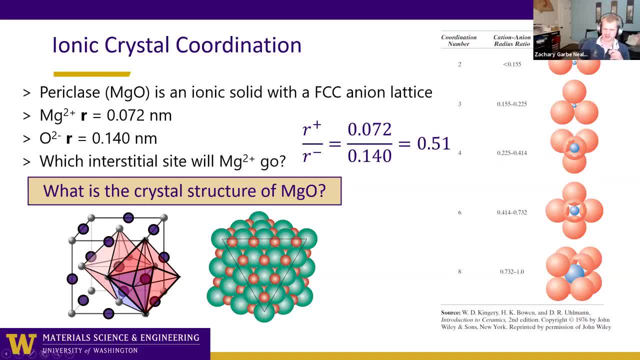 time bcc can be a crystal structure, otherwise it's a lattice. uh and uh, how? yeah, you're right, halite is correct. uh, sodium chloride, uh, crystal structure or rock salt. this is the halite rock salt or sodium chloride crystal structure. all right, it's the same as what we saw before. i won't. 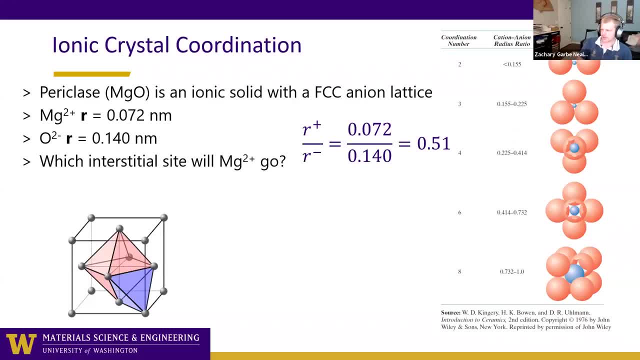 you just take the ratio between the two. you just take the ratio between the two. okay, and so the ratio between magnesium and oxygen: 0.5, 1. so that falls into here. coordination number 6, which is an octahedral. all right, so magnesium is. 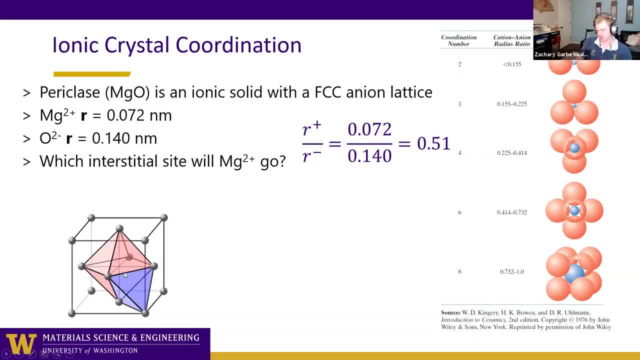 gonna fit into the octahedrals, not into the tetrahedrals. it's it's more energetically favorable and that's why these, these numbers are determined. it's it's which coordination makes it more energetically favorable. if you have a too. 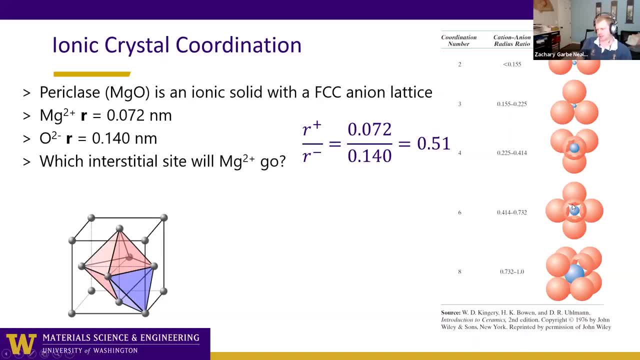 small of an atom inside the octahedral. it's not very energetically stable and that's a little bit more than you might want to have to do when you're You can think of like a small atom rattling around in a cage. It'd rather be too big than too small. 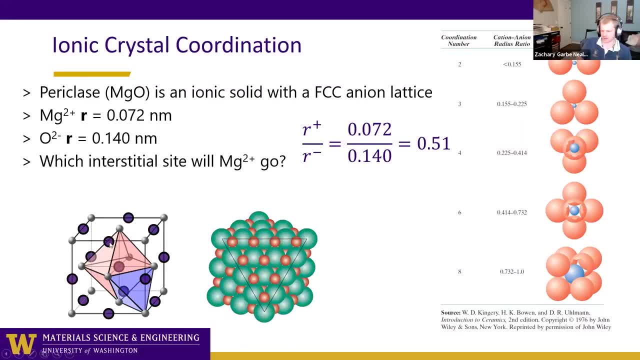 So this is what that looks like If we take the magnesium, put it at each of these edges and inside the center and then if we expand this octahedral. this is the next-door neighbor octahedral interstitial site. I think there was another question I had. Yeah, what's the crystal structure of magnesium oxide? 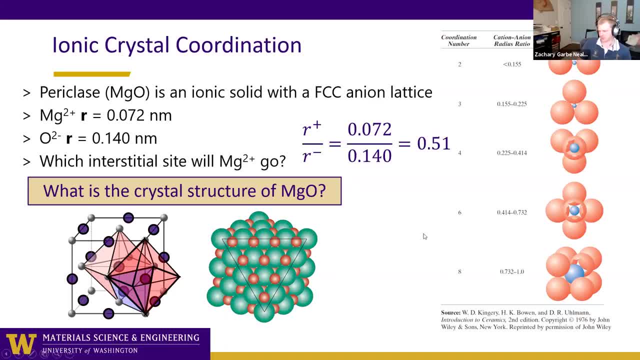 What do you guys think? And you should be able to just look at this and know right away what the crystal structure is, And it's one of the crystals that we already talked about. What is the crystal structure? And what I'm looking for is the name of the crystal structure, right? 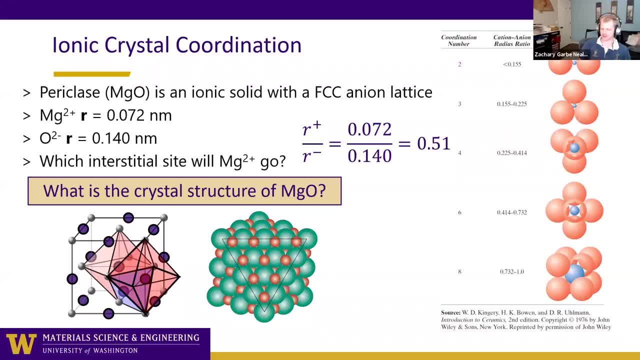 So not BCC. BCC is only a crystal structure. if the entire material is the same composition, like iron, It's all made of iron. That's the only time BCC can be a crystal structure, Otherwise it's a lattice. 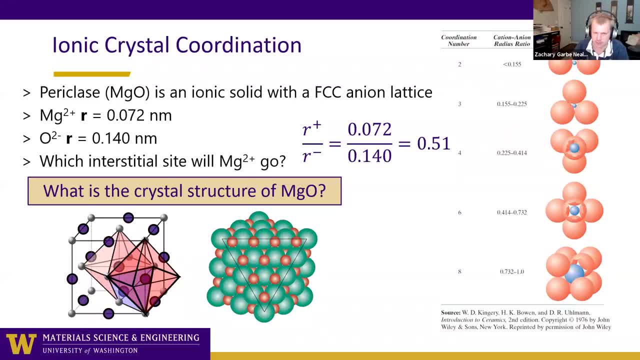 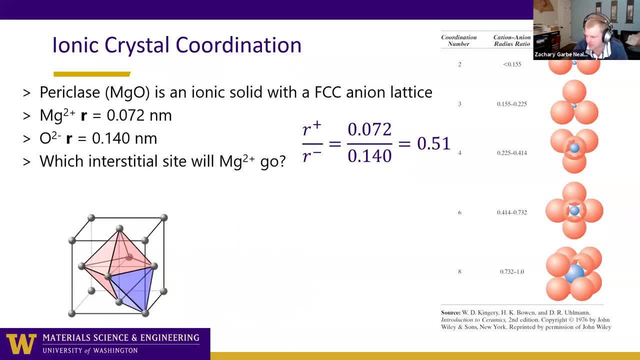 Yeah, you're right. Halite is correct, Sodium chloride crystal structure or rock salt. This is the halite rock salt or sodium chloride crystal structure. Alright, it's the same as what we saw before. I won't go all the way back. 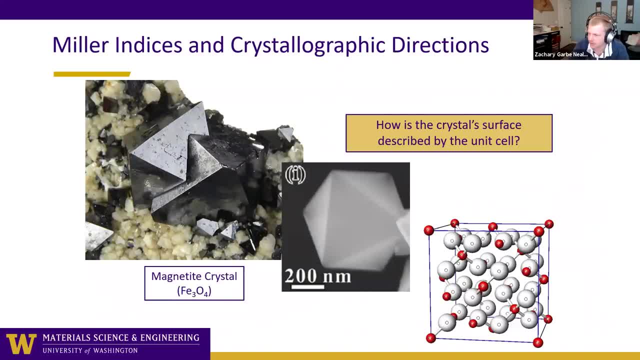 Okay, Let's go into Miller indices and crystallographic directions. So you know if we want to describe the range or the plane of atoms inside a unit cell, or perhaps what the atoms look like at the surface of different single crystals. 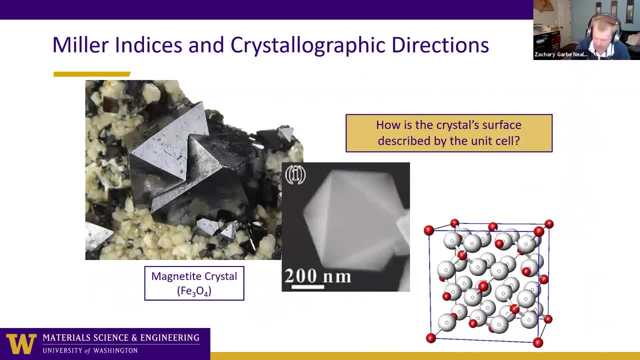 go all the way back, okay. uh, let's go into miller indices and crystallographic directions. so you know if we want to describe, uh, the range or the, the plane of atoms inside a unit cell, or perhaps what the atoms look like at the surface of different 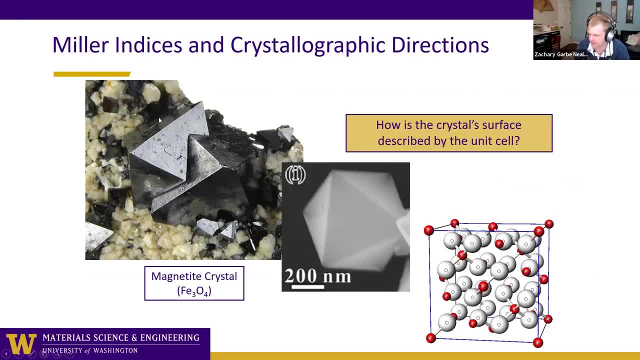 single crystals we use what's called miller indices. all right, here's an example of the spinel crystal structure. this is iron, uh, what we call this iron 304. it's also iron 2- 3 oxide, because it has mixed of iron 2 plus and iron 3 plus. it's called magnetite and the 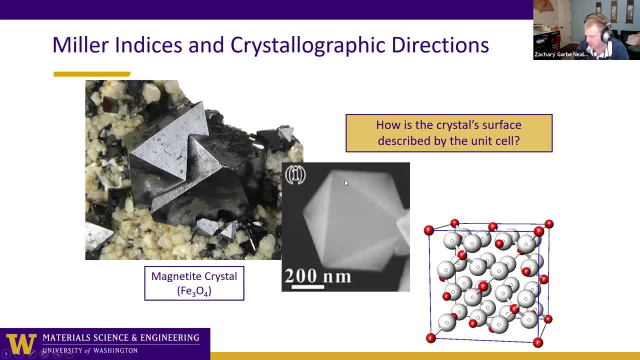 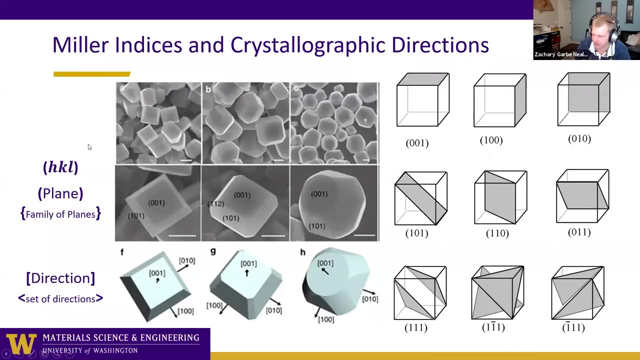 spinel crystal structure and these nanoparticles of that spinel and macroparticles, crystals having the same shape, and the shape is determined, of course, by the crystal structure. but the question is: you know, how do you, how can you describe the surface of these crystals? and we use miller indices. miller indices have this abbreviation hkl, and these are integer values. 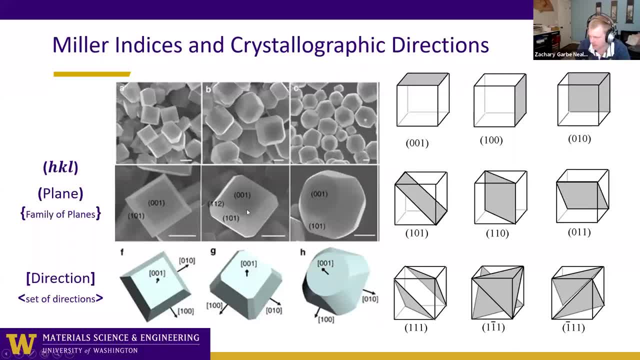 so here's another example of some kind of nanocrystal, i forget, but it describes the different surfaces of this crystal with the miller indices. and then there's also- you should just distinguish it from the direction- uh, where are the crystal structures such as halite found? um, i don't quite, don't quite understand the question where crystal structures 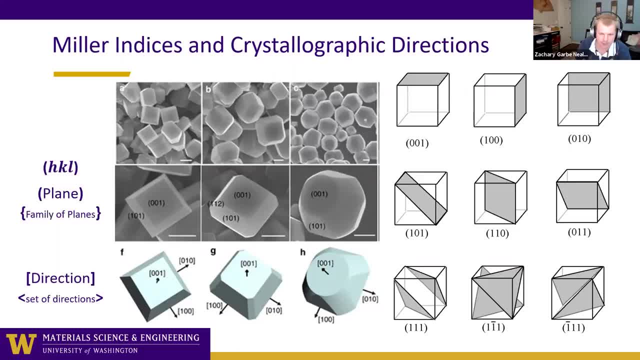 such as halite found. you mean like on earth? oh, the like a list of crystal structures? um, i i am pretty sure chapter three- if not chapter three, it's chapter 14, i believe, was part of the reading. there's a small reading of some in chapter 14 i think that talks about ceramic crystals. 14 or 12. oh, did i mix that up? 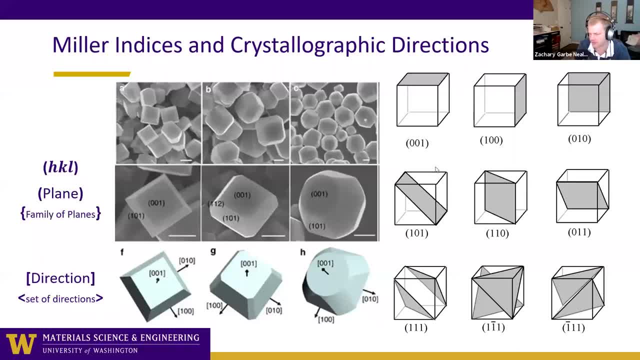 it might be 12, then if i'm. i don't have it right in front of me, so i'm not sure it might be 12 not 14. uh, the chapter is about, uh, ceramic crystals, or ionic crystals, i believe, and it should give you a different list of crystal structures. um, and then the direction. uh are just 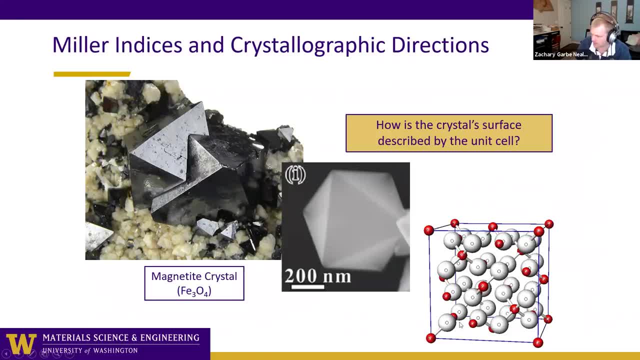 we use what's called Miller indices. Alright, here's an example of the spinel crystal structure. This is iron. This is iron 3-O-4.. It's also iron 2-3 oxide because it has a mix of iron 2-plus and iron 3-plus. 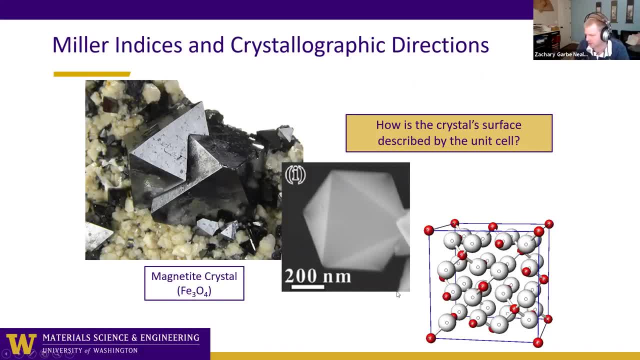 It's called magnetite. It makes the spinel crystal structure and these nanoparticles of that spinel and macroparticles, crystals having the same shape, And the shape is determined, of course, by the crystal structure. But the question is: you know, how do you, how can you describe the surface of these crystals? 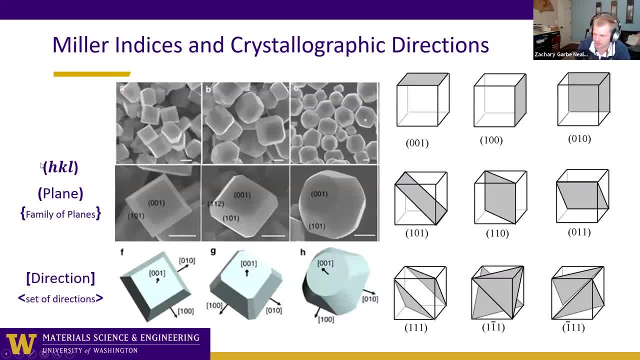 And we use Miller indices. Miller indices have this abbreviation HKL, and these are integer values. So here's another example of some kind of nanocrystal- I forget, but it describes the different surfaces of this crystal with the Miller indices. And then there's also 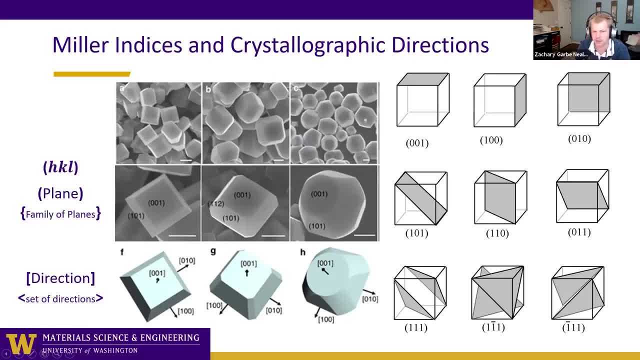 you should just distinguish it from the direction. Where are the crystal structures such as halite found? I don't quite, don't quite understand the question: Where are crystal structures such as halite found? You mean like on Earth? Oh, like a list of crystal structures? I am pretty sure chapter 3, if not chapter 3, it's chapter 14,. 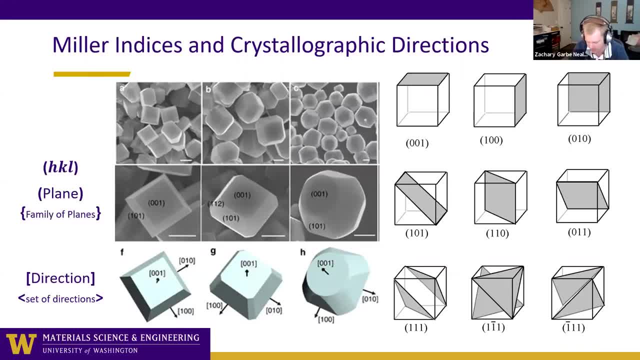 I believe was part of the reading. There's a small reading of some in chapter 14.. I think that talks about ceramic crystals. 14 or 12?? Oh, did I mix that up? It might be 12, then if I'm I don't have it right in front of me. 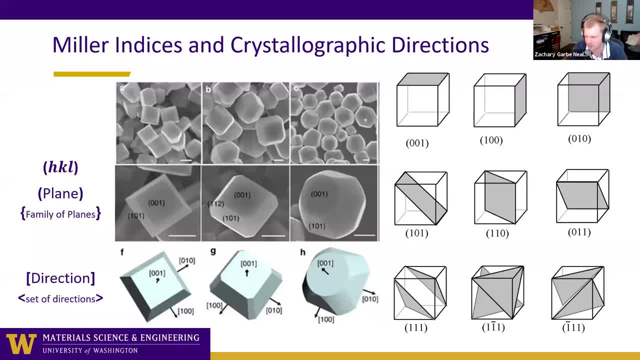 so I'm not sure. It might be 12,, not 14.. The chapter is about ceramic crystals, or ionic crystals, I believe, and it should give you a different list of crystal structures. And then the direction are just vectors, but you need to make sure that you're using the correct notation If you're talking about a plane. 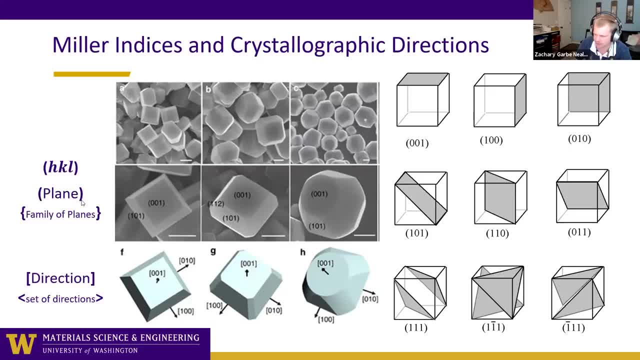 in space for Miller indices. it's using parentheses or sometimes these curly brackets. We're talking about a family of planes And if it's a direction, you use the square brackets or these little. what do you call those? I don't know. 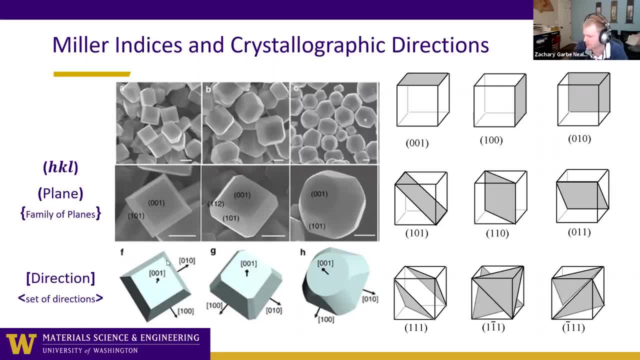 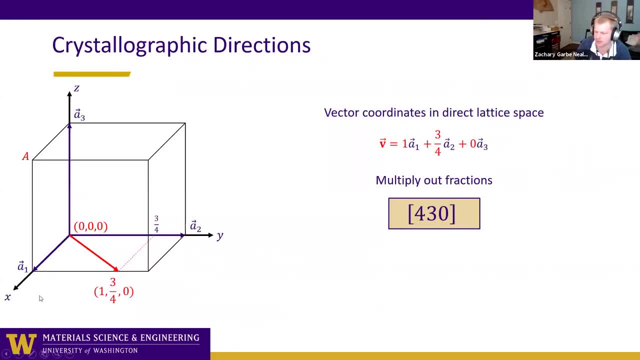 carrots, arrows, whatever- for a family of directions. So I have a couple problems, but I think we'll just go through them because we don't have much time And, like I said, don't feel obligated to stay I this recording will be posted this evening, once it. 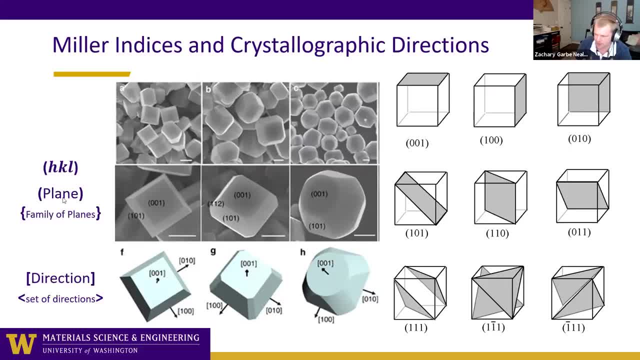 characters, but you need to make sure that you're using the correct notation. if you're talking about a plane in space, uh, for miller indices, it's using parentheses or sometimes these curly brackets. we're talking about a family of planes, um, and if it's a direction, you use the square brackets or these. 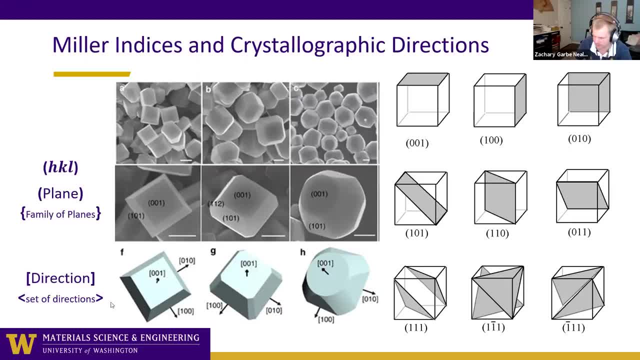 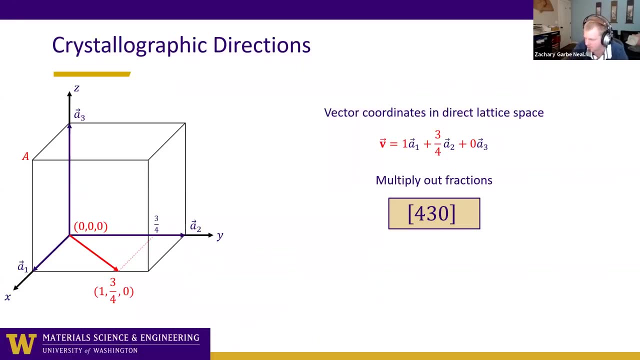 little. what do you call those, i don't know- carrots, arrows, whatever for a family of directions. so i have a couple problems, but i think we'll just go through them because we don't have much time and, like i said, don't feel obligated to stay. i this recording will be posted uh this evening, once it finishes compiling. uh, so for crystallographic. 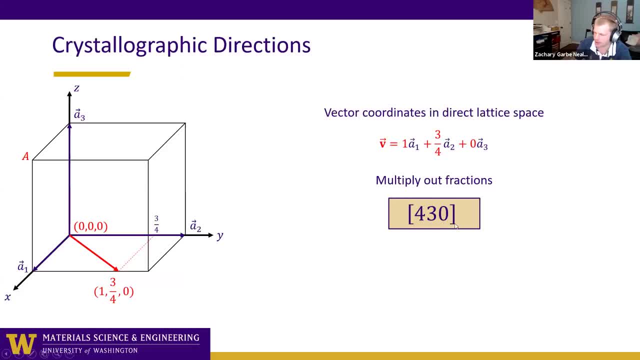 directions. all right, using the square brackets. uh, it's very simple, just vector math, all right. so you take the, the final coordinate point in real space and minus the initial coordinate point. um, or, excuse me, this should be lattice space, because this, this, uh, you know, here i show x, y and z. 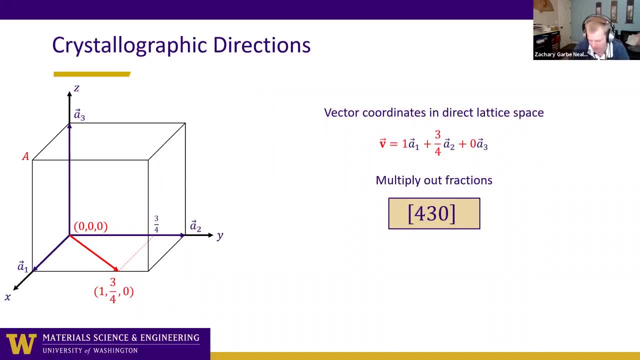 and to think of three dimensions. but that's only correct if your unit cell is orthogonal. okay, if it has, uh, these right angles. but you, as you know, some unit cells don't have right angles at the origin. so it's not really correct to say x, y and z, uh, but we're talking about lattice space. 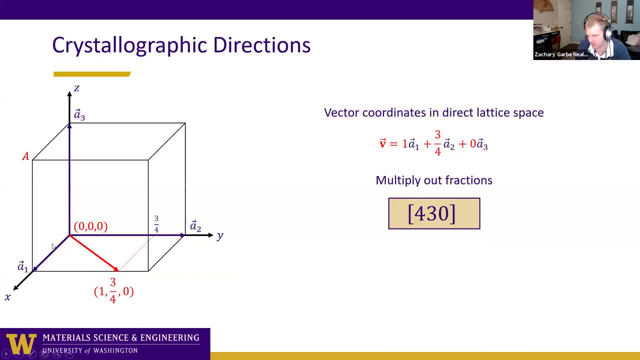 the, the vector math will still be the same. so you should use these uh unit vectors instead of x, y and z, but in these examples they're all the same. so you should use these uh unit vectors instead of x, y and z, but in these examples they're all the same, so you should use these uh unit vectors. 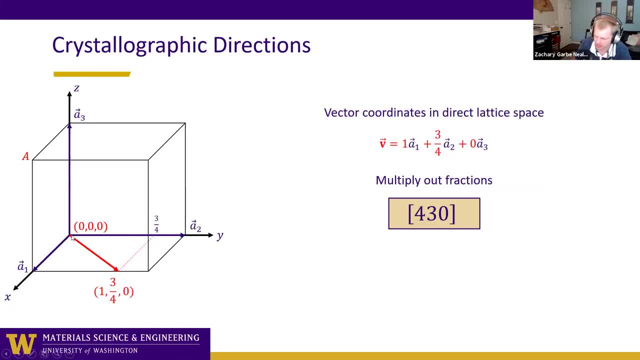 cubic. so it's, it's all the same. but, like in this example, you know, just doing the vector math, finding the end end coordinate, the beginning coordinate, and that will give you, and you should multiply the fractions out. so in this example the end coordinate is one and then three quarters zero. 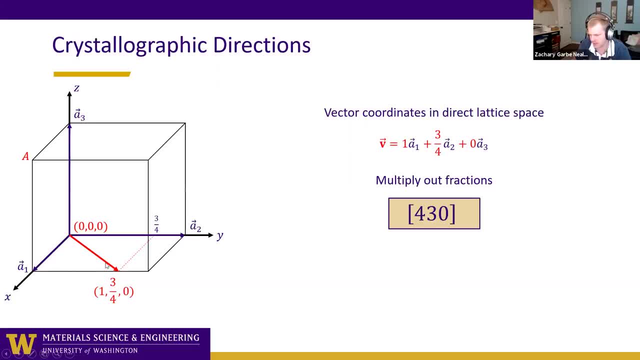 because there's no. there's no change in the z dimension. um initial is the origin, so you need to do is multiply by four to remove fractions. okay, so there's no fractions in the matrix, but you can replace them bysover. so that's the original idea of the searches byletter. 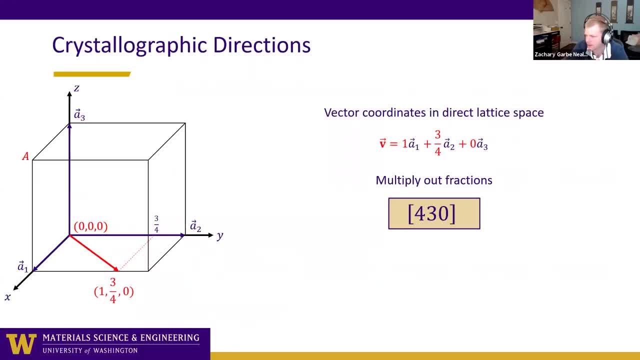 finishes compiling. So for crystallographic directions, alright, using the square brackets, it's very simple, just vector math. alright, So you take the, the final coordinate point in real space and minus the initial coordinate point, Or, excuse me, this should be in lattice space, because this you know. here I show x, y and z and 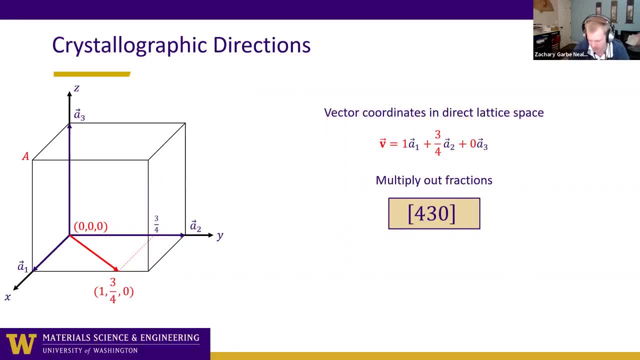 to think of three dimensions. but that's only correct if your unit cell is orthogonal. okay, if it has these right angles. But as you know, some unit cells don't have right angles at the origin. So it's not really correct to say x, y and z. 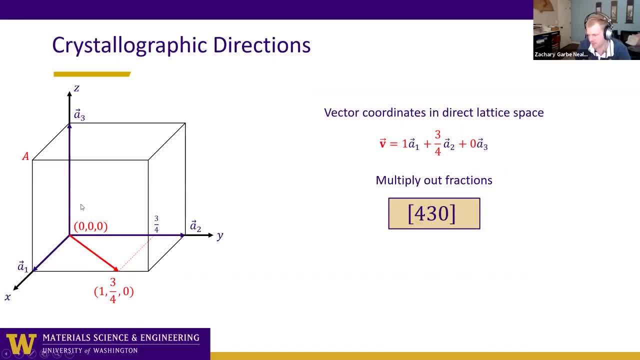 but we're talking about lattice space. The vector math will still be the same, so you should use these unit vectors instead of x, y and z. But in these examples they're all cubic, so it's all the same, But like in this example, 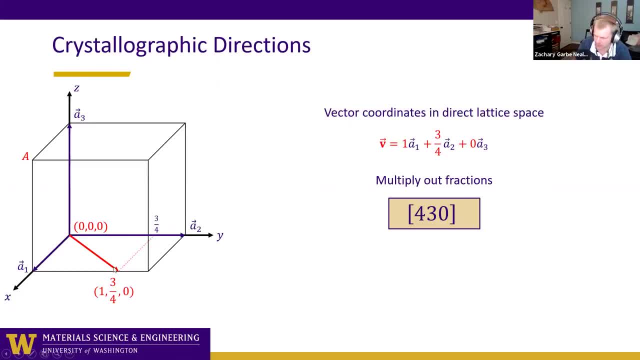 you know, just doing the vector math, finding the n-coordinate, the beginning coordinate, and that will give you, and you should multiply the fractions out. So in this example the n-coordinate is one and then three-quarters zero, because there's no change in the z-dimension. 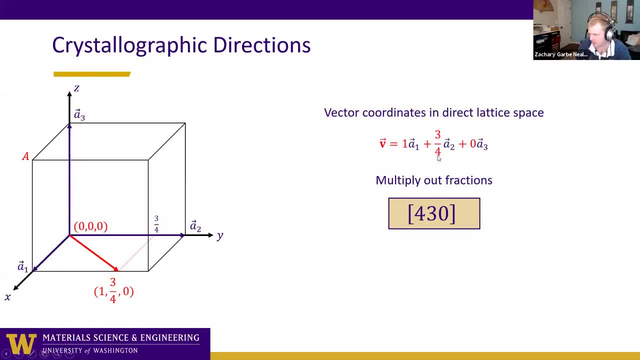 Initial is the origin. so you need to do is multiply by four to remove fractions. okay, So there's no fractions in the Miller notation for directions or for values. So this direction would be called brackets four, three, zero. Okay, I had some questions that I was going to have you guys do yourself. 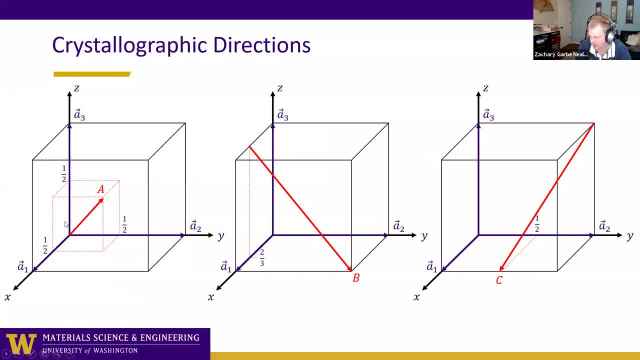 but because there's not enough time, and I'm pretty sure your homework deals with questions like this as well, But here I'll just go through this. So this direction: to point A, the coordinates are one-half, one-half, one-half and it starts at the origin. So then, if we multiply, 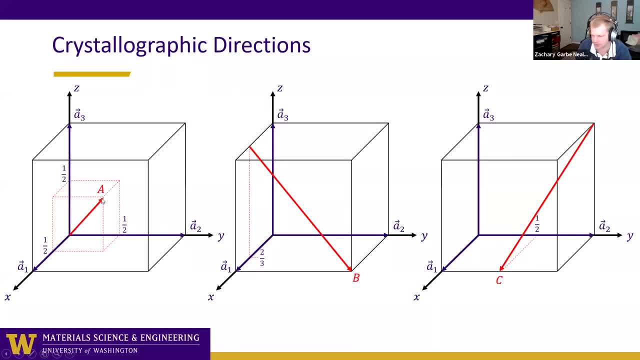 out the fractions, so we multiply everything by two. this is going to be one one one. all right, in brackets, one one one. this is the one one, one direction. this one is not starting at the origin, okay, so you have to kind of do the math here. uh, so we start and you can always move this to the. 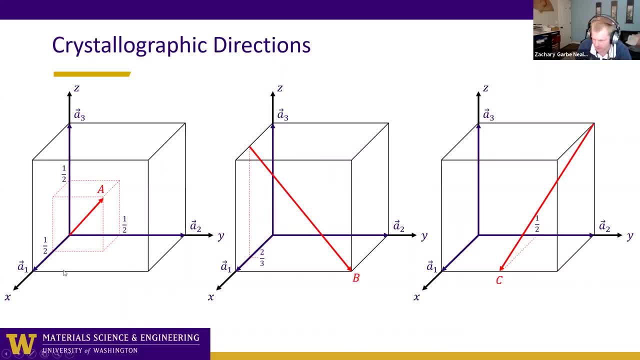 all right. so when you look at the wave 3000, you'll see that you'll have two different. all right, so when you look at the wavea inclusivw and then again, the most important is this is that you don't have to come up with a derivative. you can, just you can write it in your 계. a is pictures. 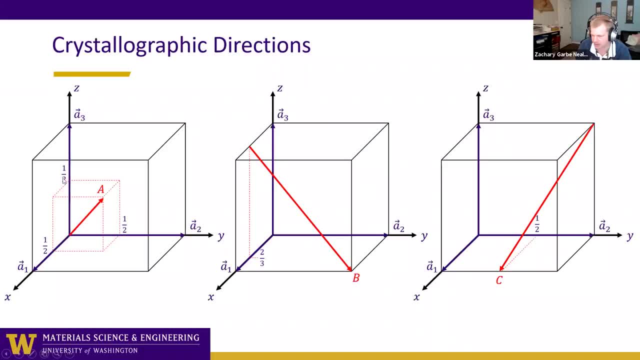 or values, and then you can say: to take a different model, and then the cost is a Russian cost, is the term Sabrina spielt, your muito right. and then they: you should multiply by two. and then you, it starts at the origin. So then, if we multiply out the fractions, so we multiply everything by. 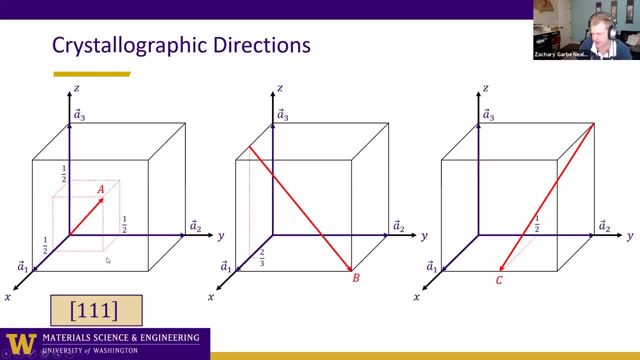 two: this is going to be 1, 1, 1,. right In brackets: 1, 1, 1.. This is the 1, 1, 1 direction. This one is not starting at the origin, okay, So you have to kind of do the math here. 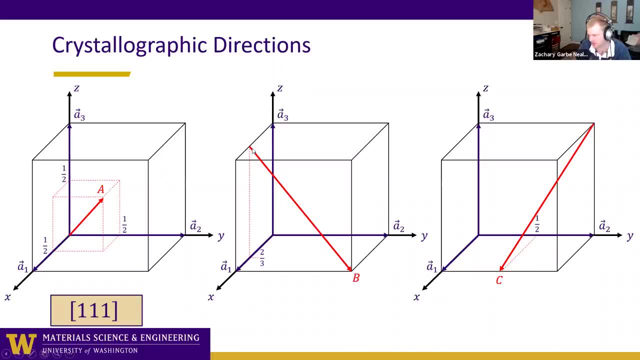 So we start, and you can always move this to the origin to make it easier, and that's what I'll try to visualize. So in the x direction, we're moving over one-third, We're going from two-thirds to one, okay. And then in the y direction, we're moving one and the z direction we're moving. 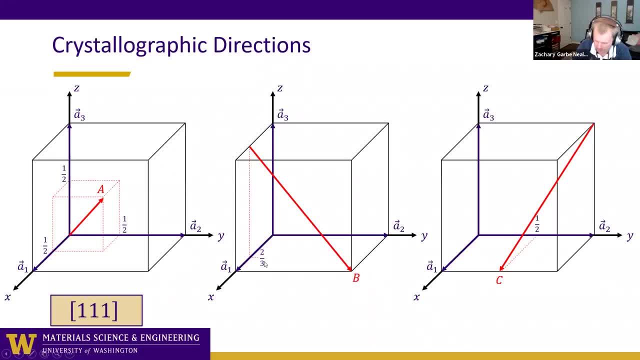 negative one For negatives. in Miller notation, negatives are written with a bar over the number. okay, So we need to multiply out the fractions. So this was what did I say: one-third for the x direction. So we're going to multiply everything by three, So it's going to be turning to three. and then to one in the y direction and then one- excuse me, one-third- for the x direction. So we're going to multiply everything by three. So we're going to multiply everything by three, and then to one in the y direction and then one. 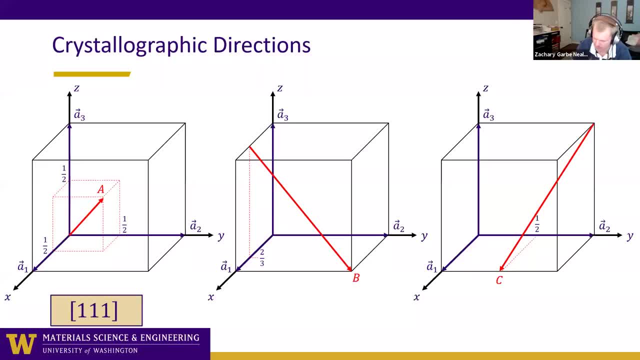 Excuse me, I'm sorry I messed that up. It's gonna be one three, three bar- Okay. one three, three bar, Okay. three bar means negative. And then the last one. we're going from this corner here. 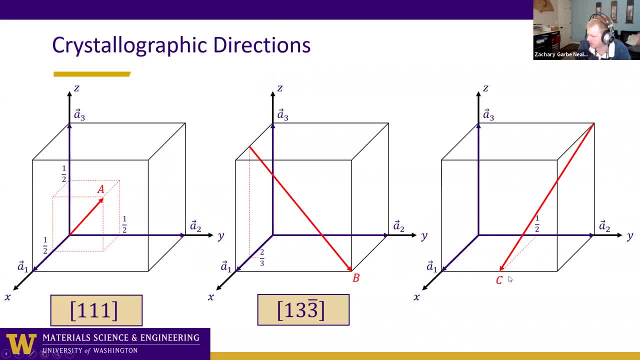 removing positive one in the X direction, negative 1 1⁄2 in the Y direction and negative one in the Z direction. okay, we remove the fractions, so we're gonna multiply everything by two, so it's gonna be two. one bar, one bar. let's see. 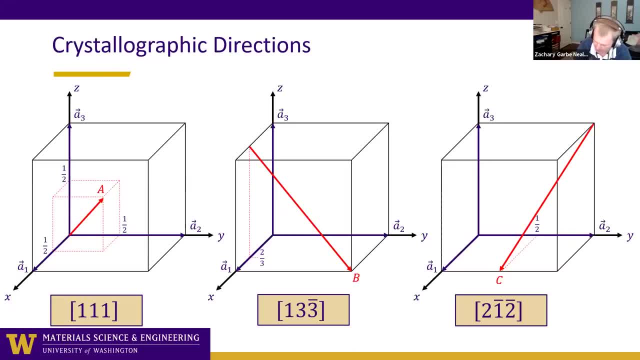 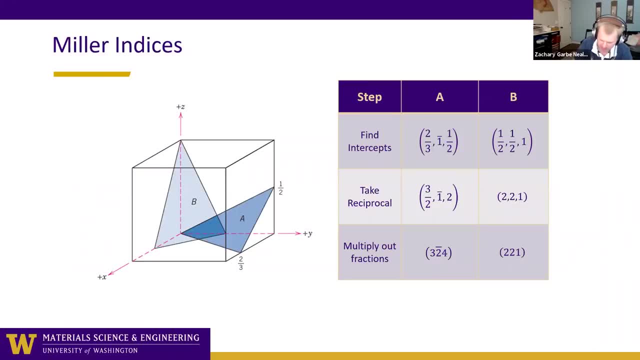 Oh, excuse me, did I do that wrong? Two, one bar, two bar. yeah, I forgot. Okay, now for Miller indices, talking about planes, it's a bit more complex. it's not as simple. We need to change it into what we call reciprocal space. 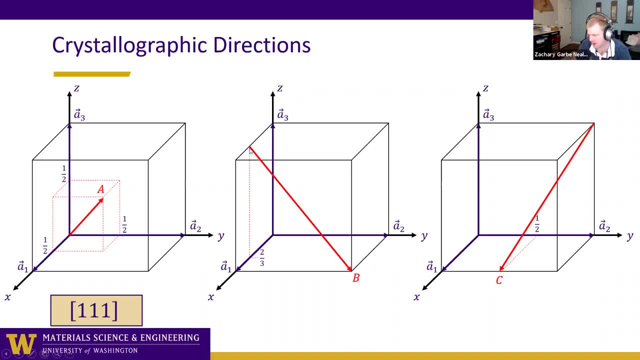 origin to make it easier, and that's what i'll try to visualize. so in the x direction we're moving over one third, we're going from two thirds to one, okay, and then in the z direct y direction we're moving one, and the z direction we're moving negative one. uh, for negatives in miller notation: 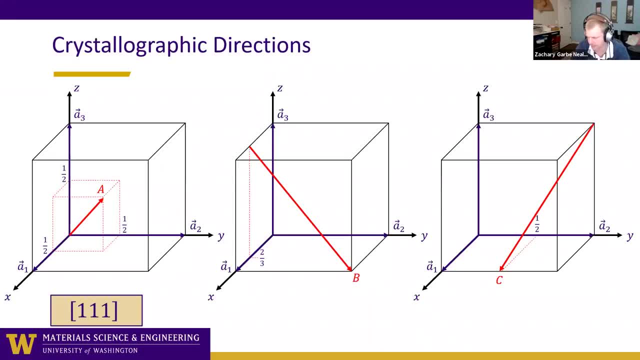 negatives are written with a bar over the number. okay, so we need to multiply out the fraction. so this was, uh, what i say: one third for the x direction. so we're going to multiply everything by three, so it's going to be turned into three, and then it's one in the y direction and then 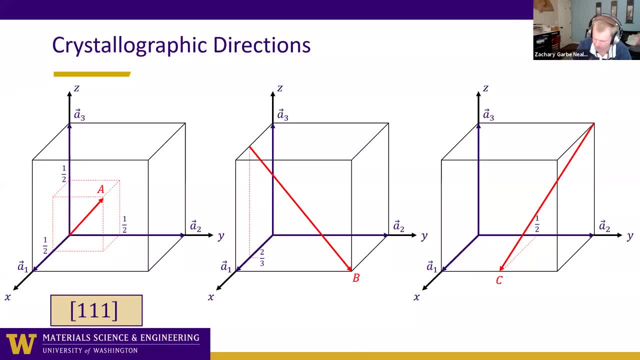 one. excuse me, i'm sorry, i messed that up. it's going to be one three, three, three bar- okay, one three, three bar, okay, three bar means negative. and then the last one. we're going from this corner here we're moving. uh, positive one in the x direction, negative one half in the 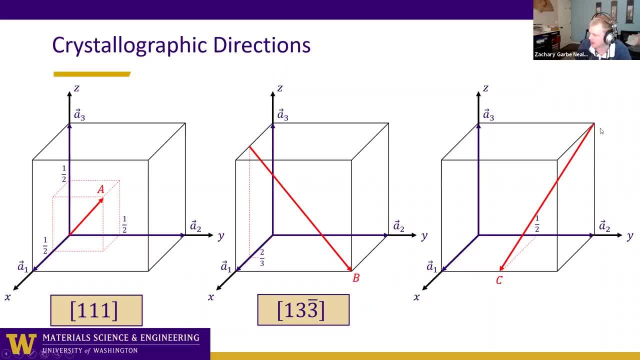 y direction and negative one in the z direction. okay, we remove the fraction, so we're going to multiply everything by two. so it's going to be two, one bar, one bar. let's see, oh, excuse me, did i do that wrong? two, one bar, two bar. yeah, i forgot. 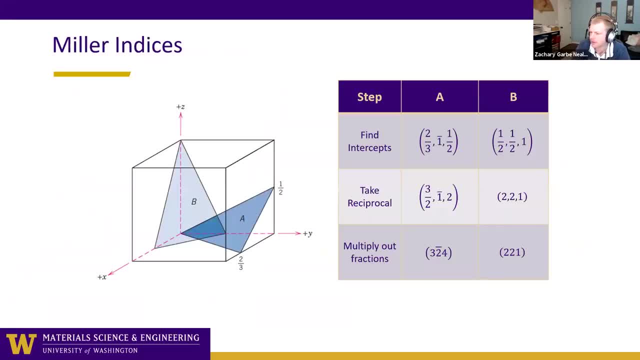 okay, uh, now for miller indices. talking about planes, it's a bit more complex. it's not as simple. there's a uh, we need to change it into what we call reciprocal space, um, but it's still not too complicated. a lot of your homework will be uh will have some of these problems. in fact, this might. 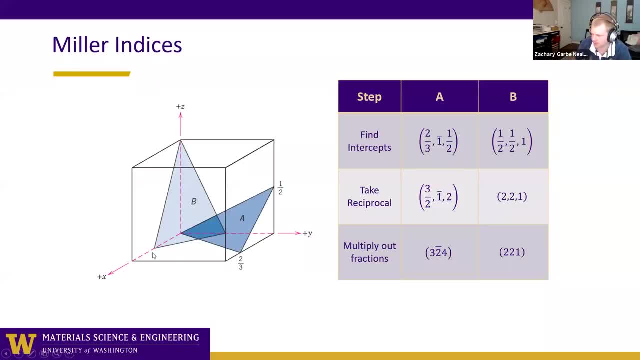 even be a problem from your homework. let's start with uh b, for example. so we want to find out what the miller indices of plane b is. b is easier than a, so we'll start with b. so what you need to do is, from the origin, find. 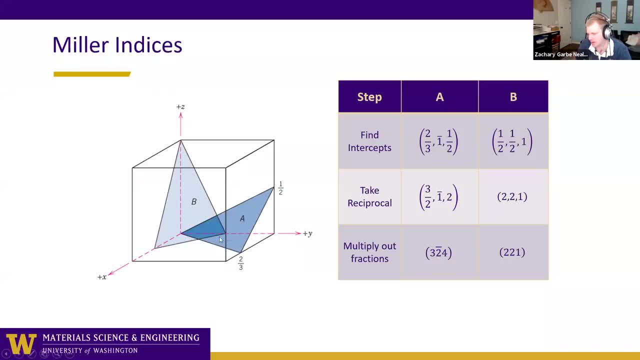 the intercepts of this plane with the different axes, all right, so this b plane intercepts x axis at one half, okay. it intercepts the y axis at one half and intercepts the z axis at one, okay. and then the next step is to find the intercepts of this plane with the different axes. all right, so. 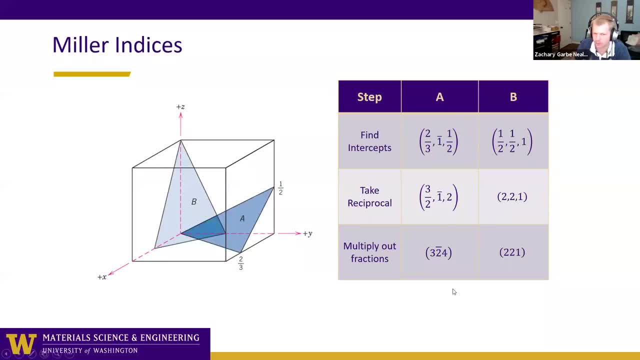 but it's still not too complicated. A lot of your homework will have some of these problems. In fact, this might even be a problem from your homework. Let's start with B, for example. So we wanna find out what the Miller indices of plane B is. 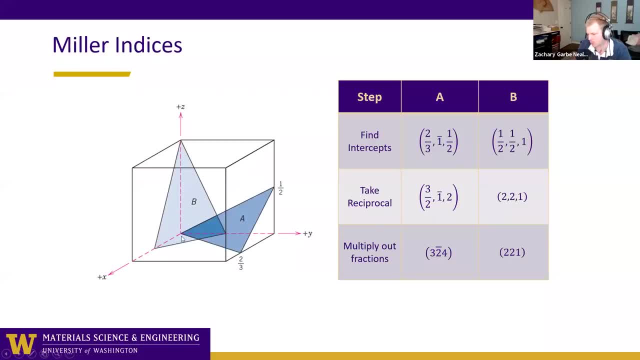 B is easier than A, so we'll start with B. So what you need to do is, from the origin, find the intercepts of this plane with the different axes. All right, so this B plane intercepts X axis at 1 1⁄2,. 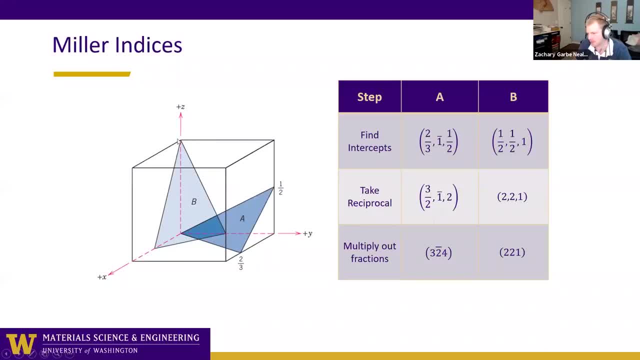 okay. It intercepts the Y axis at 1 1⁄2, okay, And it intercepts the Z axis at 1, okay, And then the next step is to take the reciprocal. So this is how it's different than the regular vector notation. 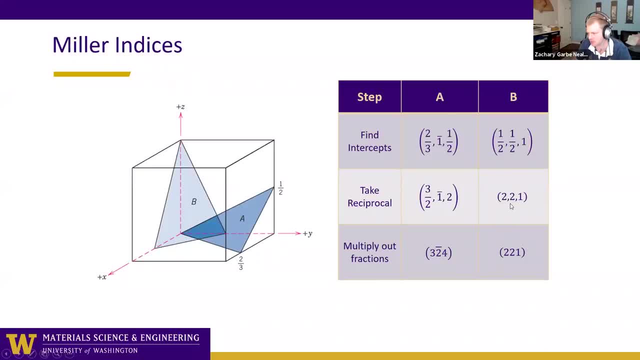 We're gonna take the reciprocal of these intercepts so it becomes two, two, one. reciprocal of one is one, And then, if there's any fractions, you multiply them out And then the final notation is two, two, one for this plane. 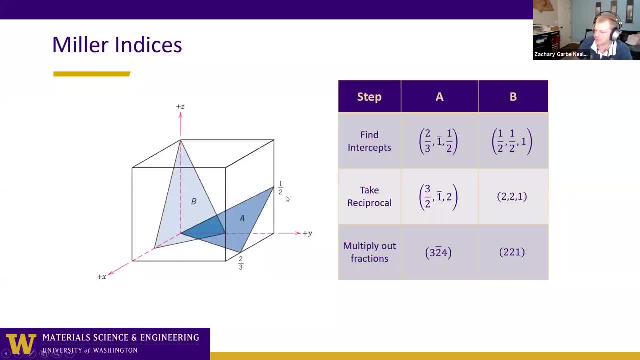 That's how we describe this plane. For A it's a bit more complex, because A intersects our origin, So we need to move our origin. We can't have it intersect the origin. We need to move the origin in order to calculate it. 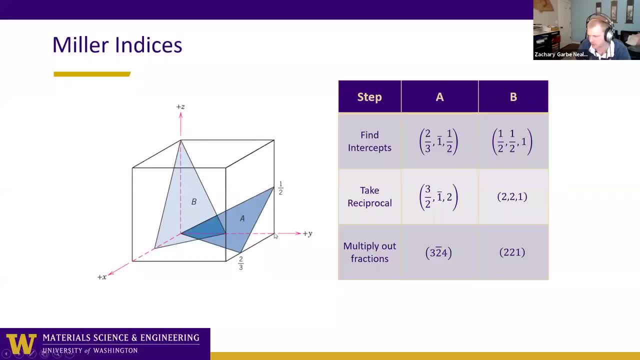 So if we move the origin to this position here, so we consider this 0, 0, 0,. oops, oh sorry. And the X axis intercepts at 2, 1⁄3.. The Y axis- now we're going to negative- intersects at 1.. 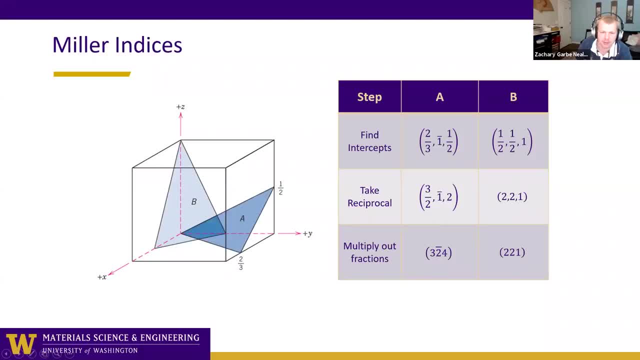 And the Z axis intercepts at 1 1⁄2.. Let me see there's a question: How do we know when to write two, two, one that we mean the plane and not the vector. Oh yeah, so the vector is always gonna be. 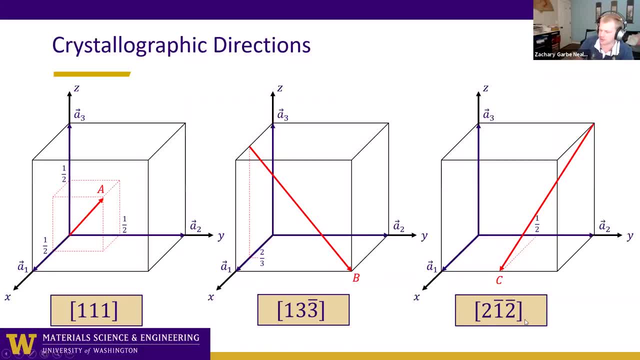 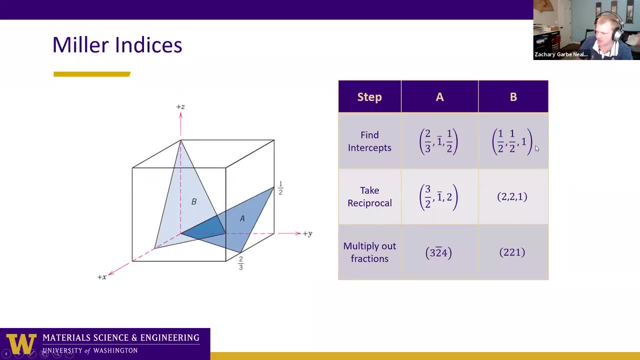 this is the square brackets. Whenever you see a square bracket, you know it's a vector, a direction, But when it's a plane, we use the parentheses. So that's how you know. So moving, going back, let's see where was I. 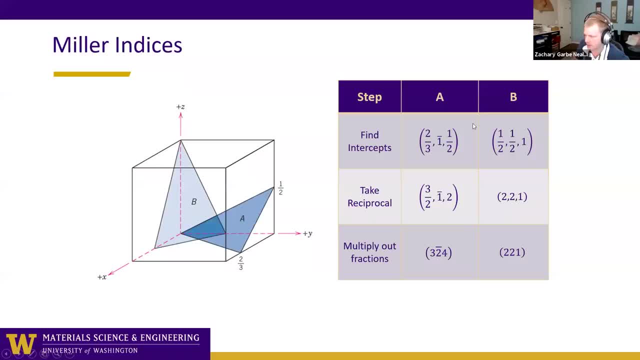 The Y direction is negative one and the Z direction is 1 1⁄2,. right, here is the- excuse me, the Z intercept is 1 1⁄2.. Then take the reciprocal, so 2 1⁄3 becomes 3 1⁄2. 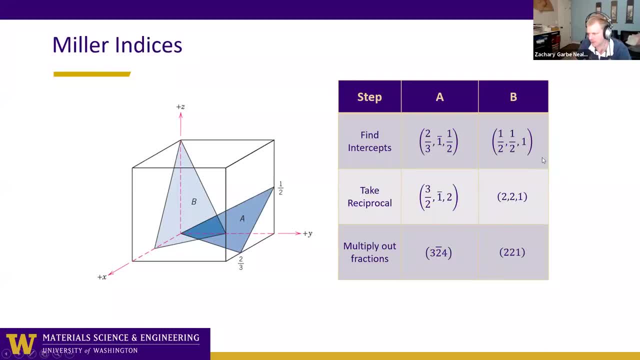 what we're going to do is to take the reciprocal. so that's what this, this is how it's different than the regular vector notation. we're going to take the reciprocal of this, these intercepts. it becomes two, two, one. reciprocal of one is one and then, uh, if there's any fractions, you. 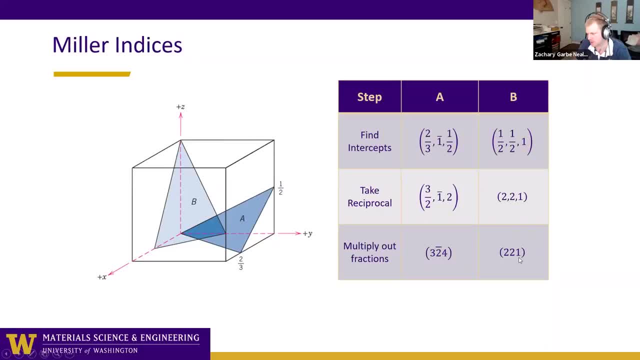 multiply them out and then the final notation is two, two, one for this plane. that's how we describe this plane. uh, for for a it's a bit more complex, because a intersects our origin, so we need to move our origin. we can't have it intersect the origin. we need to move the origin. 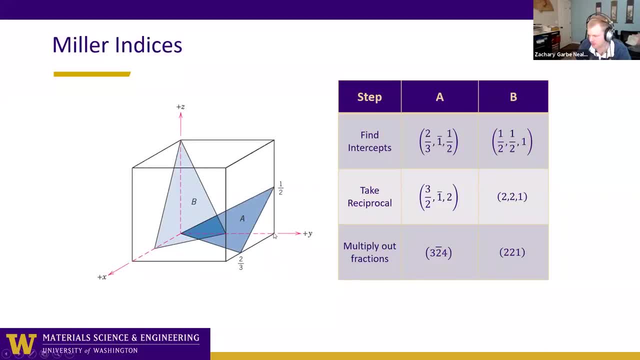 in order to calculate it. so if we move the origin to this position here, so we consider this zero, zero, zero. oh sorry, in the x axis intercepts at two-thirds, the y-axis- now we're going to negative intersects at one, and the z-axis intercepts at one half. uh, let me see there's a question. how do we? 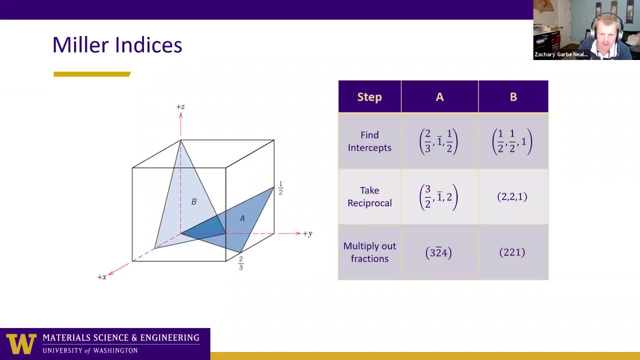 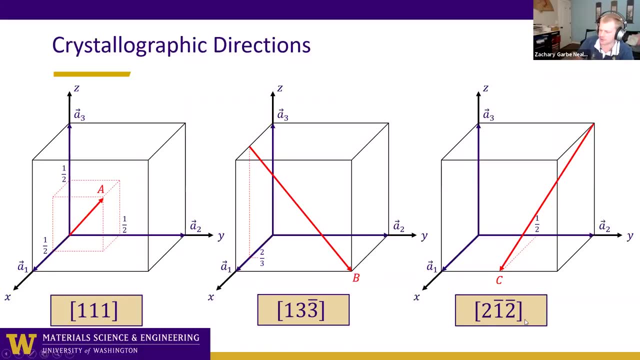 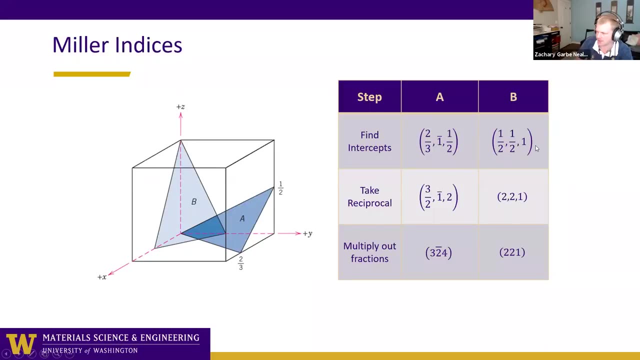 know when to write two, two, one, that we mean the plane and not the vector. oh yeah, so the vector is always going to be this is the square brackets. whenever you see a square bracket, you you know it's a vector, a direction, but when it's a plane, we use the, the parentheses. so that's how you know. 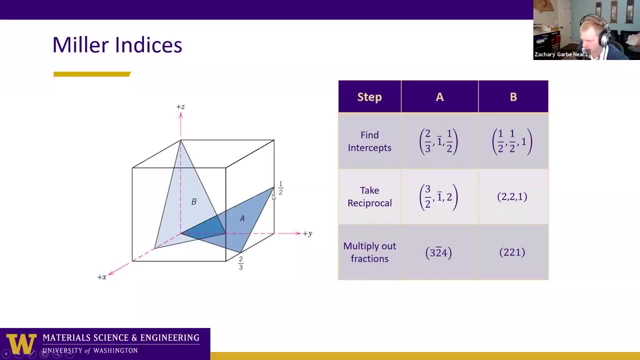 um, so moving, going back, let's see where was i. the the y direction is negative one and the z direction is one half. right, here is the, excuse me. the z intercept is one half. then take the reciprocal, so two-thirds becomes three halves negative. one is still negative one. one half becomes two, and then you. 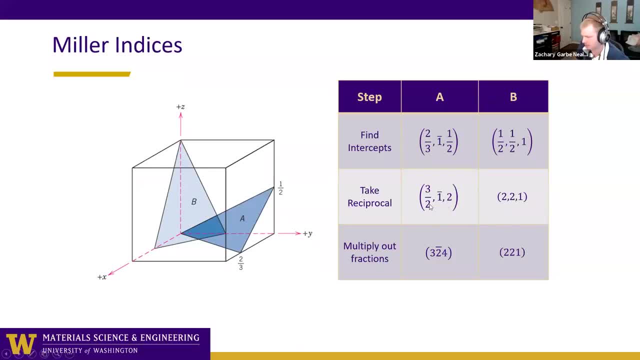 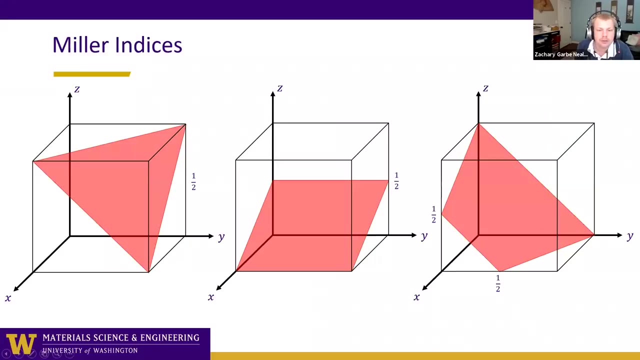 need to multiply out the refractions. so multiply everything out by two so this becomes three. two bar four. so that is the miller indice for this plane, a. okay, there's another question i missed. how do you know the right order of the numbers? um, are we talking? 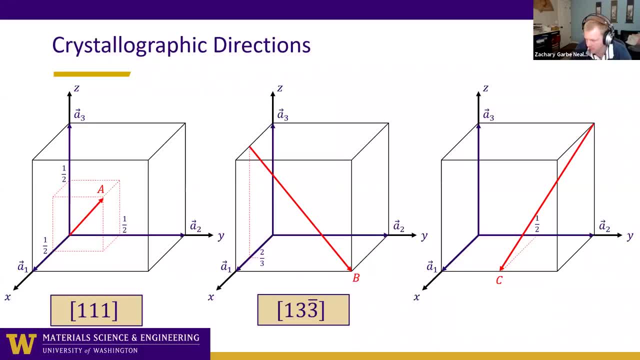 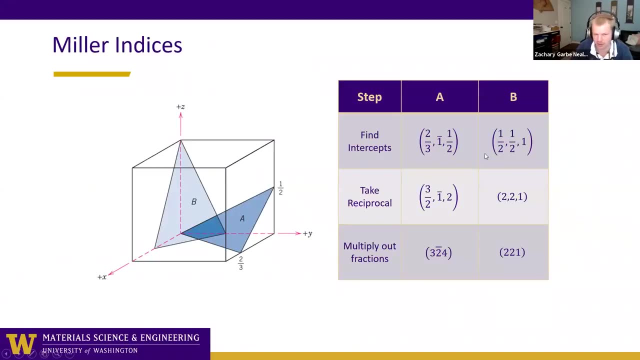 about daniel? this was your question. the right order of the numbers are we talking about the directions here? so it's it's always going to be like xyz for the planes. the right order- um, it's again the when we're talking about intercepts will be xyz is always in that order and, like i said, xyz. 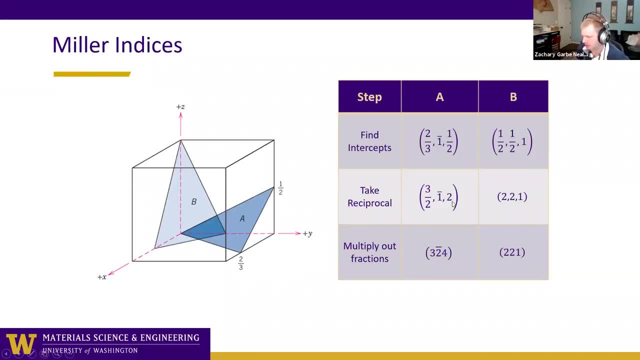 Negative one is still negative. one 1 1⁄2 becomes two, And then you need to multiply out the refractions. So multiply everything out by two, So this becomes three. two bar four. So that is the Miller Indice for this plane A. 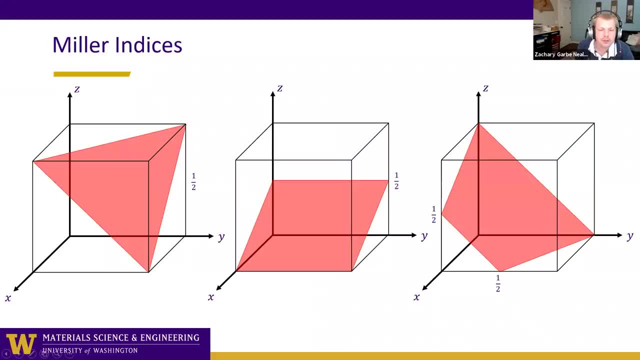 Now let's move on to the next measure. Let's move on to the next note. There's another question I missed. How do you know the right order of the numbers? Are we talking about, Daniel? this was your question: The right order of the numbers. 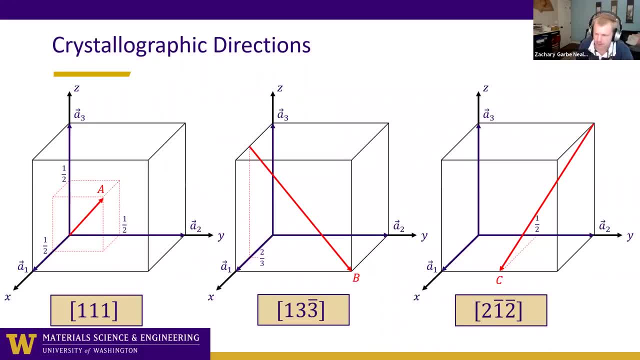 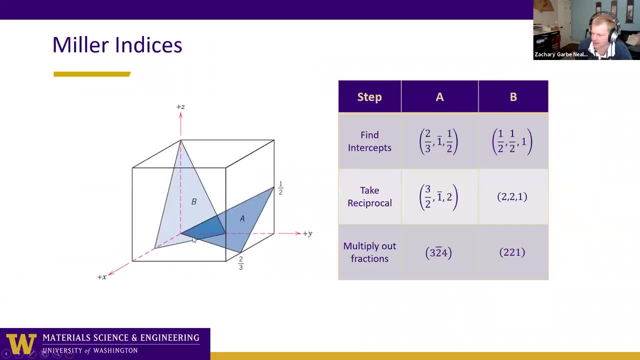 Are we talking about the directions here? So it's always gonna be like X, Y, Z. oh, for the planes, the right order It's again. when we're talking about intercepts it'll be X, Y, Z is always in that order. 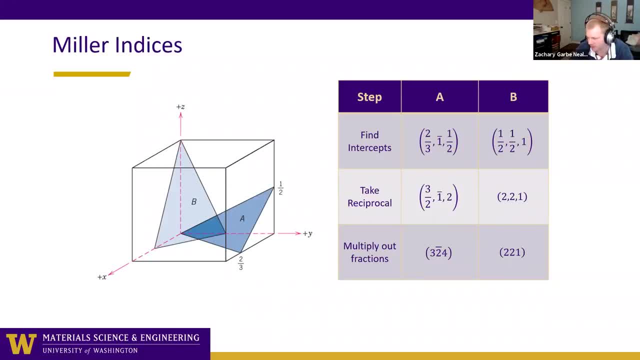 And, like I said, XYZ is a bit misleading, especially if we're changing into. this is supposed to be lattice space and not real space. But for cubic the lattice space is the same as real space. But if your unit cell is like trigonal or monoclinic, 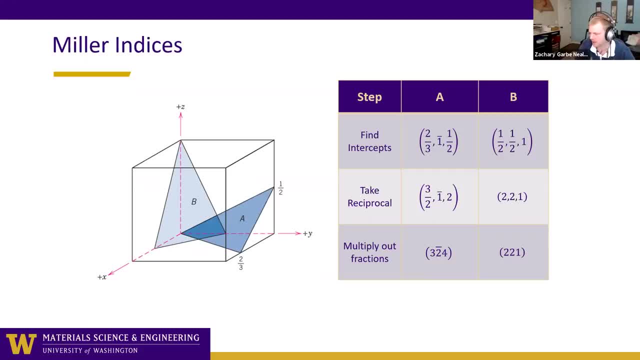 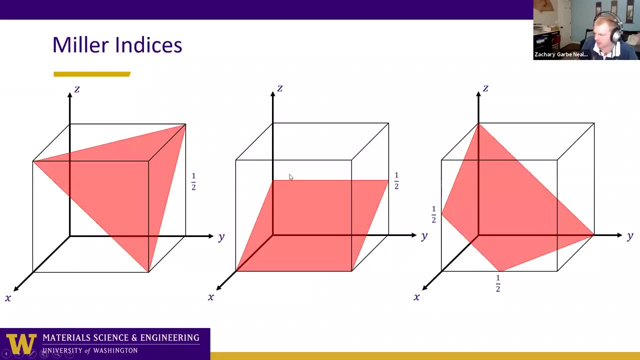 is going to have different angles, the procedure is all the same. So here's some problems that we'll go over. I think there was a typo here. This one half is by itself. It shouldn't be there, So we're going to find the Miller indices. 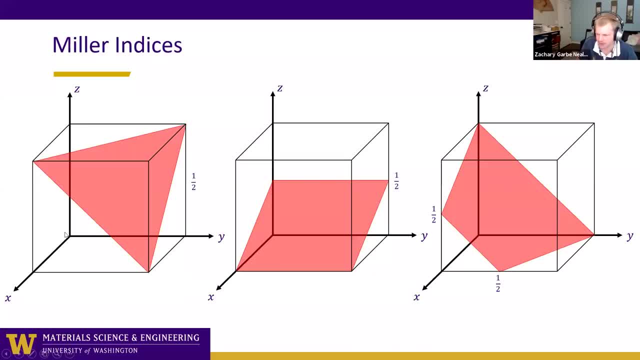 of these different planes of the cubic unit cell. So this one here is a bit different because we don't have it doesn't intersect right. In fact you could expand this plane and intersect way up here, But instead what we'll do is we'll move the origin. 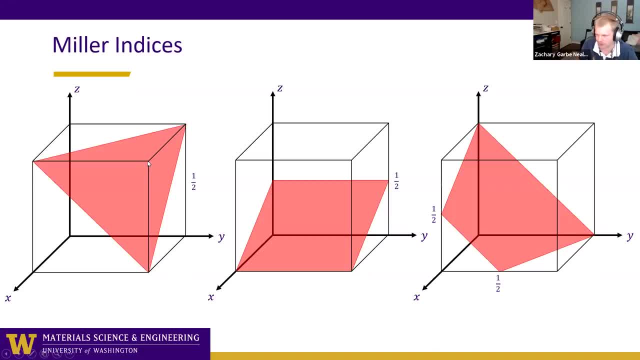 We're going to move the origin to this top corner here, And so in the X direction it's negative one, In the Y direction it's negative one, And the Z direction it's negative one. So this Miller indices of this is going to be one bar. 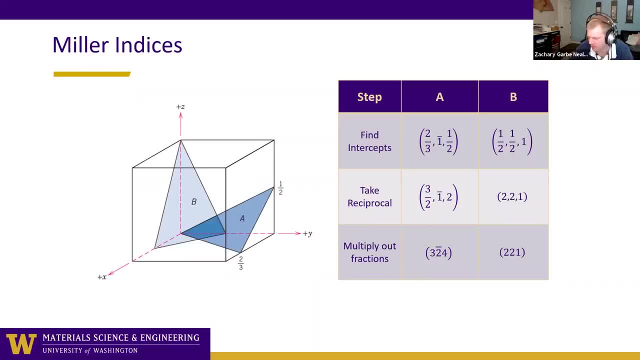 is a bit misleading, especially if we, if we're changing into: uh, this is supposed to be lattice space and not real space. but for cubic the lattice space is the same as real space. but if you're, if your unit cell, you know, is like trigonal or monoclinic, is going to 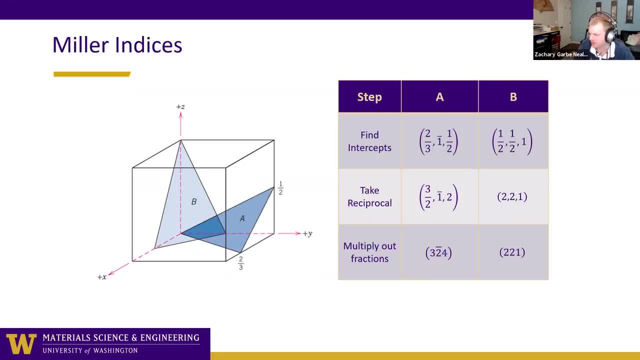 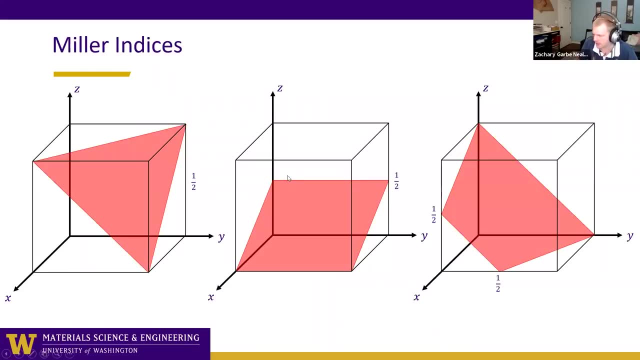 have different angles. the procedure is all the same. yeah, um, so here's some uh problems that we'll go over. i think there's a typo here. this one half is by itself. it shouldn't be there. uh, so this: we're going to find the miller indices of these different planes of the cubic unit cell. 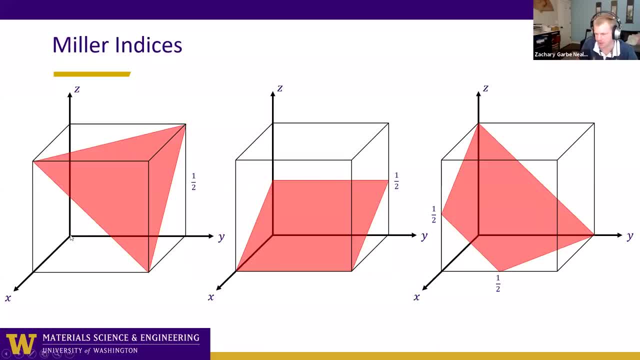 so this one here is a bit different because, uh, we don't have, uh, it doesn't intersect right. in fact, um, you could expand this plane and intersect way up here, but instead what we'll do is we'll move the origin. we're going to move the origin to this top corner here, and so in the x. 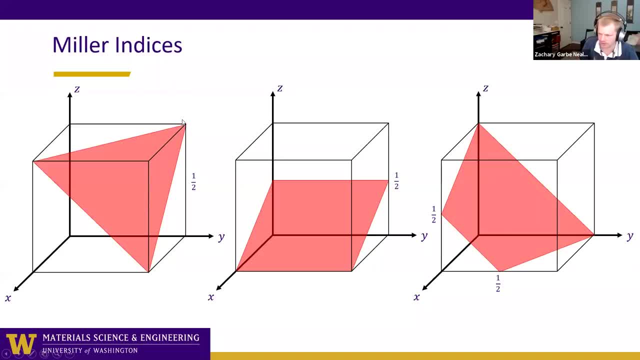 direction it's negative one, in the y direction is negative one and the z direction it's negative one. so this, this miller indices of this, is going to be one bar, one bar, one bar. let's see, yeah, that's right. okay, and this plane is equivalent to, uh, one one one. all right, one bar, one bar, one bar is equivalent. 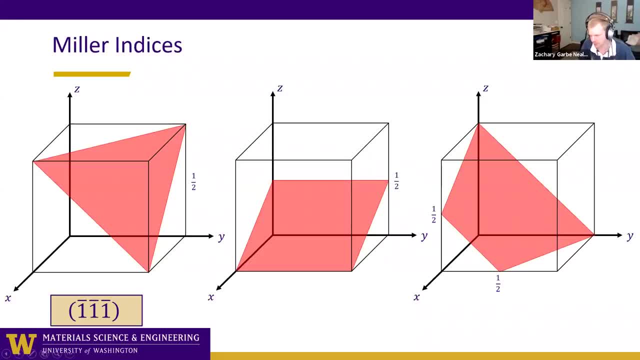 to one, one, one, uh. it's also equivalent to two, two, two and so on. all right, uh, but so one, this, you know. the correct answer would be one bar, one bar, one bar, uh, the next one, let's see. so this problem is a bit different than other ones, because the it never intersects the y-axis. 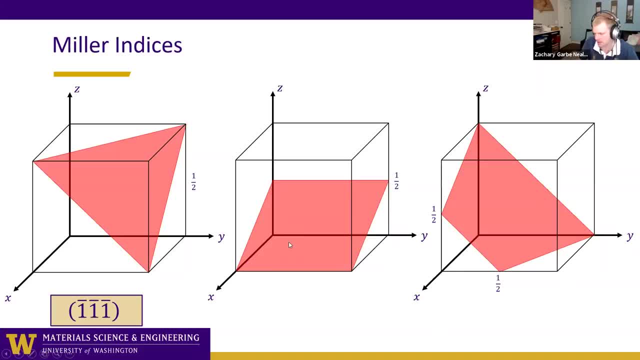 all right, this plane never intersects the y-axis, uh, so that in that case, for y will be zero. let's start with x, though x is going to be one y, zero, because it never intersects y. and then, uh, z is one half. so, remember, we need to take the reciprocal. so we start: one zero, one half, take the reciprocal. 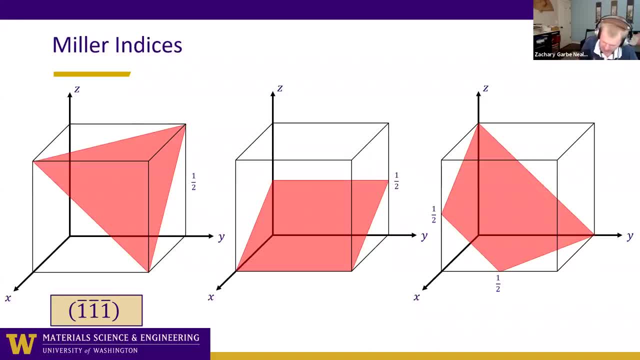 one bar, one bar. Let's see, Yeah, that's right, Okay, And this plane is equivalent to one one one. All right, One bar, one bar. one bar is equivalent to one one one. It's also equivalent to two, two, two and so on. 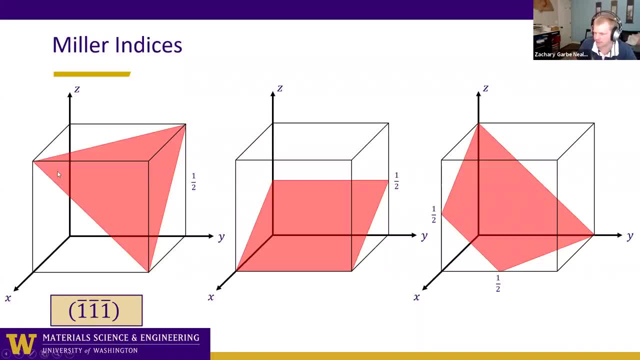 All right, But so one this. you know, the correct answer would be one bar, one bar, one bar. The next one, let's see. So this problem is a bit different than the other ones because it never intersects the Y axis. 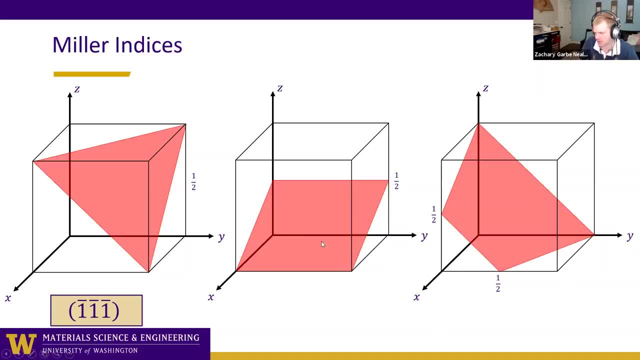 All right, This plane never intersects the Y axis, So that in that case, for Y it'll be zero. Let's start with X, though X is going to be one. Y is zero because it never intersects Y, And then Z is. 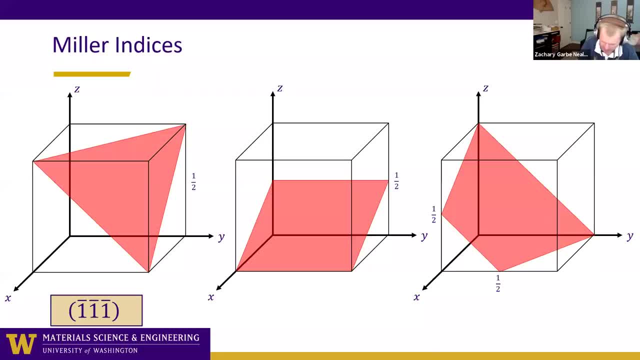 is one half. So remember we need to take the reciprocal. So we start one zero one half. Take the reciprocal is one zero two And then there's no fraction. So that should be the answer. One zero two is the Miller Indice for this plane. 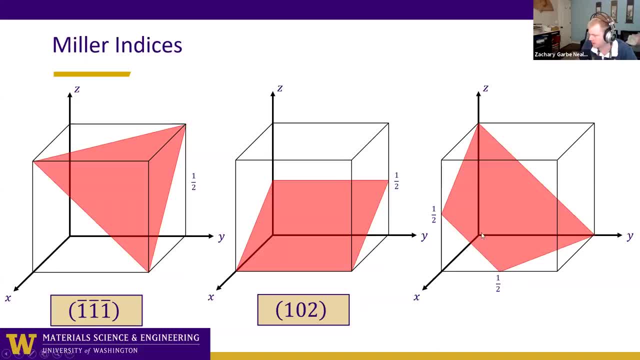 This next one is a bit more difficult because, again, the intersection with the X axis is not in the view of this unit cell, So you would have to extrapolate this plane down. So if this is one half here and this is one to one half, 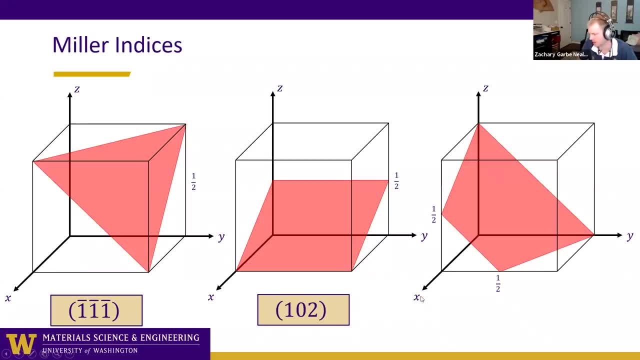 and then continue down, then it's going to end up intersecting X at two. So X is two, Y is one and Z is one, And this was starting at the origin. again, Okay, So it was two, one, one. 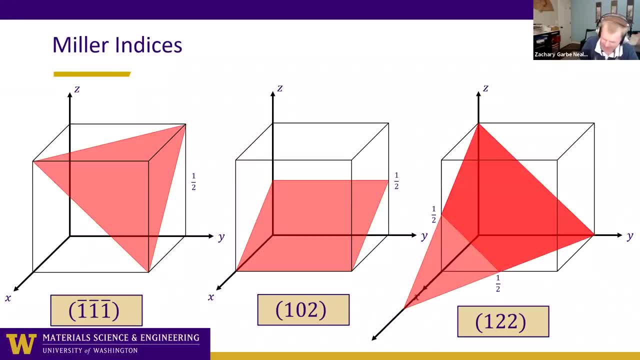 Oh, I got that wrong. What did I have? Oh, I forgot to take the reciprocal. Yeah, yeah, So it's two one, one before the reciprocal, But remember, we need to take the reciprocal, reciprocal, reciprocal. 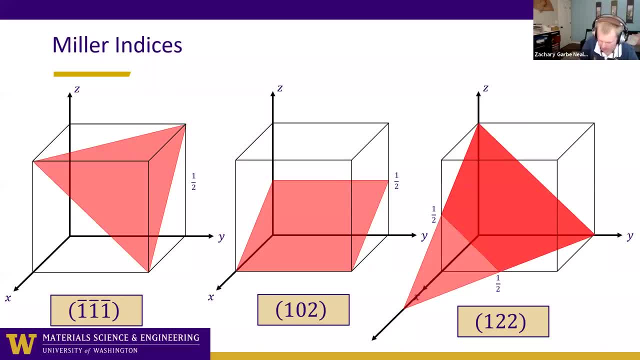 so two turns into one half. So then it's one half one one. then multiply out the fractions, it becomes two, one, one. excuse me, one, two, two. Okay, so I got that one wrong because I forgot to do the reciprocal. 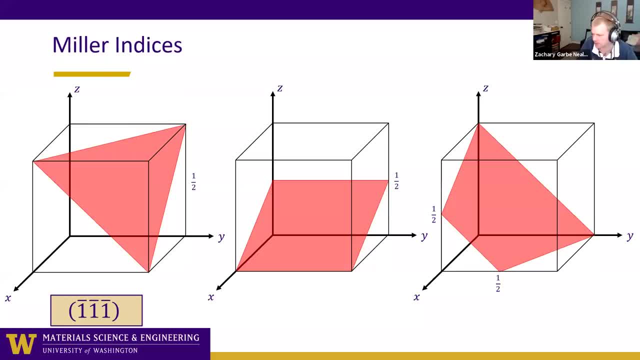 is one zero two, and then there's no fraction. so that should be the answer: one zero two is the miller indices for this plane. this next one is a bit more difficult because, again, the the intersection with the x-axis is not in the view of this unit cell. 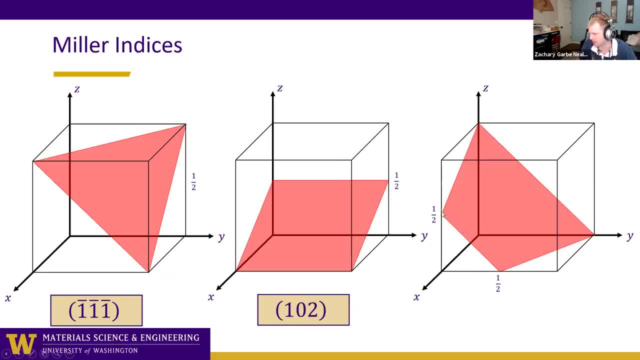 so you would have to extrapolate this plane down. so if this is one half here, if- and this is one to one half and then continue down, then it's going to end up intersecting x at uh z and then it's going to end up at two. so x is two, y is one and z is one, and this was starting at the origin. 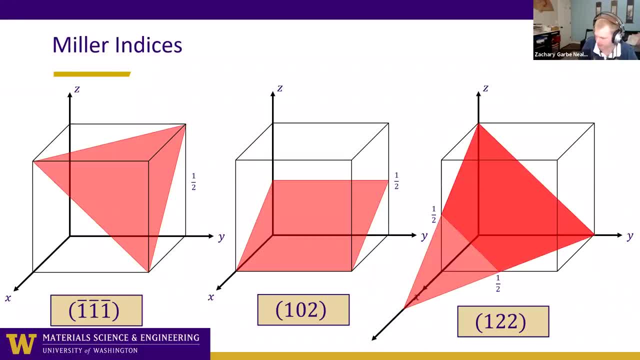 again. okay, so it's two, one, one. oh, i got that wrong. what did i happen? oh, i forgot to take the reciprocal. yeah, yeah, so it's two, one, one before the reciprocal. but remember, we need to take the reciprocal reciprocal. so two turns into one half. so then it's one half one. 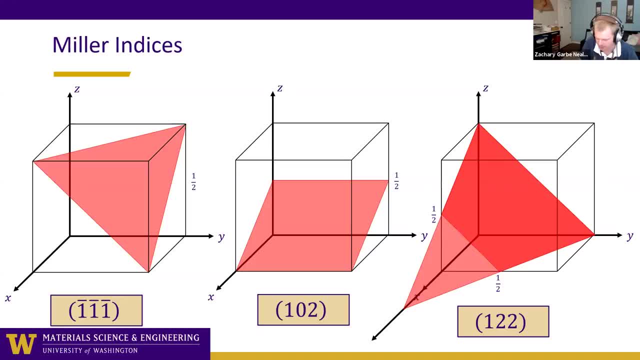 one, then multiply out the fractions, it becomes two, one, one, excuse me. one, two, two. okay, so i got that one wrong because i forgot to do the reciprocal. so always remember for planes you need to take the reciprocal before the final answer. okay, and then here's another question. 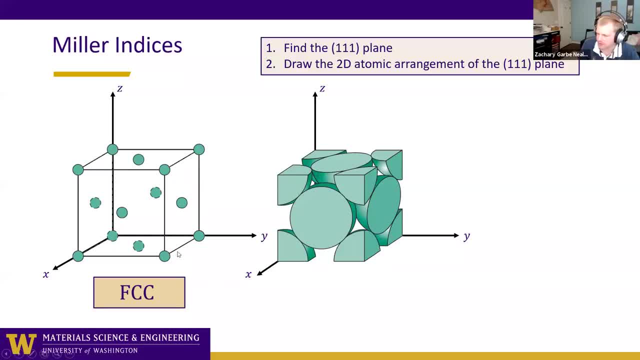 find the one, one, one plane of this unit cell, this fcc unit cell, and then also draw the 2d atomic array arrangement of that one one, one plane. now there's a question on your homework that's very similar to this and i i want to- uh, you know it's, it's the homework said. it was a hard, a difficult question. 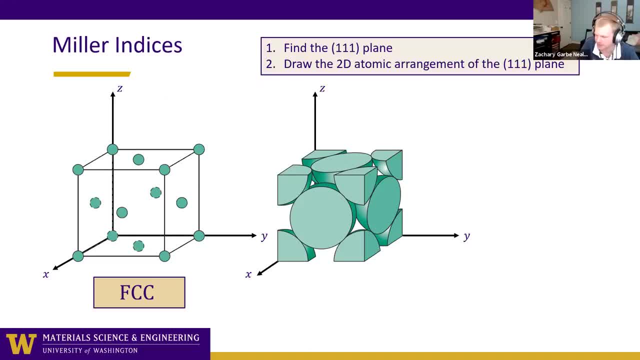 but it could be very easy if you know this trick, if you know this, i guess. uh, so one, one, one, of course. uh, the x intercept is one here, the y is one here and z is one here. so that makes this triangular plane okay. and then, if we were to do the reciprocal, we would have to take the reciprocal. 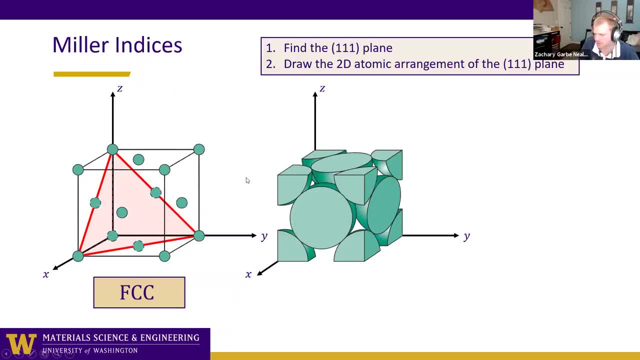 do right. when are we leaving at x1 right or y? once we're done here, one one is to 0, 1 and z is one, or meaning 1 at x1 right. so only one is needed. so that's themal plane from which we got the. 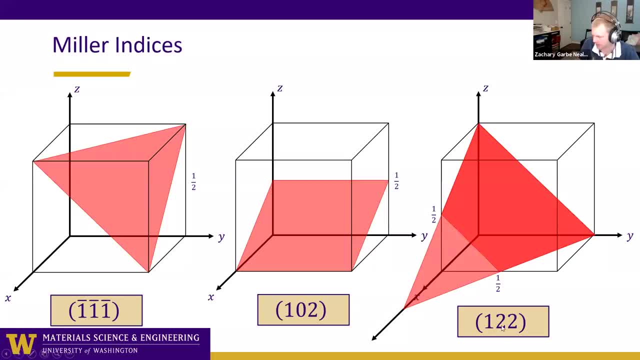 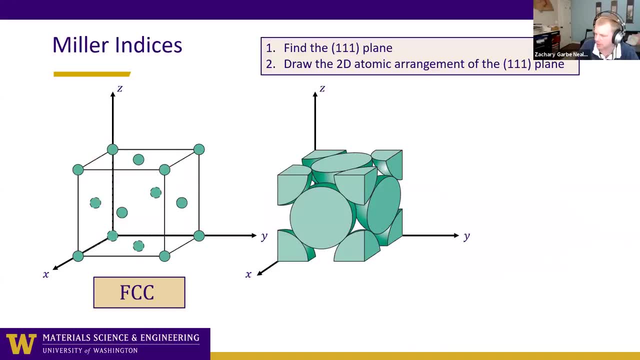 So always remember: for planes you need to take the reciprocal before the final answer. Okay, And then here's another question: Find the one, one, one, one plane of this unit cell, this FCC unit cell, and then also draw the 2D atomic arrangement. 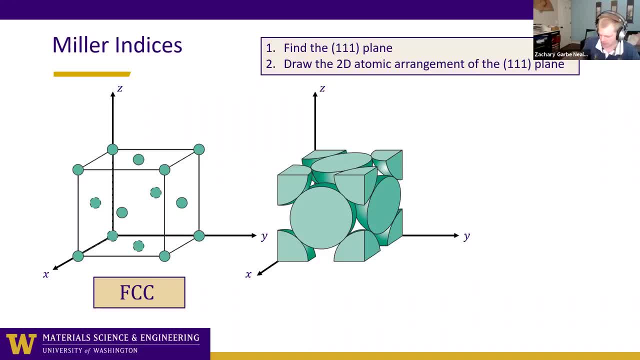 of that one, one, one plane. Now there's a question on your homework that's very similar to this And I want to you know it's. it's the homework said. it was a hard, a difficult question. 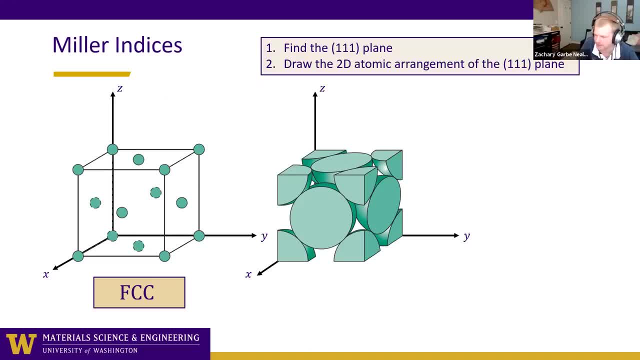 but it could be very easy if you know this trick, if you know this, I guess. So one one one, of course. the X intercept is one here, the Y is one here And Z is one here, So that makes this triangular plane. 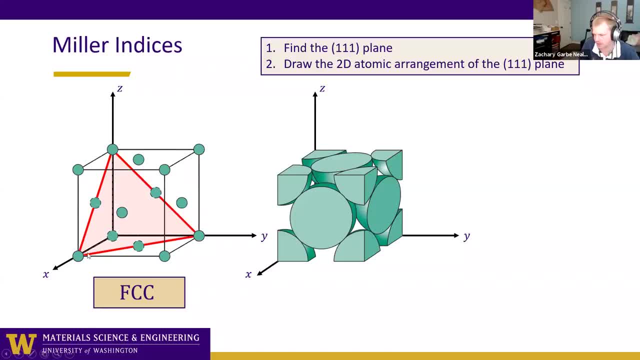 Okay, And then if we were looking at the atoms that intersect this plane? as you draw out those atoms, you know you get the closed-pack structure, the closed-pack plane. So for FCC unit cells, one, one, one is the closed-packed plane of atoms. 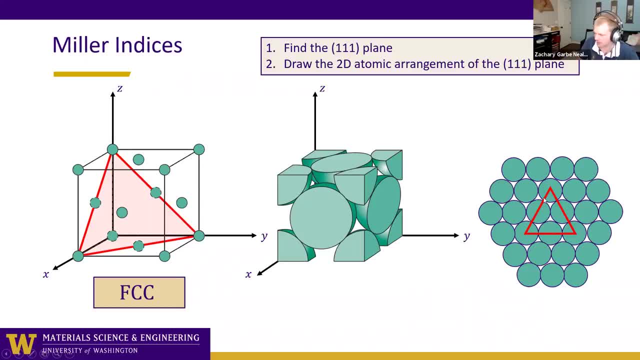 Whenever you see this hexagonal symmetry, right, this hexagonal symmetry of the atoms like this, this closed-packed plane, you should know right away that it's either, it's either the one zero zero plane of HCP. one zero zero. 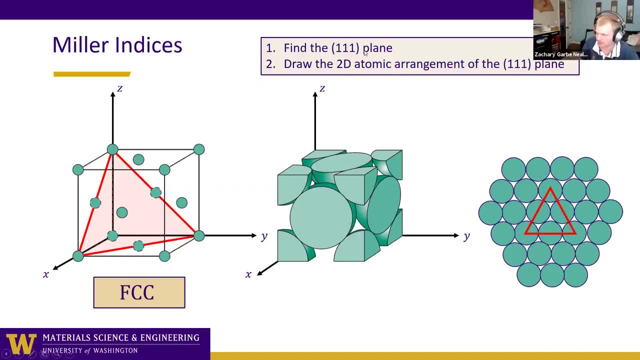 of HCP or a one one, one plane of FCC. All right, So there's a question on your homework that might seem at first a bit difficult, because it wants you like to calculate something in order to find it. It gives you, like an image of this. 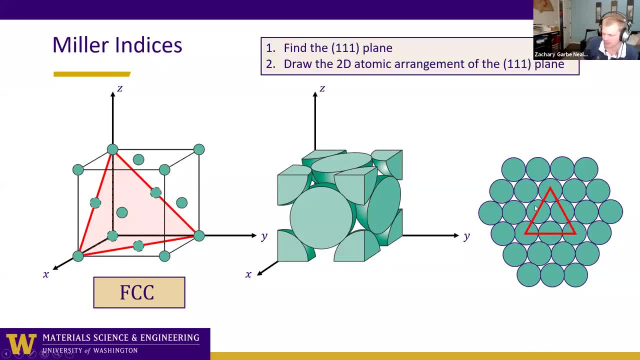 And you should know right away when you see this: oh, that's the one, one, one plane of FCC. Okay, So this is the one, one, zero, zero plane of HCP. But the question made it obvious is FCC. 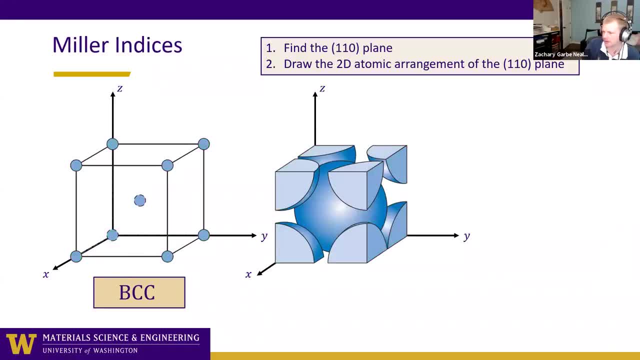 Okay, The same thing for BCC: Find the one one zero plane and then draw the atomic arrangement of that. So this one, one, one zero. the intercept on the X-axis one here and the intercept on the Y-axis is one here. 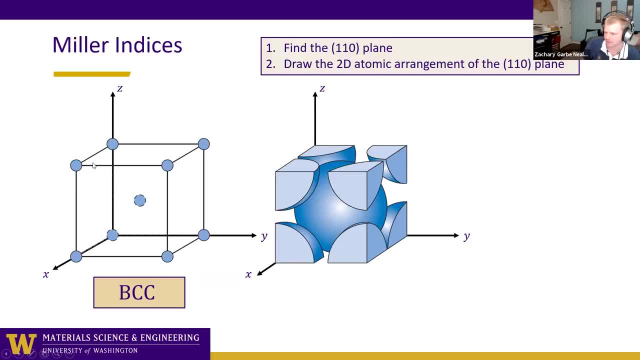 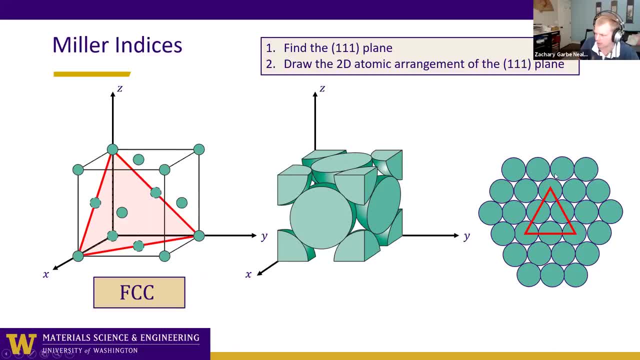 部分 alpha x1. I only need to take that is that. what i'm trying to get is help me imagine what this is for some. masse is a body. this is a physical body. this is the electronic body of aboat, which is designed to sample CO급. when we see the other two dunkом metal earth Anhang. 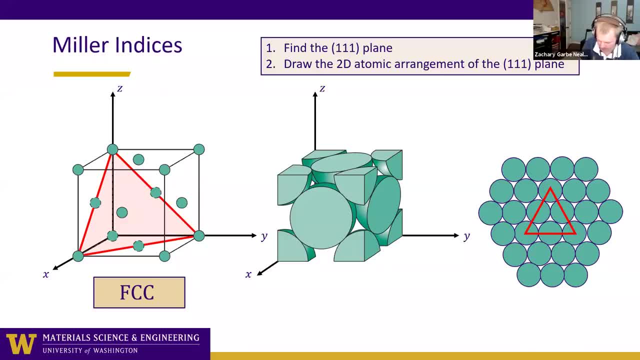 either the 1 0, 0 plane of HCP, 1 0 0 of HCP or a 1 1 1 plane of FCC. all right, so there's a question on your homework that might seem at first a bit difficult, because it wants you like to calculate. 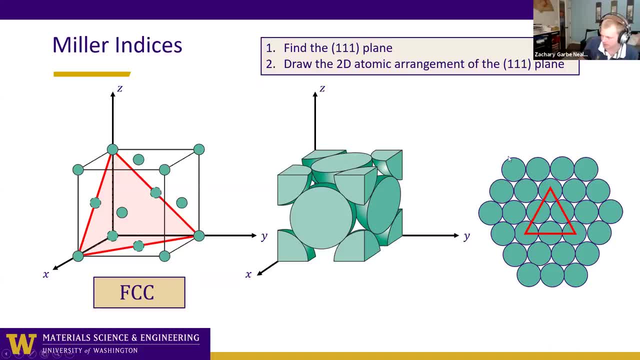 something in order to find it. it gives you, like an image of this and you should know right away when you see this. oh, that's the 1 1, 1 plane of FCC or the 1 0, 0 plane of HCP. but the question: 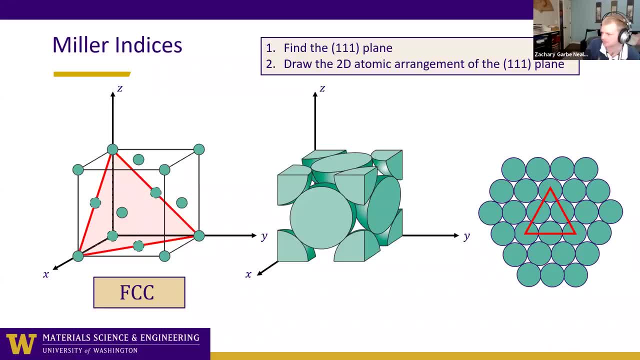 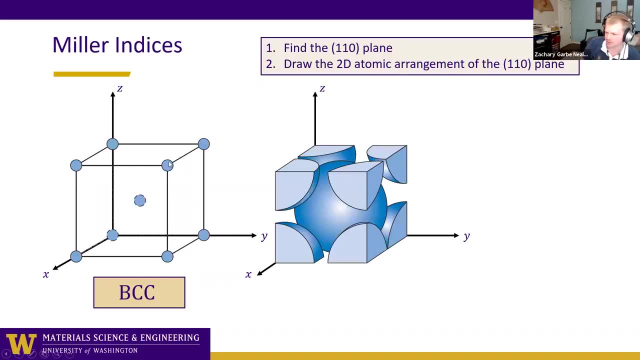 made it obvious is FCC. okay, the same thing for BCC. find the 1 1, 0 plane and then draw the atomic arrangement of that. so this one: 1 1 0, intercept on the x-axis- 1 here, and then intercept on the. 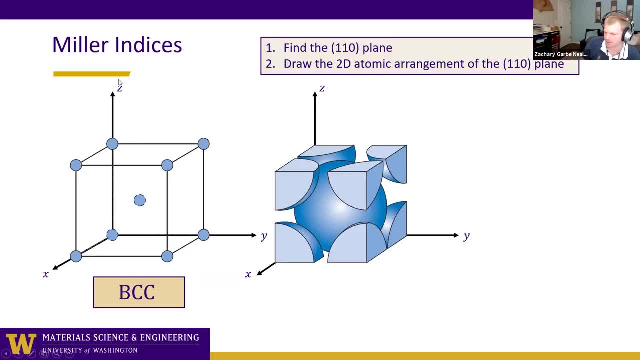 y-axis is 1 here and there's no intersect on the 0, on Z, so this is going to be a slice along the diagonal here. okay is the 1, 1, 0 plane, and if we were to draw out the atoms on this plane, this is what it looks like. 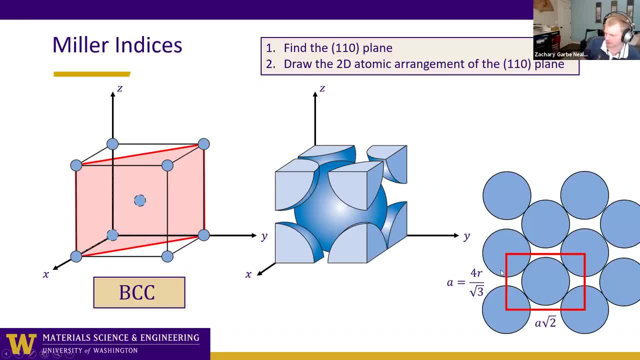 and remember we talked previously what the unit cell last parameters were, and so this is the atomic arrangement of the 1: 1: 0 plane for BCC. so if you had a iron, for example, iron is a BCC metal. if you had a single crystal of iron, for example, 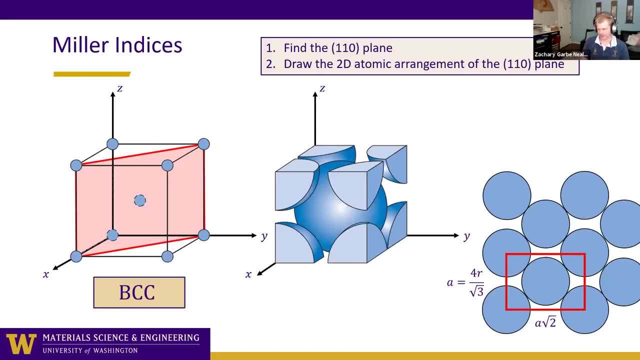 if you had a single crystal of iron and it was cut along this 1 1, 0 plane so that the surface of the single crystal one was 1: 1, 0 at the surface, the atoms would be arranged in this pattern. all right, so that's what that means there. okay, I think. next I'm going to talk about x-ray diffraction.